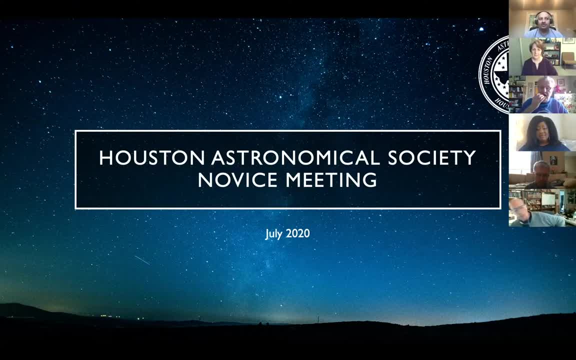 is a chat feature in the Zoom client where you can go ahead and post any questions you might have. I'll go ahead and keep track of those as we go through the presentation and then we can ask those at the end of Tom's talk as well. For those of you who are watching through our Facebook page during: 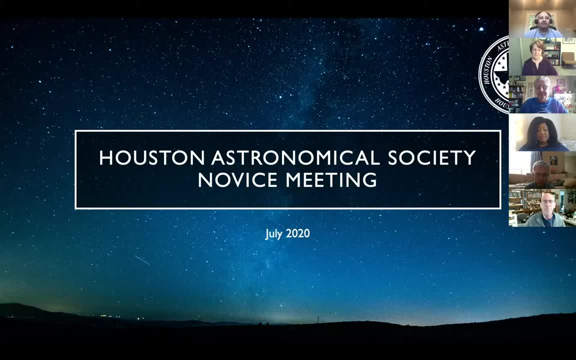 the live stream. go ahead and ask your questions there in the Facebook page as well, and we'll get to those at the end of the talk additionally. So I've done all the talking I want to do and I can't wait to hear Tom's presentation tonight. So I'll pass it over to Debbie Moran for her announcements. 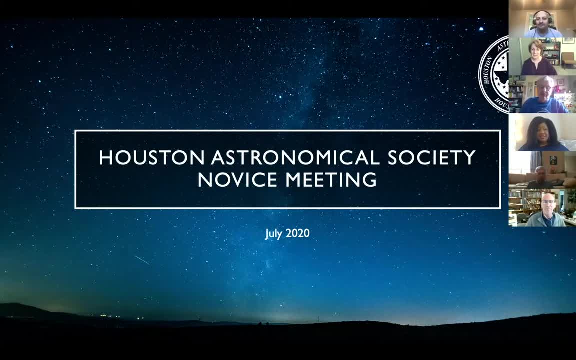 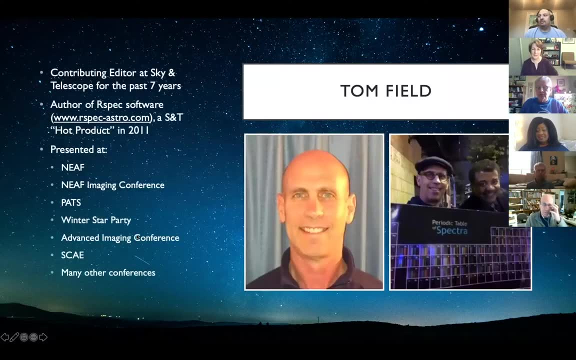 and to let her introduce our guest speaker. Hi everybody, I'm Debbie Moran, I'm the novice chair And we have two types of talks in this novice group. One's really for beginners And I just want to let everybody know. if you really need, 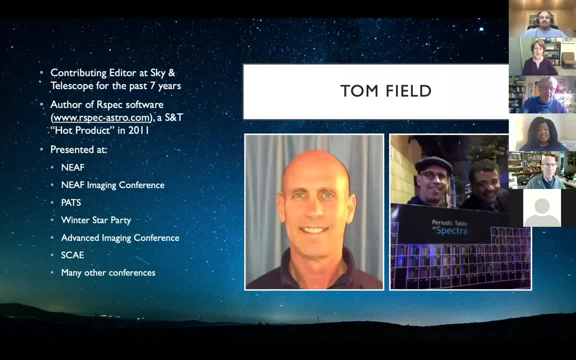 to know the basics of telescopes or sky navigation or what's up in the spring or the summer. we have a lot of recorded talks, anytime you need them, at our Houston Astronomical Society website And you can find that under recorded presentations We also do talks like tonight, Tom. feel free to. 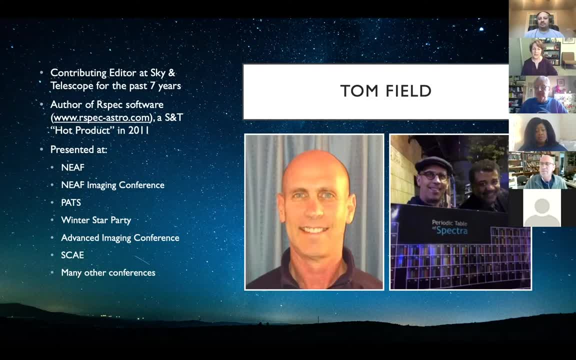 jump right in. Hi, I'm Debbie Moran. I'm a graduate student at Houston Astronomical Society. I'm here today for the first time as a graduate student at Houston Astronomical Society And we have a talk with our graduate student, Dr John Bogdanovich, who's going to talk about spectroscopy, And we're going to 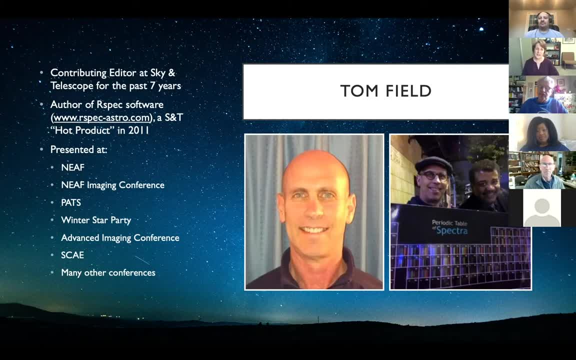 talk about how to do spectroscopy through your telescope. So this may be a new pursuit even for a more experienced astronomers. And I was especially excited when he wrote to say he has this talk, because I remember when I took astronomy at the University of Texas one of my favorite projects was 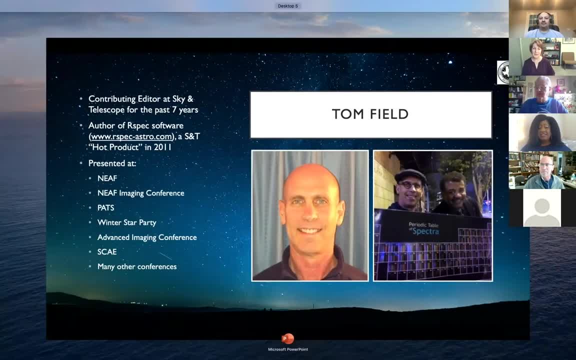 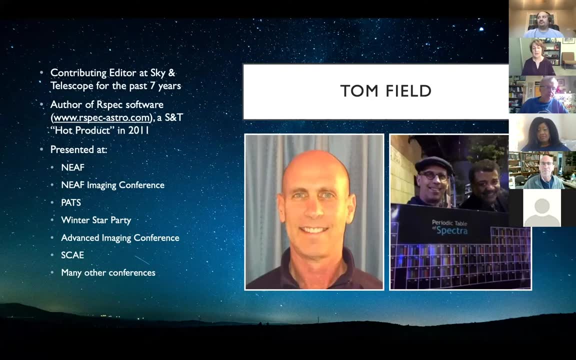 making a rudimentary spectroscope, light sources in the laboratory and lights in the sun and on my ceiling, and it was just a wonderful experience. I also learned very much about all the information you can pull out of the spectrum far beyond this composition of a star. so we'll hear all about that tonight from Tom. he is a contributing. 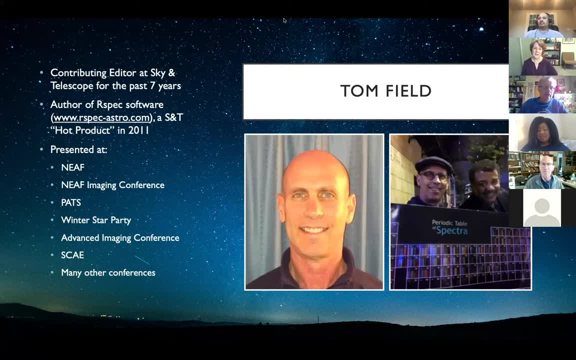 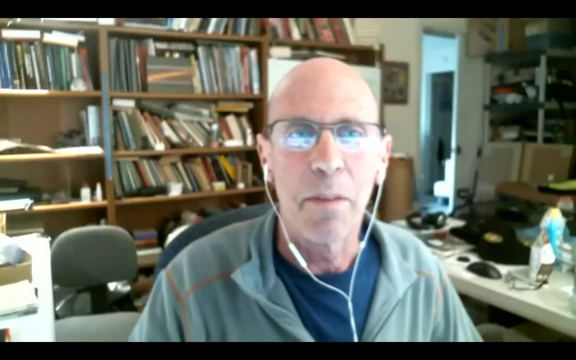 editor at Sky and Telescope magazine for the past seven years and the author of the R-SPEC software, and he is based in Seattle Washington right now, and so we're very pleased to have Tom field. thank you very much. thank you, and I appreciate this club really has it going on. I'm a little intimidated. there's just 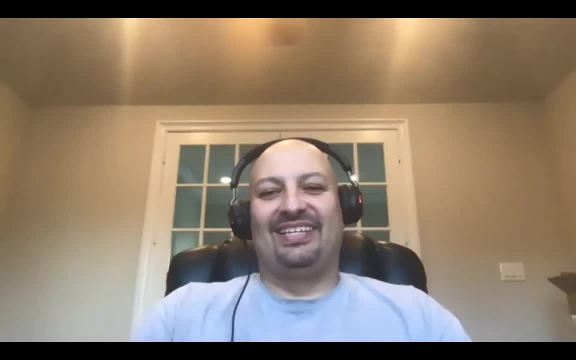 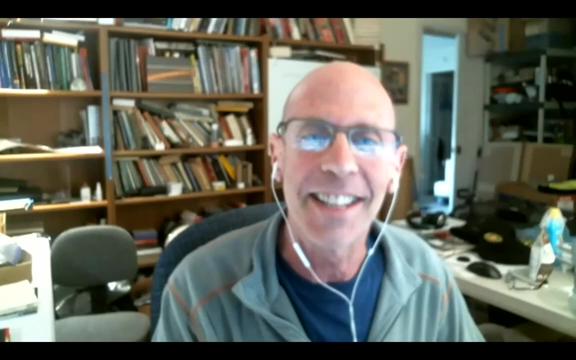 this real professionalism, like go get them, this is a Texas thing or what's going on here. they don't pay us either, right, so great, listen now. thanks everybody for coming tonight. I appreciate the introduction and the opportunity to talk. I'm gonna share my screen here and then. 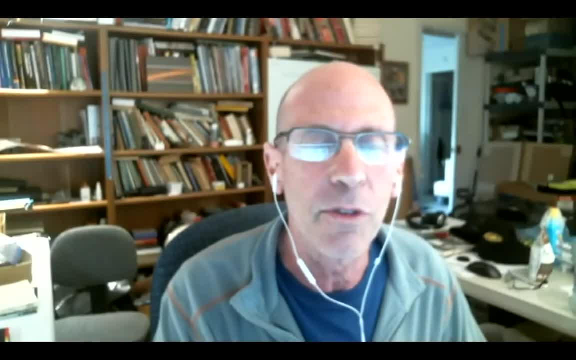 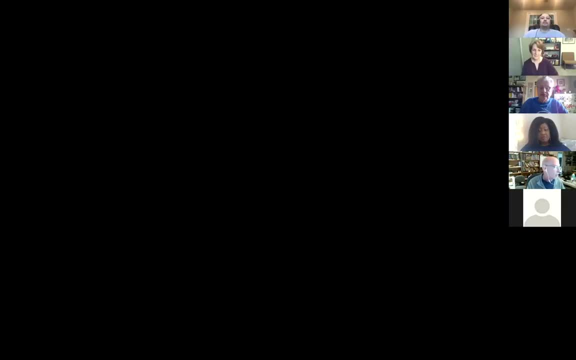 uh, bring up another slide deck for us to take a look at. I'm actually on a different monitor than it was when I started the other monitor. I had just been having some trouble and I thought that, geez, all I need is to screen share and have that monitor cause problems, so you all can see that prism now, there I 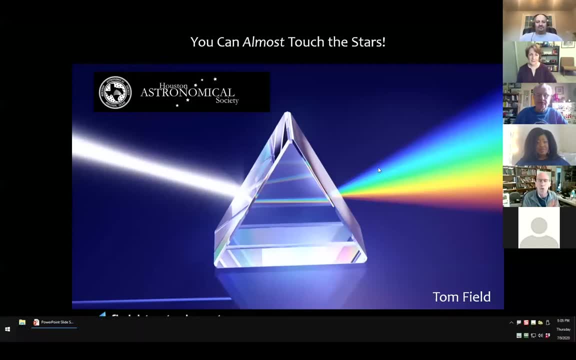 suppose. so I'm gonna talk for 40 to 50 minutes. I've got a lot of ground to cover. I'm gonna talk a little science, a little history, and then get into the meat, which is the kinds of things that we all can do with spectra. 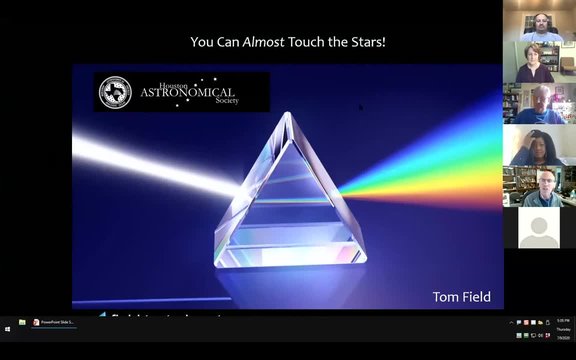 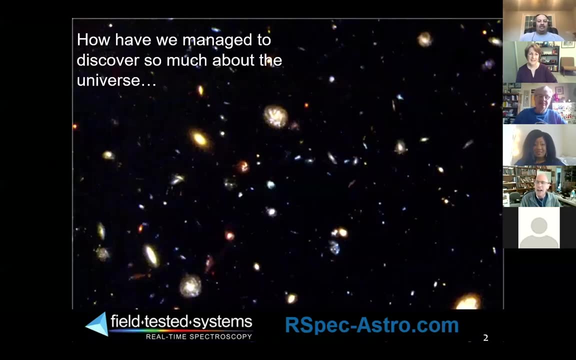 so let's get started. let me get things just a little more set up here. I love your logo, by the way. well, thank you. I can't tell you when it was designed, but yeah, it's, it's kind of stood the test of time. thank you, absolutely. so how? 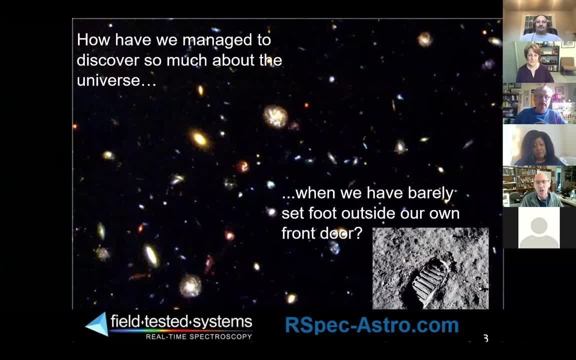 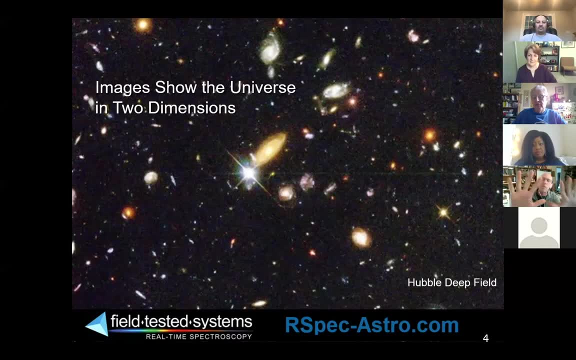 isn't? we've managed to discover so much about the universe when we've barely set foot outside our own front door. you know, we can get images like this one. this is the Hubble Deep Field And, by the way, this is a piece of the sky that's the size of 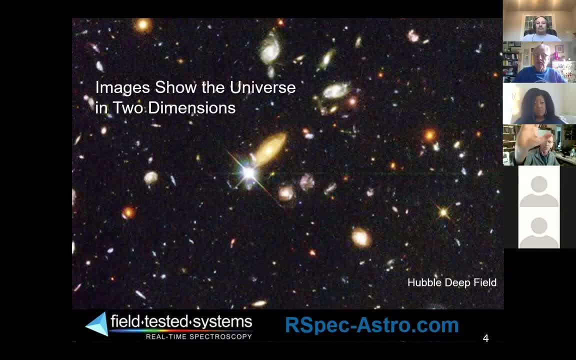 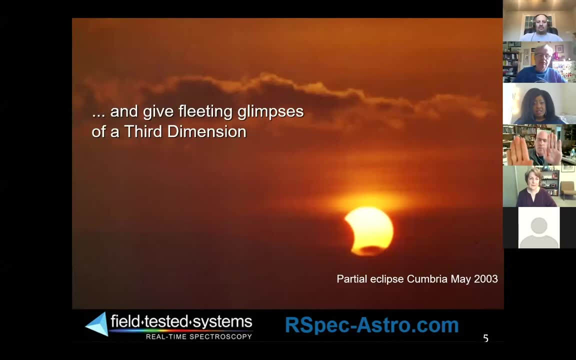 a tennis ball held at arm's length. It's really busy up there if you look deep enough, So we can get two-dimensional images, of course, And if we wait a little bit and are in the right place, looking in the right spot, we can see a little bit of a third dimension. We can see some depth. 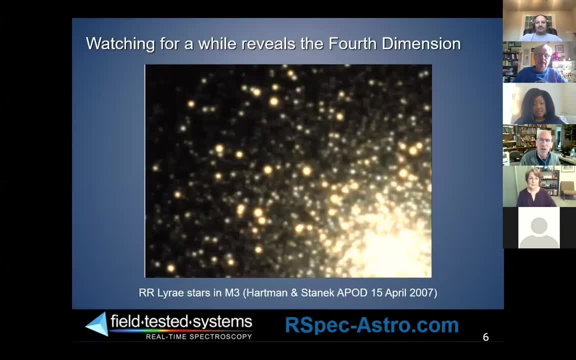 from eclipses And if we watch for a while we can see a fourth dimension time And I think maybe you can see up there in the right-hand corner and in other places. I'm actually going back and forth between two slides, So if the period isn't exactly regular, it's not that we've made some. 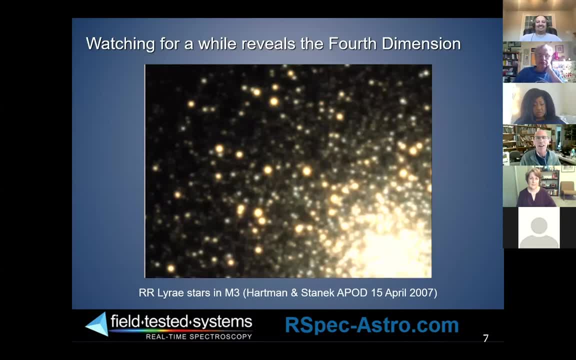 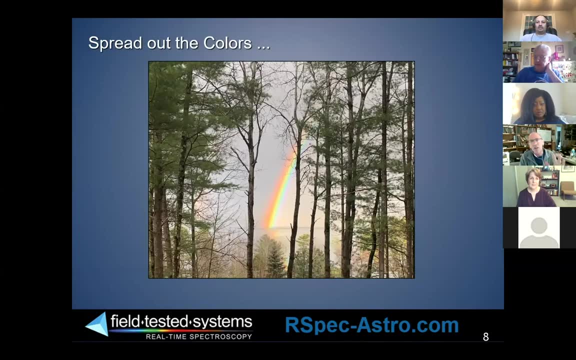 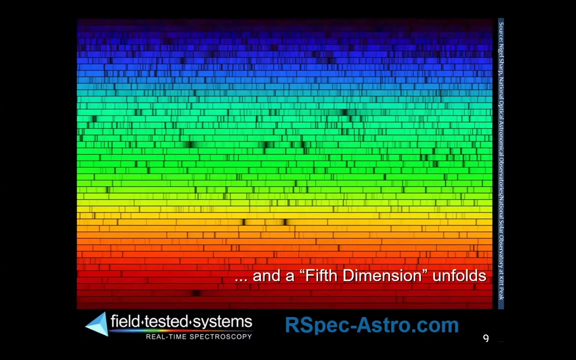 magnificent discovery about irregular variables. These are our Lyrae stars, which are one of the standard candles. Now, if we spread the colors out, we get an as-if fifth dimension. I love the colors of this. They're the real colors. They're not human-made colors. These are nature's colors. 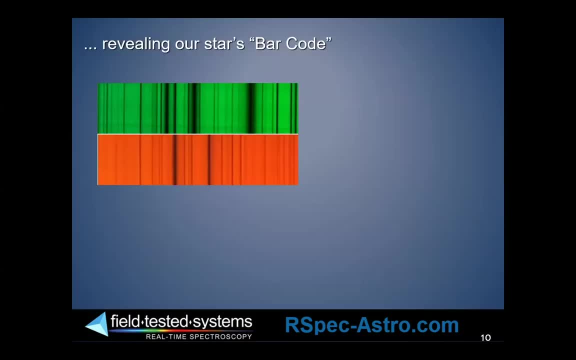 And this fifth dimension reveals the barcodes as-if of stars And we can use those to understand stars. Now, about 80% or so of the research that gets done astronomically uses spectra. Now, whether it's 50% or 70% or 80%, it doesn't matter, It's a huge number. So, even if you're not an 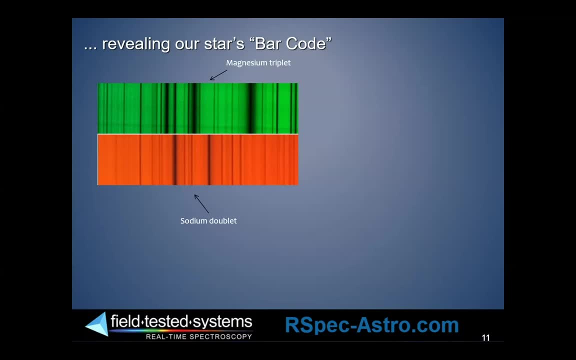 imager, it's helpful if you understand why it works and how it can be done, And so if you're an armchair astronomer and you don't go out and observe, you'll still pick up things in this talk that you enjoy. But the kinds of things that these barcodes reveal include knowing what 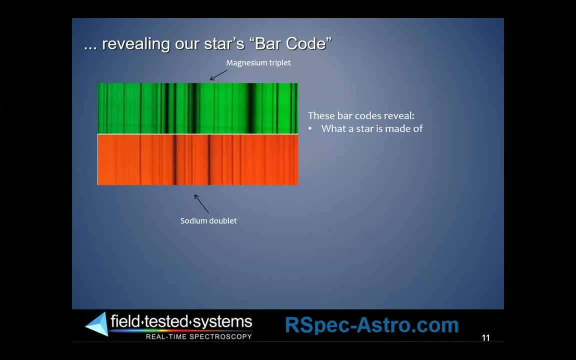 a star's made of, what its composition is, what its radial velocity is, if it's moving towards and away from us, and also if a star's spinning- And I'll give you some examples of all these tonight- And it's, of course, its temperature and where it is in its life cycle on the HR diagram. 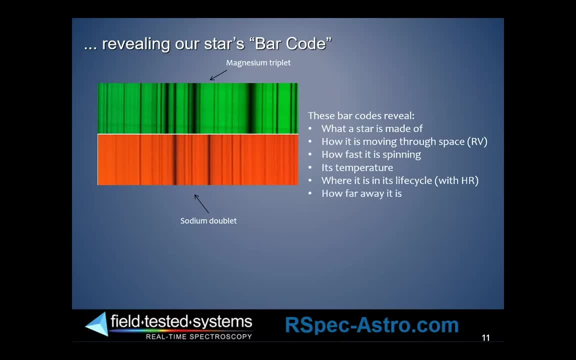 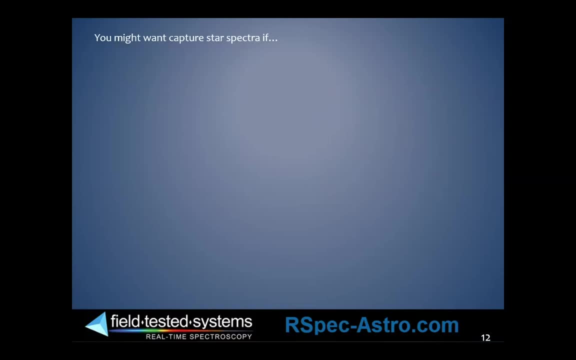 And also distances. We can measure those, And I'll show you some distance measurements that were measurements also used by well, a Nobel Prize winner, as we'll see. So, as I've given this talk over the years, I realized that in the back of my mind I had certain items that I wanted to cover. 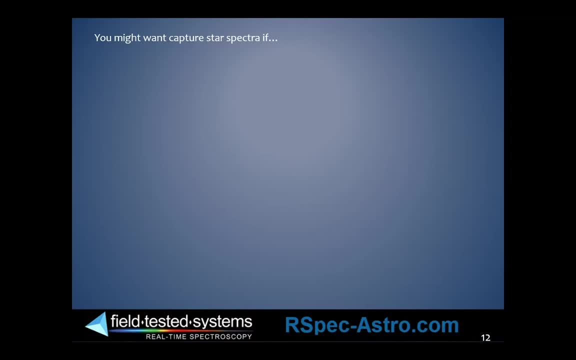 And I thought maybe I'd just lay them out here So you might want to capture spectra, if you remember the thrill of that first image you took of the moon. Now, if yours was like most of ours, it was blurry, it was overexposed, but it was the most beautiful image you had ever. 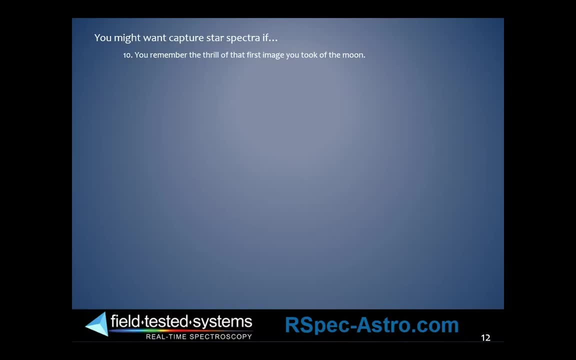 captured or seen right, You were showing it to your spouse or your friends, your colleagues. So that same thrill is a thrill that when I got started in spectroscopy about 10 years ago I realized I could recapture again And it was exciting for me that I think the brain is a 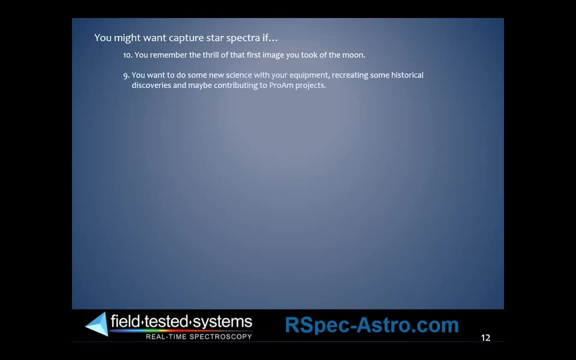 novelty engine, you know. So it was very exciting. Maybe you want to do some new science with your equipment, Maybe recreating some discoveries of different spectra, or contribute to some professional amateur projects. You might want to capture spectra. By the way, this is more words on one. 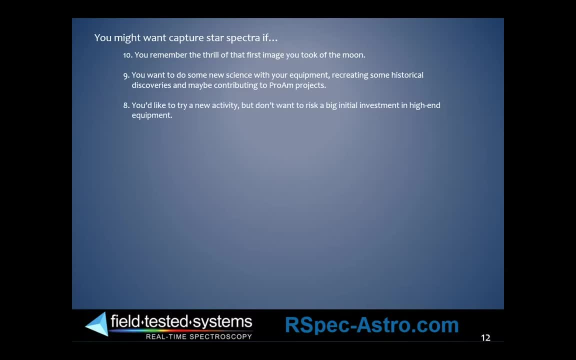 screen than you'll see for the rest of the talk. This is really bad PowerPoint to do all these words And I'm trying not to read them. So for me, somebody online in the last day I was reading they were saying: well, I wanted to buy a telescope, but I have to get it past my credit. 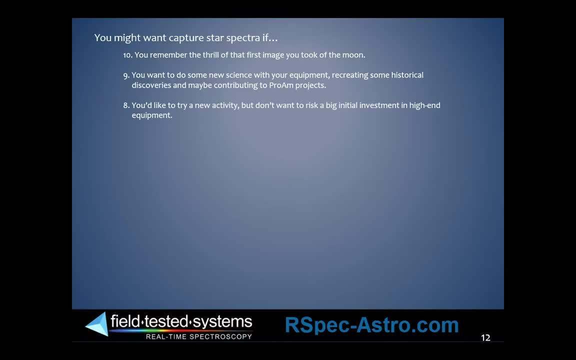 card scrutineer. Now, I'd never heard of a credit card scrutineer. I'd never heard of a credit card scrutineer before. But again, we all, many of us, have scrutineers in our lives when we're looking. 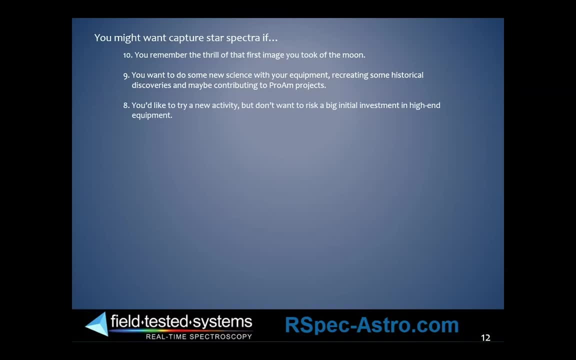 to make hobby purchases, And often we're our own- and well we should be. So what you'll see tonight is an example of the kind of thing you can do without a huge investment. The other thing I discovered is that when you actually own the data, when it's your own, you have more of an emotional 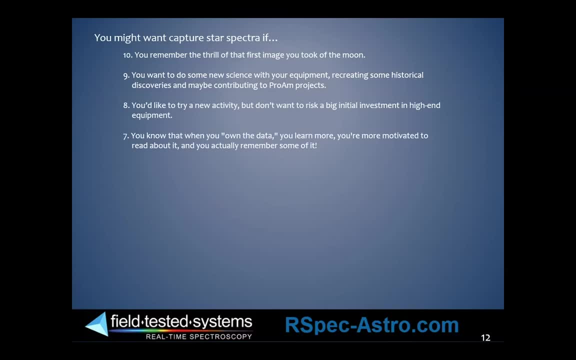 relationship to it in a good way. It's a good relationship And you tend to want to understand more about it And things actually start to change And I think that's a really good thing, Instead of going in one ear and going out the other that they do with me. 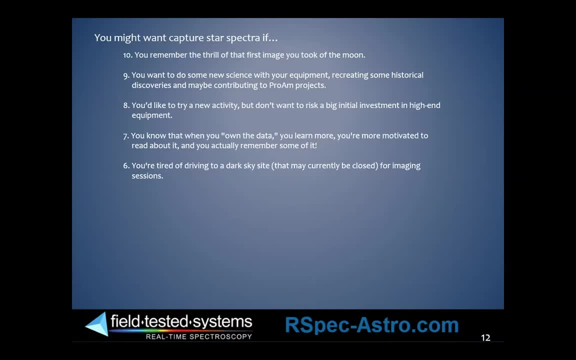 Also, I don't know, maybe your dark sky sites down there are closed right now And what you're going to see is that spectroscopy is much more immune to urban light pollution. One of the reasons is we're not really being a slave to the human eye and the aesthetics, With science looking at. 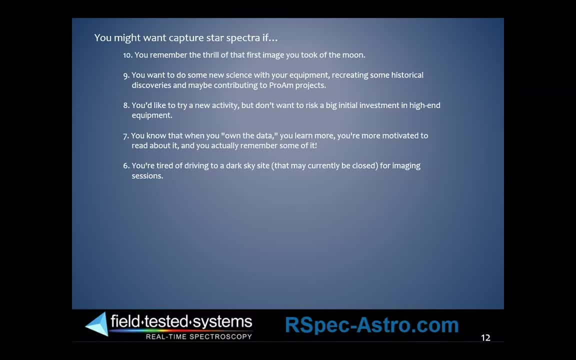 spectrum peaks and dips. we want the data pretty much the way it hit our telescope, So there's not a lot of fine tuning For me. I had done some imaging, like many of you have, I suppose, And I had one of these books. maybe you're familiar with it. It's a large format book. 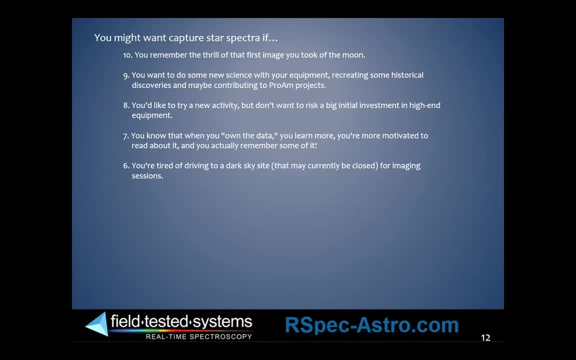 eight and a half by 11.. Let's see if I've got it over here. I don't seem to have it And it had these examples, right page, left page, before processing some great convolution process and after, And I'd look at those and I'd go I guess, yeah, I guess I see a difference, But 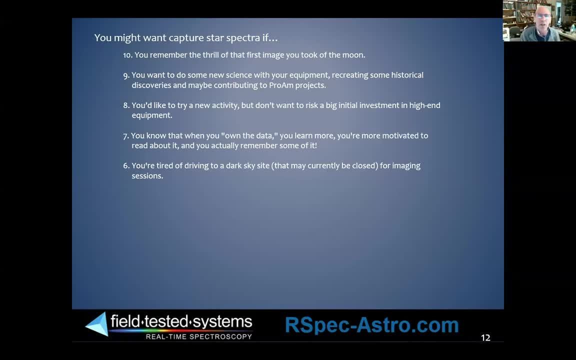 it wasn't something that excited me. On the other hand, I'm the beneficiary of those features when I see those beautiful images that some other people capture. And you might want to do spectroscopy if you want to do a little science with your telescope, but you don't have a PhD. 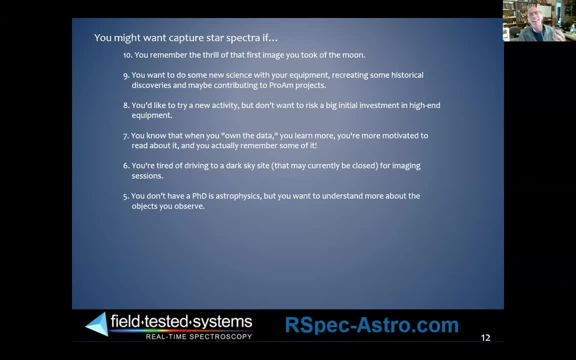 I don't. I'm a knuckle-dragging programmer And the nice thing is you don't need to know a lot of science and there's lots of ways to learn what you need to know. And for me, I don't have the 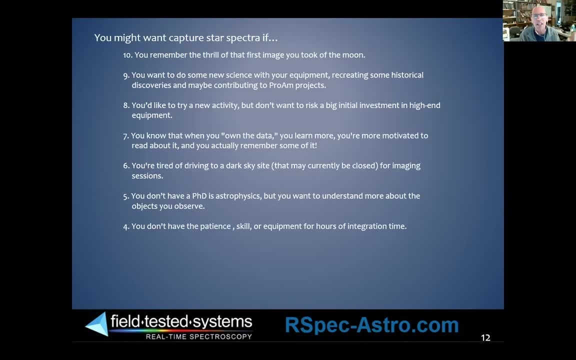 patient skill equipment, dark sky site, any of that stuff that I would need to do hours of integration time And I'm going to show you some images. And I'm going to show you some images tonight, made real time with video, And I think you'll. 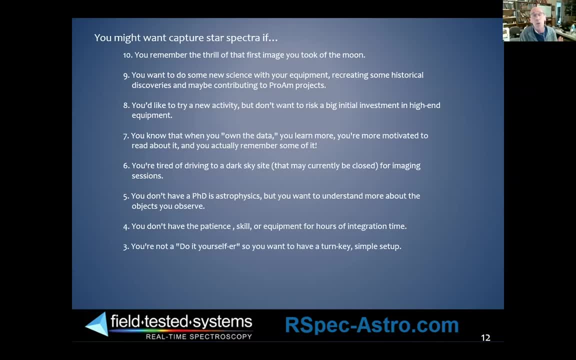 see it's remarkable what can be done, And I also break just about everything that I touch in hardware. For me, my favorite keys on my computer are edit, undo or control Z. Wouldn't it be nice if we had an edit undo in life, sometimes Just saying, But what I'm going to show you tonight, 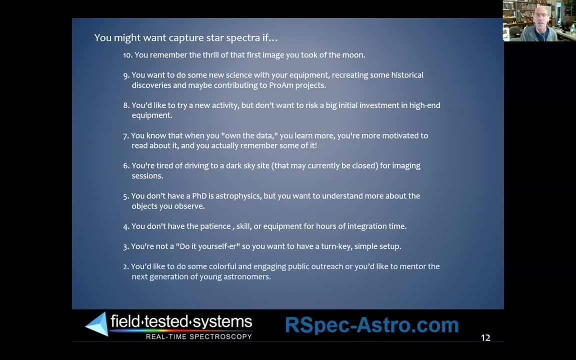 also, although there's plenty of do-it-yourself projects, you're going to see things that are easy to set up And, if you like, doing outreach, you're going to see things that are easy to set up And, if you like doing outreach, you like mentoring. this is a great topic, So keep all. 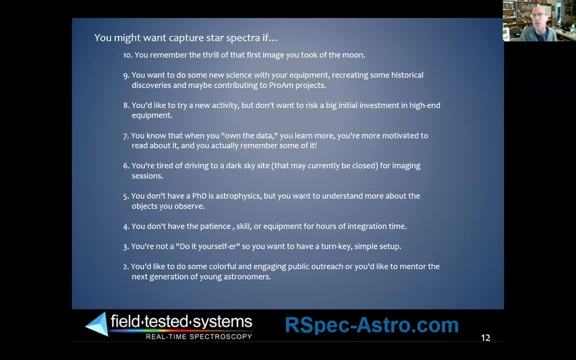 these in mind And the number one reason. number one, only because it's the last of them. you want to hang out with a cool crowd. Now, I'm not one of them, but there's a huge community of people doing this, a lot of online communities, And if it's been some time since you learned something, 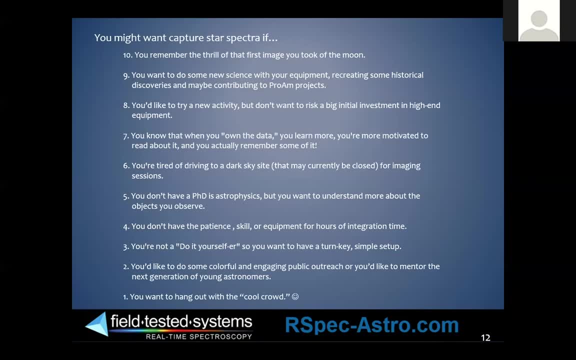 new. I can see some of you here, I can see, have been around in astronomy for a while, right? So when you last learned something new, it might have been a long time ago, It might have been decades ago, And that even with a good club like the Houston Club. 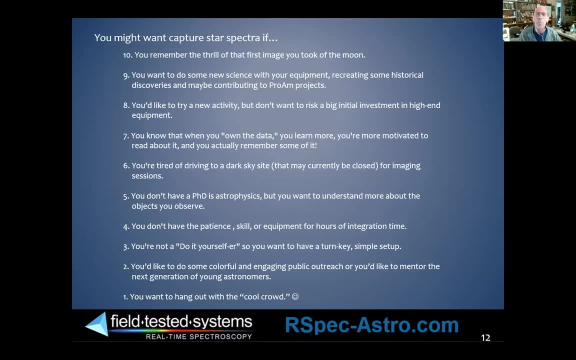 I know flattery won't get me anywhere. with this group you're tough, But even with a club it can be hard to learn all the things you need to know. Of course, these days with the web, it's all easy, Okay, so I'm going to do a little bit of history here. I'm going to jump around in. 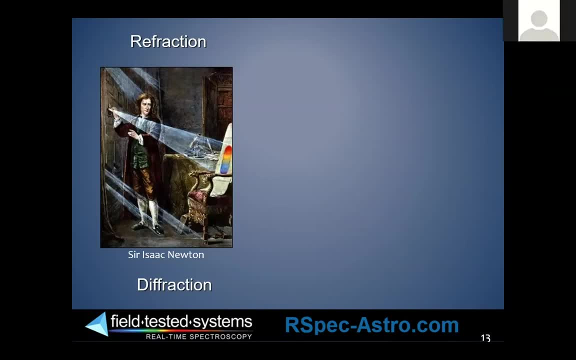 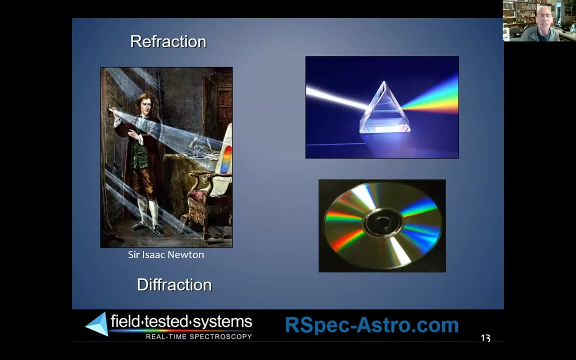 time. a little bit And then a little bit of the science. Most of us know that Sir Isaac Newton split light using a prism and discovered that it was made up of all the colors. And you can also split light by bouncing it off of a finely lined surface, like a DVD. 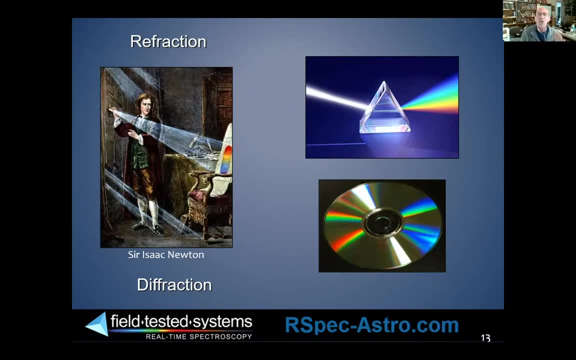 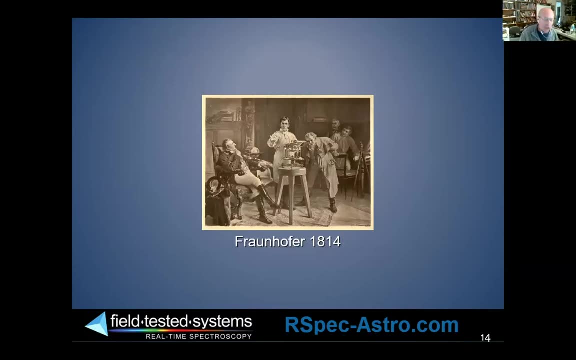 or even passing it through a finely lined, semi-transparent surface piece of glass. it's got etched lines on it. So back in 1814, this crew here, including Fraunhofer, here they're looking through a spectroscope at the spectrum of the sun, Fraunhofer. 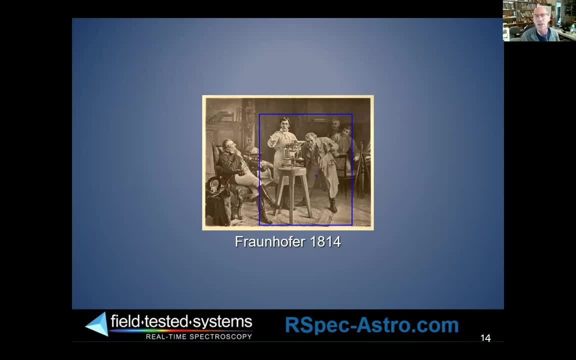 discovered the spectra of the sun and that star spectra differed from one another. They didn't know what they were looking at, but it was something of interest and led to the discoveries we're about to discuss. But before we look at those discoveries, I want to rewind about 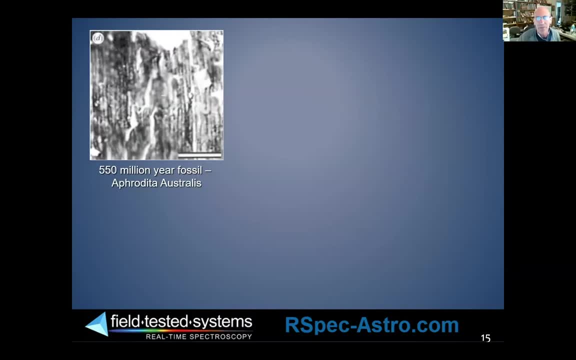 a half a billion years ago. Now some of you are going wait a second. I didn't sign up for whatever. this is paleontology So. but look at that surface of that fossil. You see all those striations. Well, this guy, Professor Parker, saw that and he said: you know, that sort of looks like the? 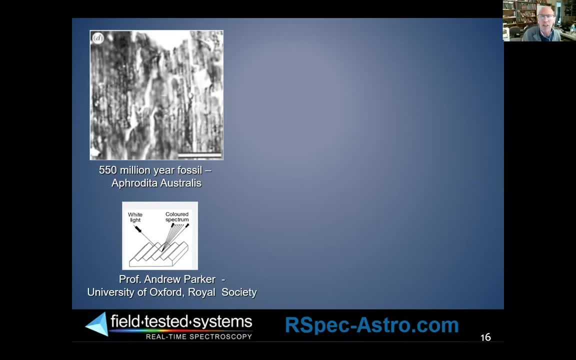 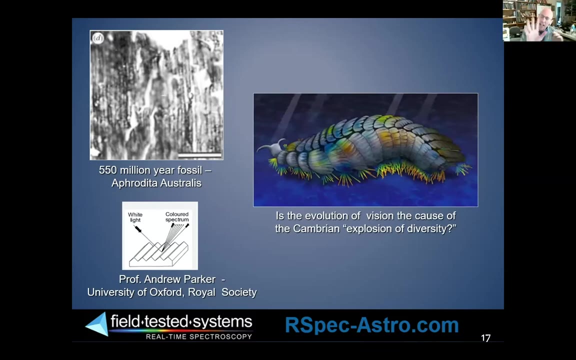 finely lined surface that would produce multiple colors like a reflecting DVD. And so he said: what would an animal look like and why would have that occurred in the history of evolution? So he said that's sort of what maybe it could have looked like, And in this era, half a billion. 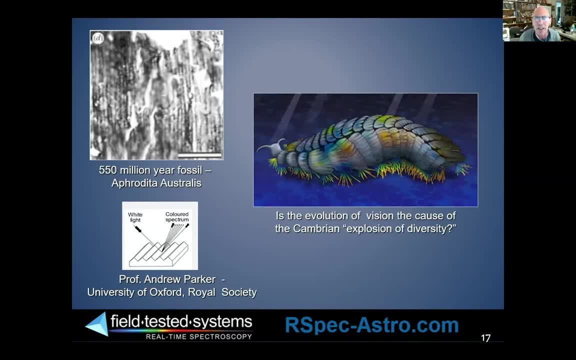 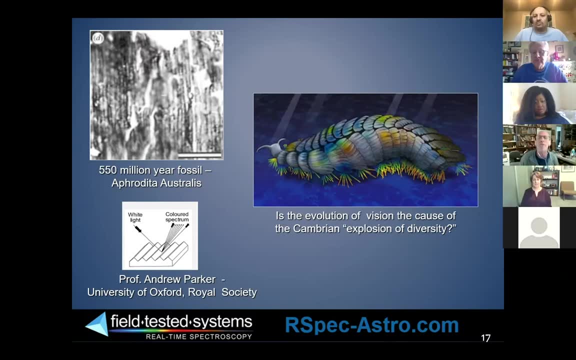 years ago there was a huge explosion in diversity. And so he said: you know, it doesn't make any sense to have all these diverse colors unless they're eyes. So maybe the two co-evolved together. Okay, let's get back onto the science, our science track. Talk just real briefly about things many of 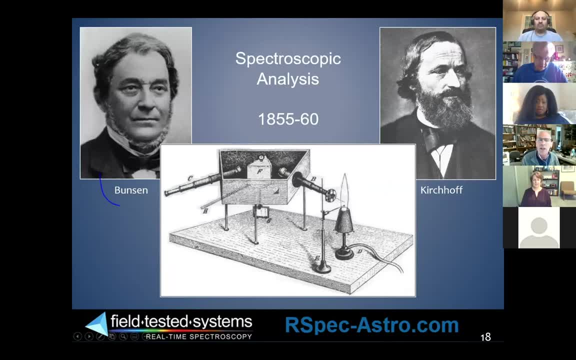 you are familiar with and can probably explain equally or better. Bunsen, of course, invented the Bunsen burner. Now the Bunsen burner which we have here. he invented to burn samples here, go through a spectrum with the light and look at the result. And he was a pyromaniac: He burned. 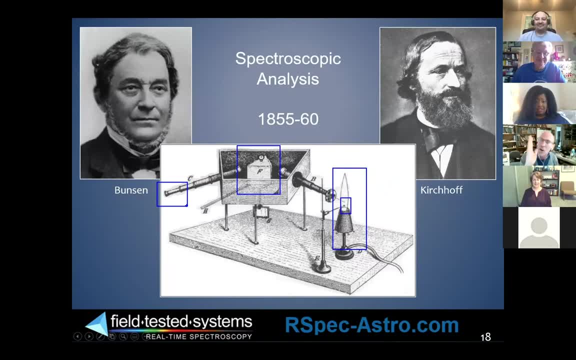 everything he could find almost literally And he was noticing. and the reason he did this is because he saw different patterns of light And we're going to look at those patterns in a minute And what they can reveal about a star. Now, Kirchhoff over here was a contemporary They knew. 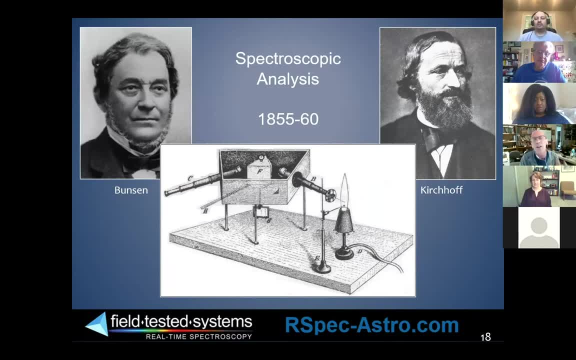 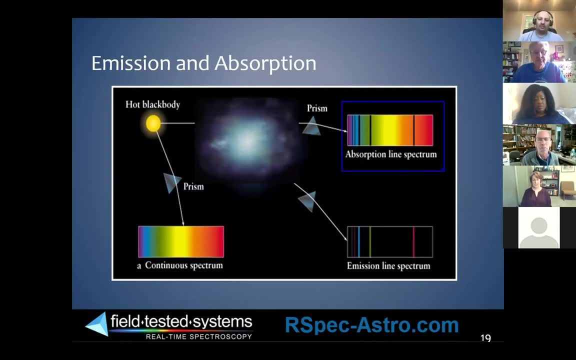 one another And Kirchhoff formulated some rules to help us understand what we were seeing. We're not going to get into a lot of the science tonight, But the one thing I wanted to point out is, if you look at this spectrum, notice that it has a rainbow with some dark lines. Those are 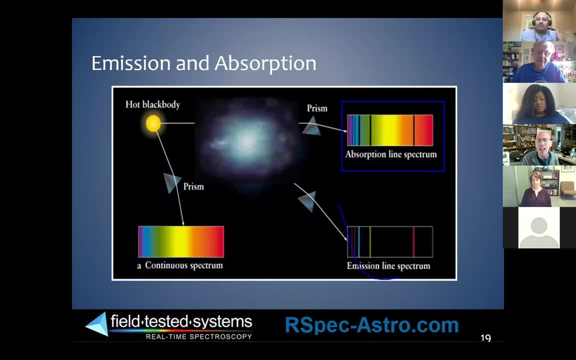 called absorption lines. But if you look at this spectrum down here- what happened to my box- then you have a dark area and some emission lines. The interesting thing about these is the lines are in the same position for a given star or material. What differs, and the reason we get lines like this, is because of reasons we're not going. 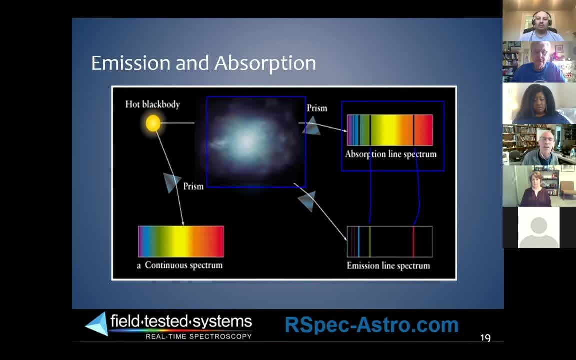 to discuss, but the temperature of the gases, the light is going through. I don't know if you just heard that Some reminder. Oh, it says I have a talk to be giving that I'm now 15 minutes late at. Okay, let's move on. So these are chemical fingerprints And you can see that each type 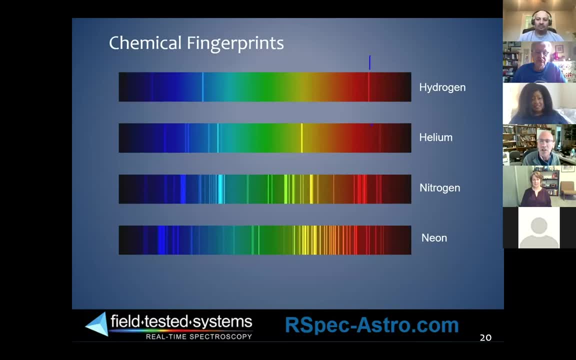 of element has its own line. So this line exists in hydrogen, but it doesn't exist in helium. Bear with me, This is a review for many of you, but we'll move on past this in just a moment. Now the hydrogen lines are so. 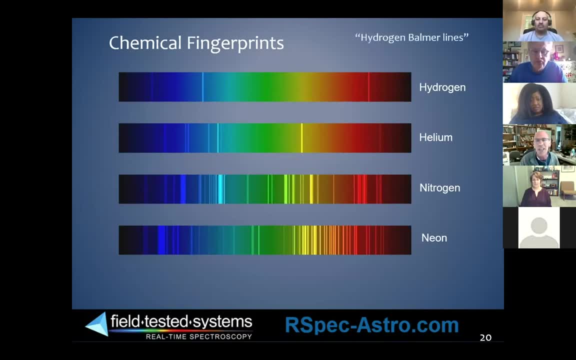 common and so important to us that we've actually given them names: Hydrogen, bomber lines- and there are the names of them, just our standard Greek names. We'll be seeing those because they're like a lighthouse. They really help us navigate. You're going to get tired of hearing those. 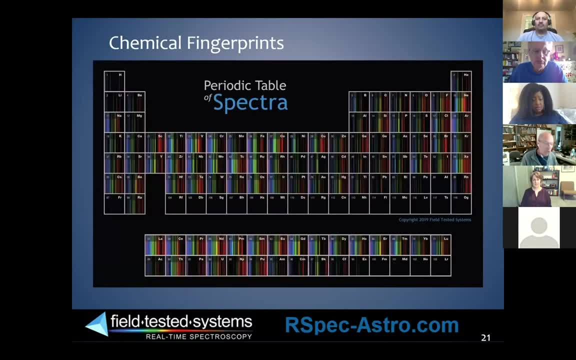 hydrogen bomber lines in the next few slides, So I wanted to show you this. This is a periodic table. This is the last chemistry diagram we'll look at like this. This is actually a poster that we created here in cell. You can see there hydrogen- There's those bomber. 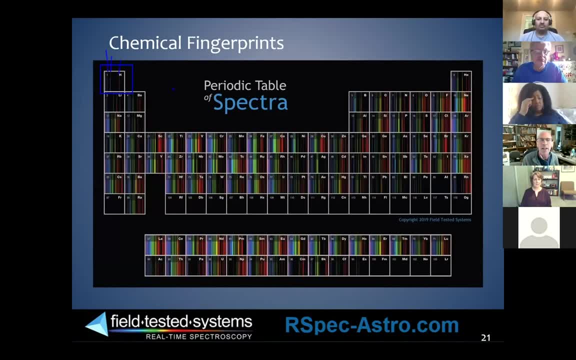 lines: hydrogen, alpha, hydrogen, gamma, hydrogen, beta, vice versa. But look over here, The helium lines are very different, right? And if you look over here, for example, the lithium in your cell phone battery, it's got very different lines. So all the elements have different numbers and 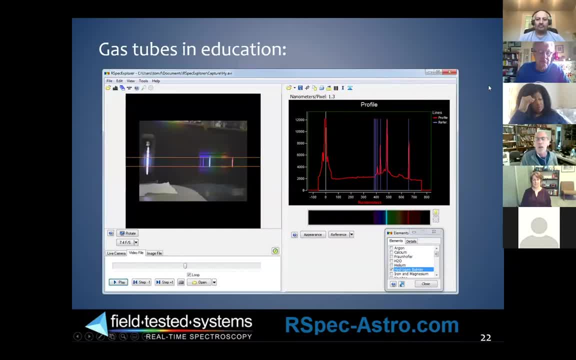 brightnesses of lines. And if you look over here, for example, the lithium in your cell phone battery, it's got very different lines. So all the elements have different numbers and brightnesses of lines. We can observe them without burning them in a Bunsen burner. But before I show you this slide, 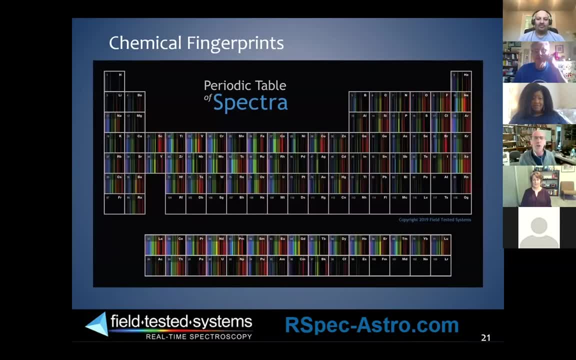 in fact let's go back so you're not reading all the fine print. I wanted to tell a quick story about Bunsen, And that is when he invented the Bunsen burner. he proclaimed- that's quite a word for a scientist to use- that he was not going to patent it. He said I'm going to release this for. 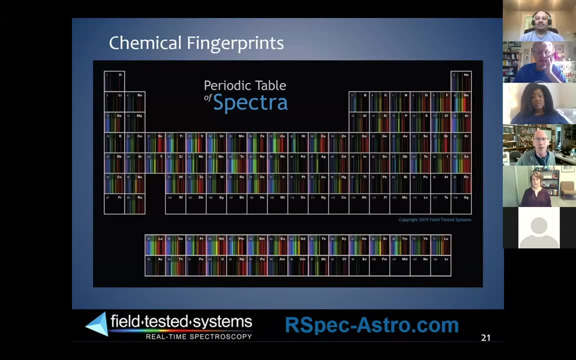 anybody to use, with no patents, no intellectual property, And he did that for the good of humanity. Now today it would have had 10 patents on it right, And we would have been paying for every one we fired up. So it's an interesting attitude that they had not that many. 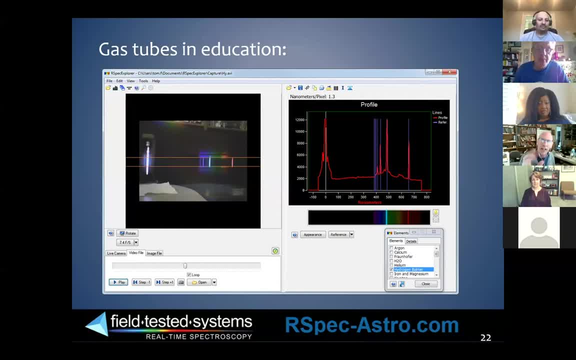 years ago. Okay, So instead of burning gas, like Bunsen did, we actually have gas tubes that we can burn gas in, And I've got one over here that I'll show you a little later. There it is, over there It's a gas tube. You can see. I don't know if you can see that light. Yeah, I guess you can. 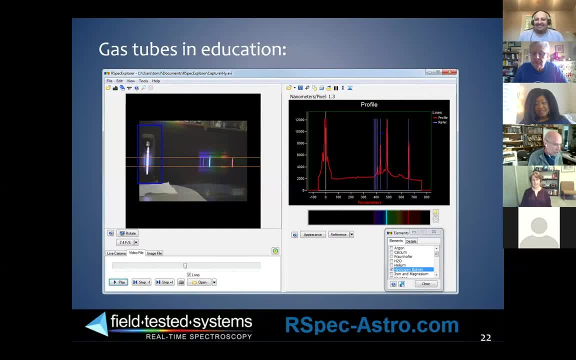 I haven't shown the gas tube in the talk before but I thought it might be fun just to show it in passing. as we move through Down here you can see the hydrogen bomber lines. There's a hydrogen alpha beta gamma. Getting the idea about those bomber lines, I hope. So now we actually sell a little. 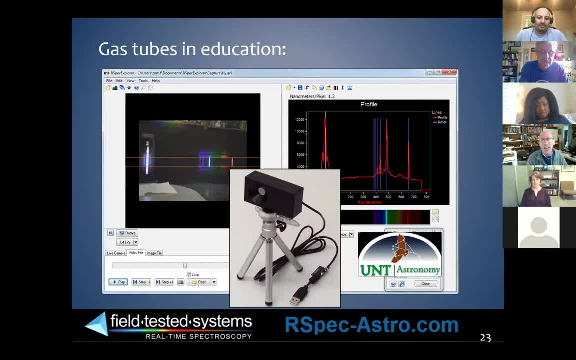 tripod-mounted spectrometer for educators to use in the classroom on gas tubes. And we did a fun project, by the way, at your state with the University of North Texas. They run 2,000 liberal arts students a year through a lab doing spectroscopy with that device as well as with. 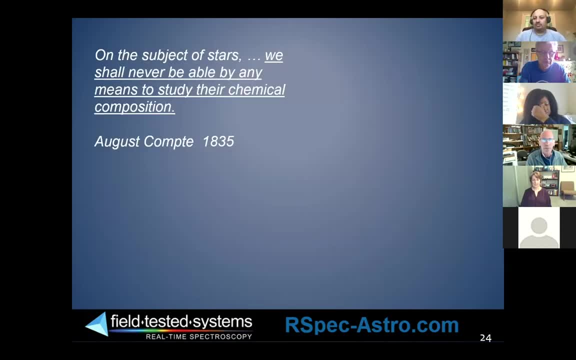 the other things I'm going to show you. It's an unbelievable number. So a little bit before Bunsen's time, this French philosopher said: we're never going to be able to study the stars: They're too far away. It seemed very reasonable at the time, But several decades 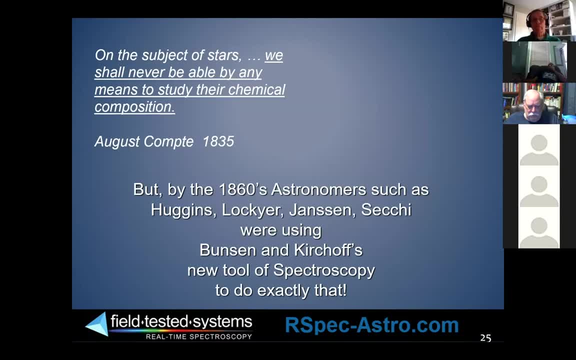 later all sorts of people were capturing spectra of stars and we were beginning to understand the stars. So again, we have somebody from Italy here, We have UK here. The French have always done a lot of spectroscopy, So Comte was wrong. But of course paradigm shift and people are. going to be able to do a lot of spectroscopy. So Comte was wrong, But of course, paradigm shift and people are going to be able to do a lot of spectroscopy. So Comte was wrong, But of course. 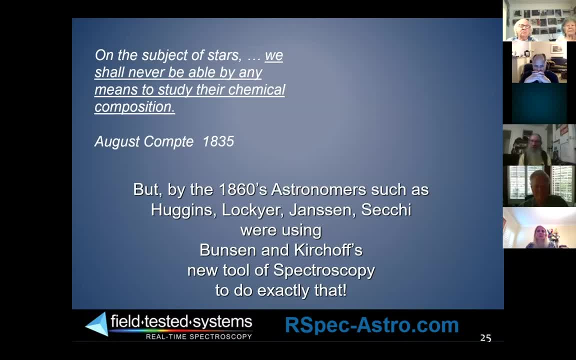 people learn new techniques and new science. It's interesting to think, 100 years from now, what the science will be and how they might look back on us and go: they didn't know this. Can you imagine how primitive- not primitive necessarily, but how starved they were for knowledge and maybe? 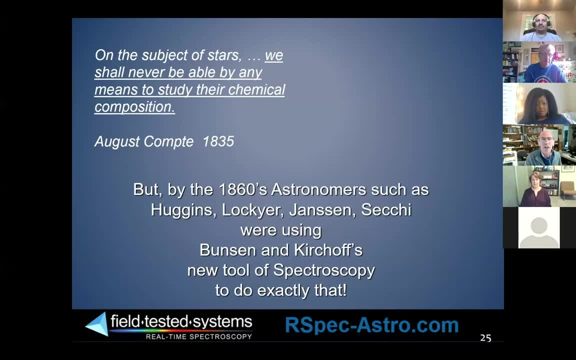 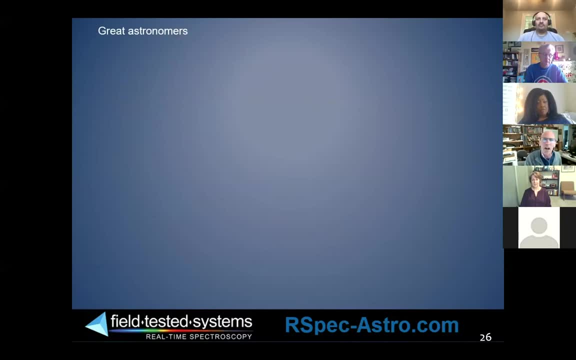 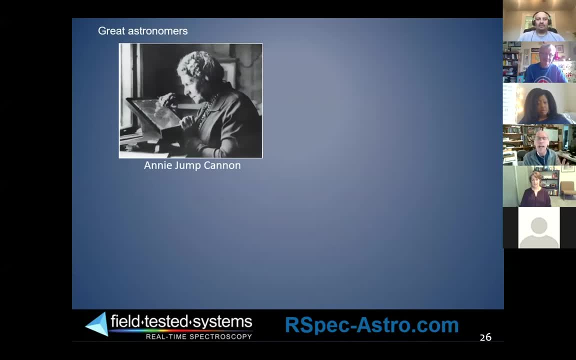 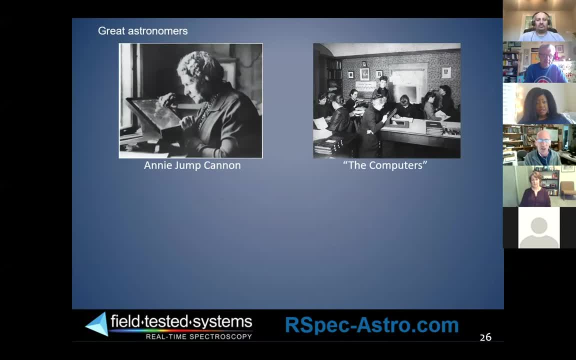 prohibited from getting access to telescopes, And so, to our great fortune and maybe theirs, instead of late nights in front of a telescope, they got to work during the day examining glass plates of spectra, And through their diligence and exactitude and creativity they came up with 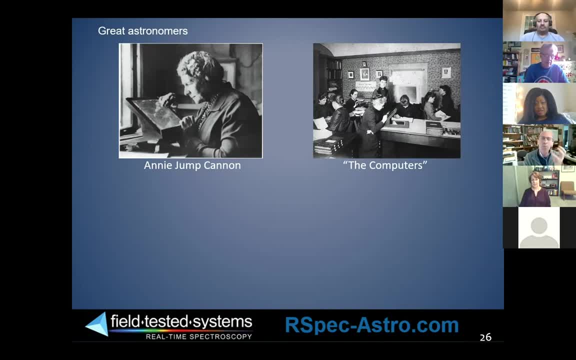 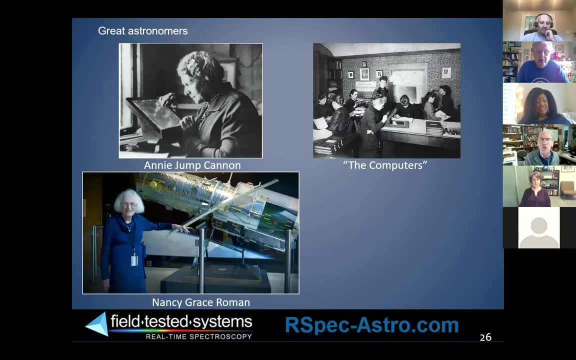 the star classification system that really helped us understand the evolution of stars. Nancy Grace Roman was a woman. she was the first astronomer for NASA. She got her PhD in the late 40s And the Hubble Space Telescope was her vision, her dream. she made it happen. really remarkable. 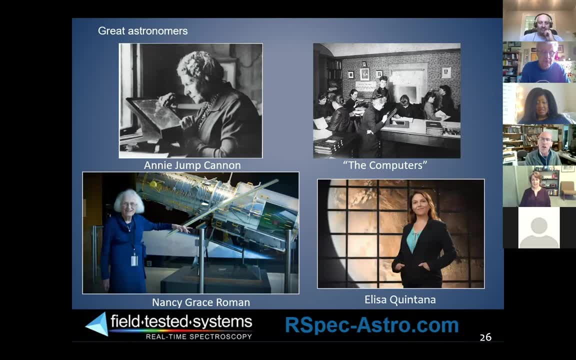 And Elisa. here is a modern-day current astronomer And because I don't live, I don't speak Spanish, I'm not going to try and pronounce her last name, which is unfair of me. This is only the second time I've done this slide in a talk. I'm going to learn that name before I give my second talk. 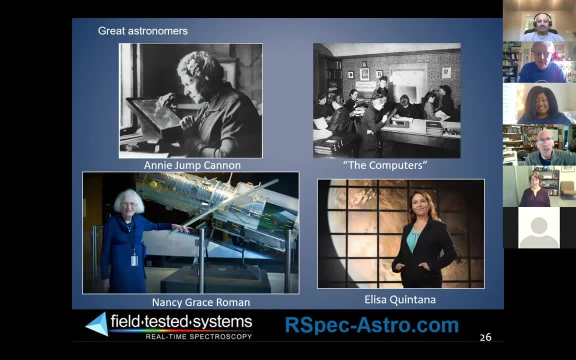 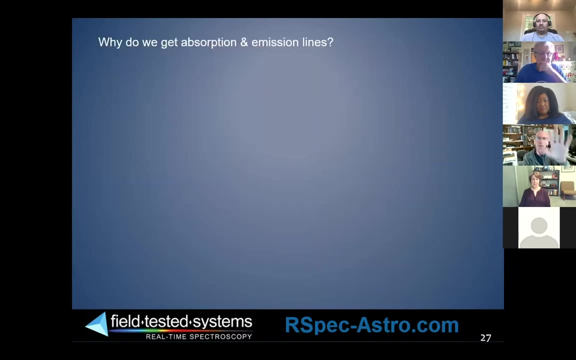 tonight, But she is an exoplanet discoverer. She discovered an exoplanet around a late stage or a cool star, and the planets are just the right distance that it could have liquid water, And so you know there could be life there for all we know. So how do we get? and again, bear with me, we're almost 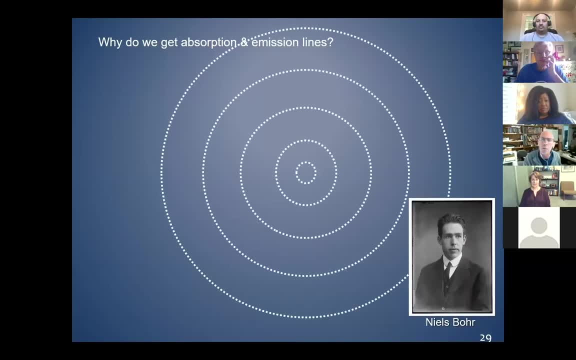 done with the science. How do we get absorption lines? Well, the Bohr model has electrons circling in shells around the nucleus of the atom And when they jump between levels they give off energy Right, Just like when you drop a ball on the Earth. once it's reached the Earth, it's less energetic. 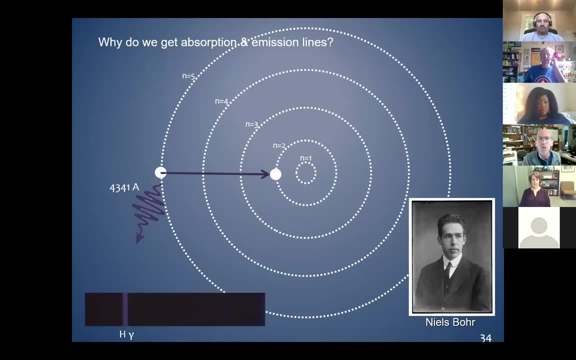 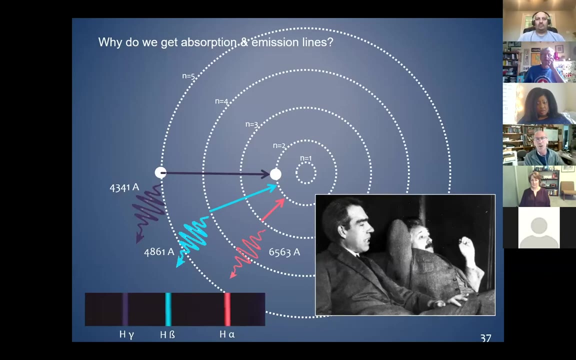 It doesn't have that potential energy in it, And some of that energy we can see as spectra. Different jumps produce different colors. Look there, we got our hydrogen alpha, beta and gamma again. So that's the spectral lines for hydrogen. This is a picture of Einstein that I love only. 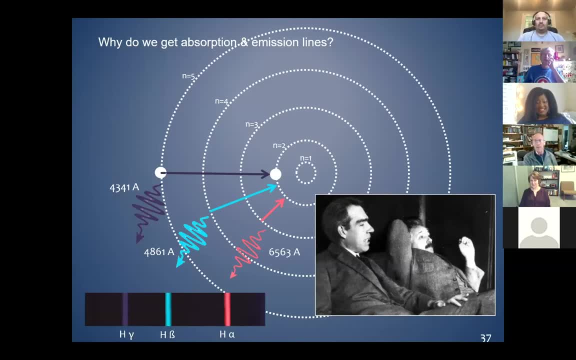 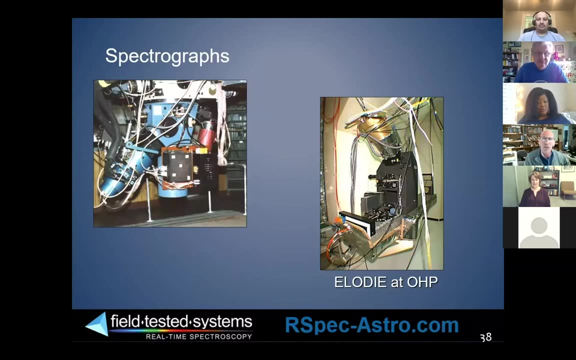 because- and he's with Bohr, Look at his posture there- I mean, is he kicked back or not? Okay, here's some examples of some professional spectrographs. The one on the right in France discovered the first exoplanet, And we'll look at an example that shows how that's done later. 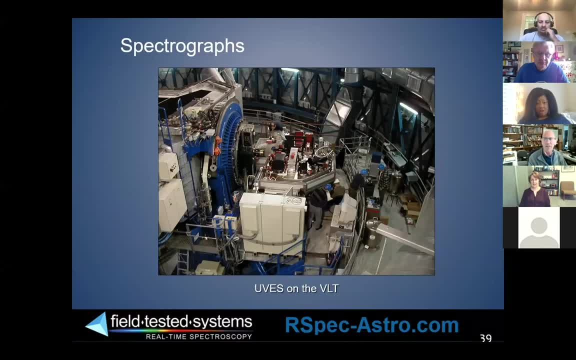 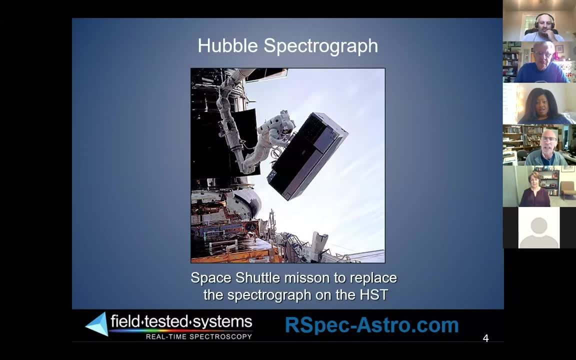 Here's a spectrograph down in Chile. It looks like just a lot of equipment until you look at how small the people are in that view. And this is the Hubble spectrograph getting serviced by the space shuttle. Now my son says that's not a spectrograph, He says that's a refrigerator. It's filled with. 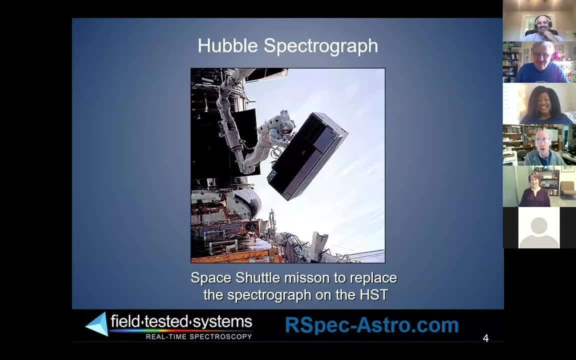 beer. And at night, which happens to be the worst thing in the world. It's a refrigerator, It's filled with beer. And at night, which happens to be the worst thing in the world. And at night, which happens, happens fairly frequently on the space shuttle or did. they are party animals and they're drinking. 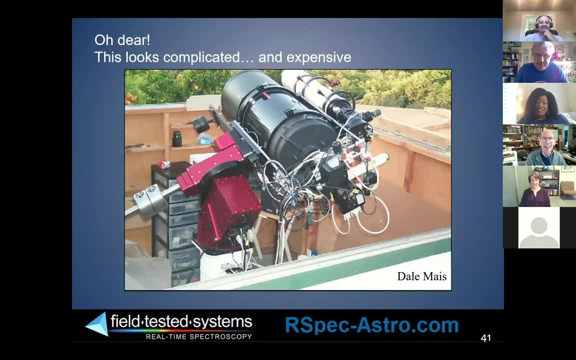 beer. now i can't prove wrong, but i think he probably is. so here's an amateur device. dale, i think, regrets having ever shared this and giving me permission to use it is far more complicated than any of us typically need. what i like about this device is down here is a gas tube that he 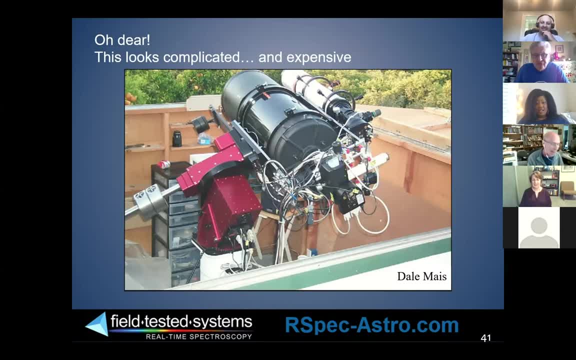 shoved into the telescope. and, in particular, what i like about it is these, these pins that are right there. you think about a, you know, a neon type tube. it's got two little pins on the end and i pictured dale with like two high voltage alligator clips clipping them on those pins and the problem. 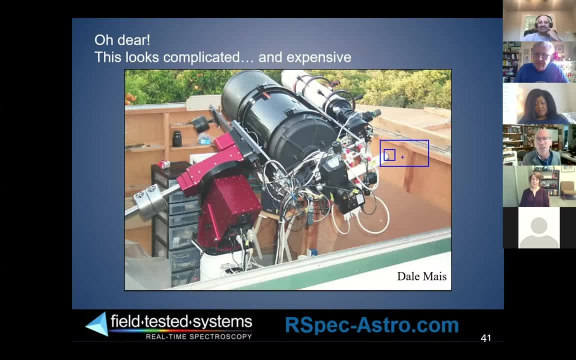 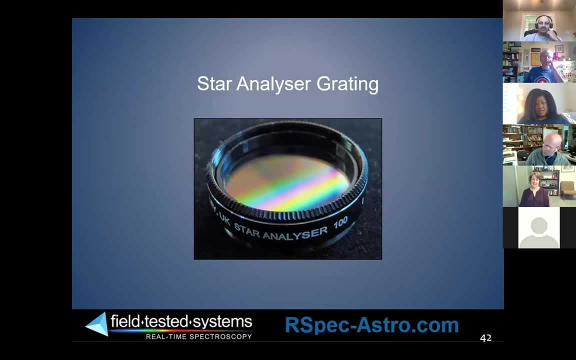 is, if he draws a spark, he ruins his night vision, right? so what i want to talk about tonight, now that we're through most of that technical stuff, is i want to talk about this grating here, which is a diffraction grating. it has 100 lines per millimeter and you can see it there and now. i 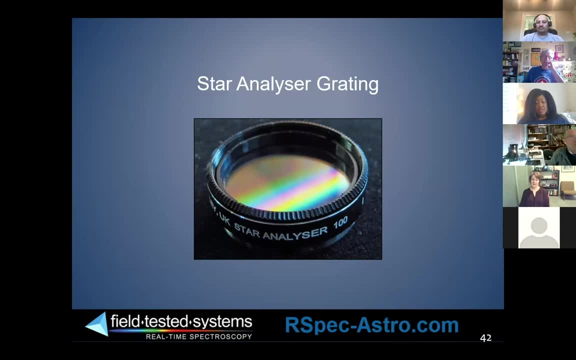 am going to try. i tried it earlier and it seemed to work. i'm going to turn on our gas tube and i'm going to hold this up and you're going to see, uh, oh, there it is in the upper, there it is diagonally. you can see a. 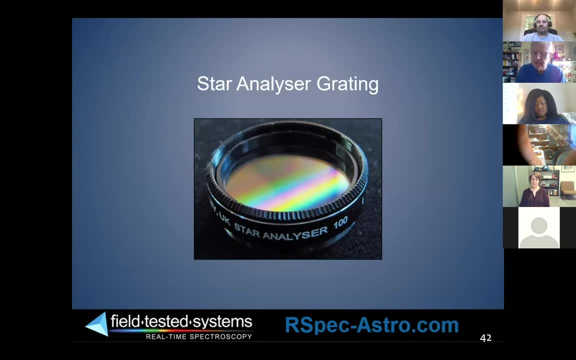 spectrum. there's actually multiple spectrums end to end. there. you see some red and some green, so this is splitting light. it's an inch and a quarter grating and so it will uh thread on to most any camera that you've got. uh, and we're going to talk about how you can use that to do some of the things. 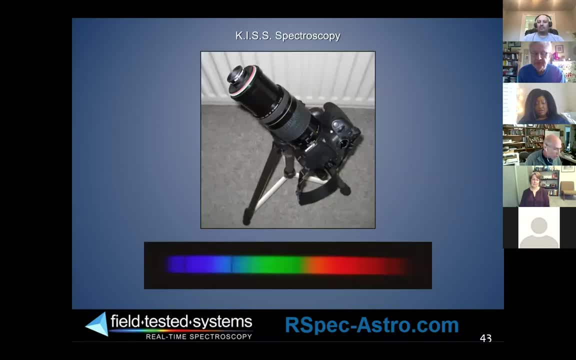 we're going to look at tonight. um, it costs 200 bucks. so here's a little bit of information about what we're going to talk about tonight. here's the first example i wanted to show you. uh, it's got the star analyzer on a dslr notice. there's. 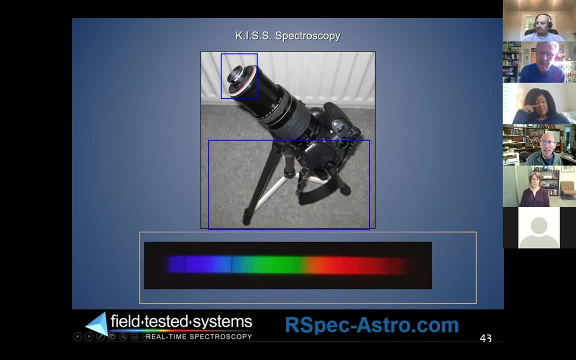 no tracking, even though there's no tracking down. here we got a spectrum and what do we get? hydrogen alpha- yeah, you're getting the hang of it, i think- hydrogen alpha, beta and gamma. so this is a little hard to do because it's a drift image, so you got to get things aligned in a small aperture, so i 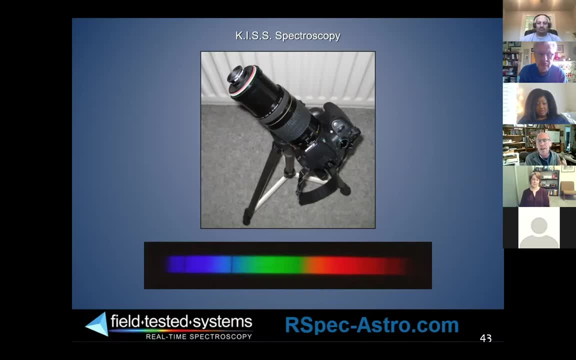 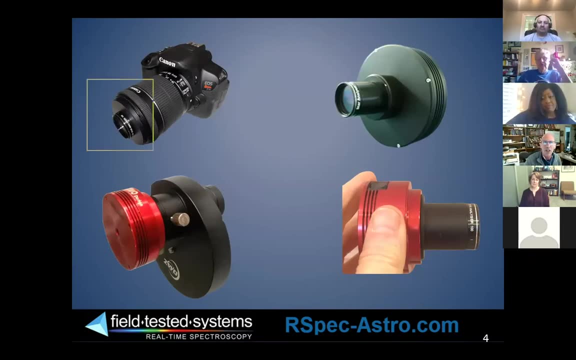 show that as an example as to how simple things can be done, but uh, it's, it's not the preferred manner at all. there's lots of other ways to mount a grating on a telescope or a camera. this is the one i just showed you, more or less. 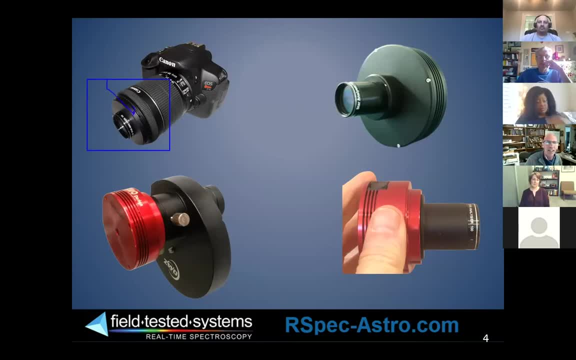 uh, and we actually, uh, have a little adapter, that's a terrible arrow that screws into the lens cap threads of a canon camera so that you can mount it that way. it's called an objective prism. in that configuration, uh, you can also use a standard fits camera. the camera can be color, can be mono. 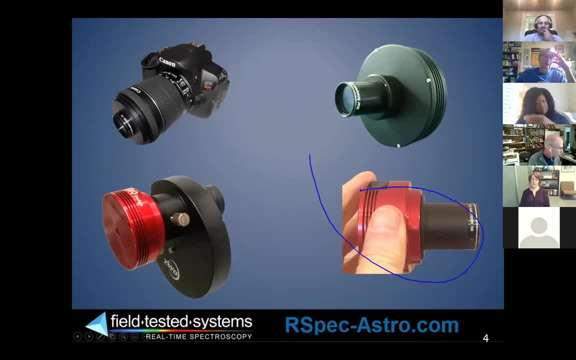 can be a video camera like this here. this is a zwo camera- not that you need to see one, since you're probably familiar with these kinds of enclosures, uh, but it just as you can see. it's a standard fit camera and you can see on. in this case it's just threaded right onto the nose piece. 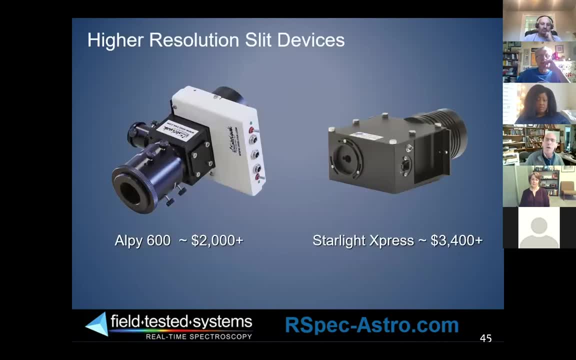 and you can also put it in a filter wheel, so there's lots of ways to mount these things. there are higher resolution devices. you can see they're also higher priced. these devices have a slit. a slit is a great thing. it great. it creates higher resolution spectra, but it also means you. 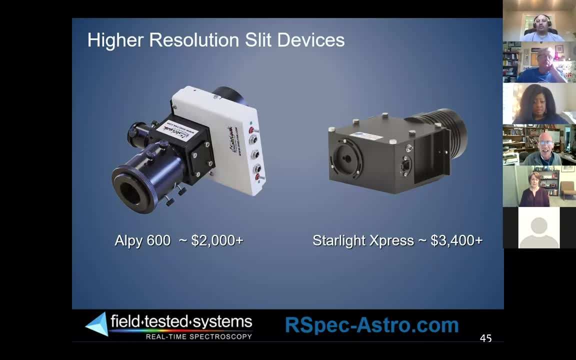 have to acquire a target and guide on, typically a 20 micron slit. it's harder to do, they're harder to use. uh, a one in a thousand people seem to start with one of these. but you can also mount it on a star analyzer. most people start with a star analyzer and uh, learn, learn the ropes that way. 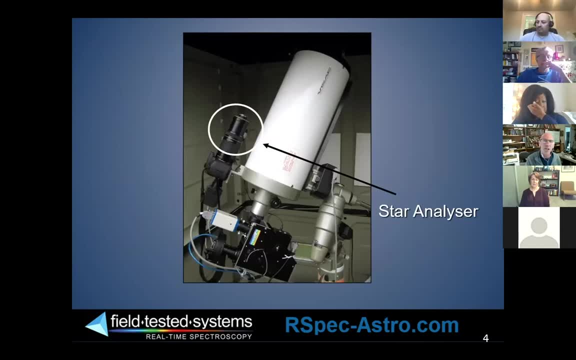 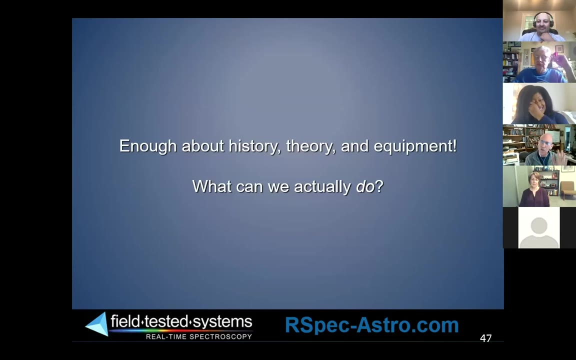 uh, some people do both. you can see a star analyzer piggybacked on the telescope, and down on the bottom here you can see, uh, a higher resolution device that's like a 3200 device. okay, now we're done that sprint. so we've seen the history theory equipment. what can we actually do? that's why you're. 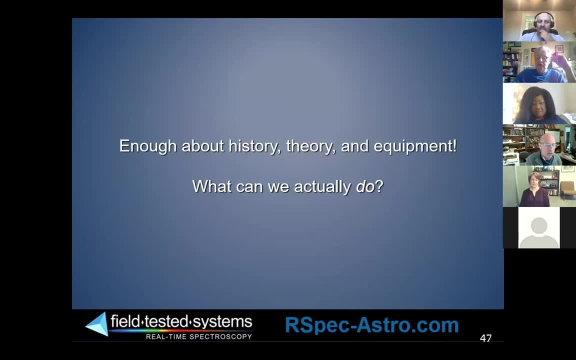 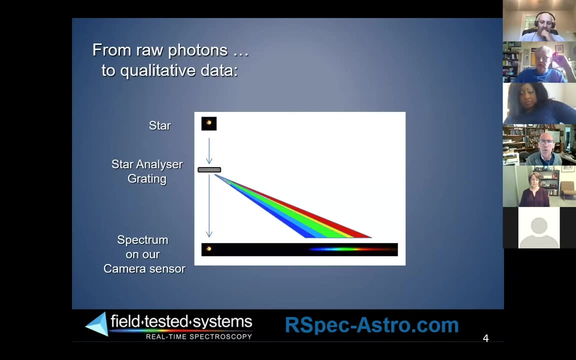 here tonight, but now we've got everybody to the same level, so i appreciate your suffering through it. and uh, a second question, and the question is: do you really need the current equipment we need to be able to capture linear modes of light in a telescope. it's not a big deal, that's actually. 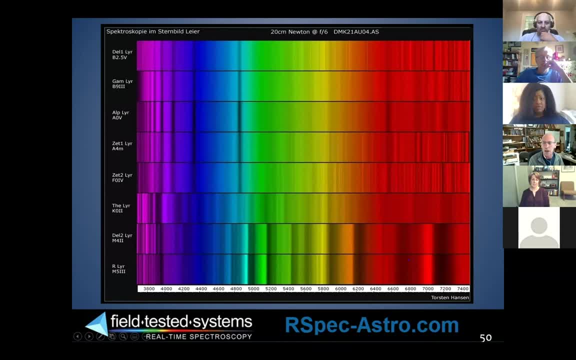 an easy one to do, so we're gonna go ahead and talk a little bit about how that works, okay, so let's start by saying we'll talk about a little bit about theantis, which is a very popular technology we use in the lab, within the lab, and it can capture images. now, this is the first thing. 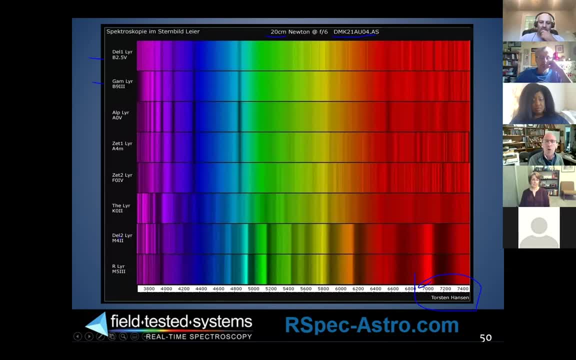 that we put. we put starlight through a grating, we get a spectrum and we can capture that spectrum on our camera. here's our first example. this is a series of different spectrum. these were captured by torsten hansen down here with an eight-inch telescope and one of those imaging source video cameras. so we're not talking long exposures here. 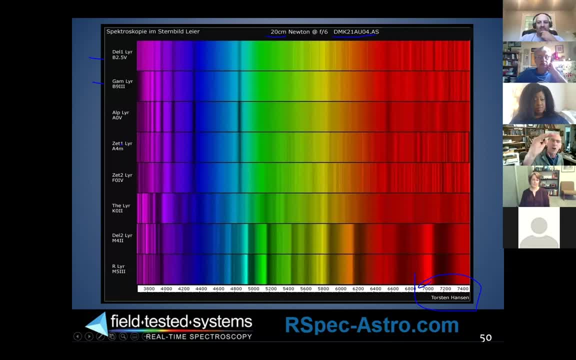 A stars. So for those of you who aren't familiar with this, the stars were classified originally by the women that I showed you in that earlier slide by temperature order, And there's a reason the letters are this way, but it's a historical reason, We need not get into it. The stars at the 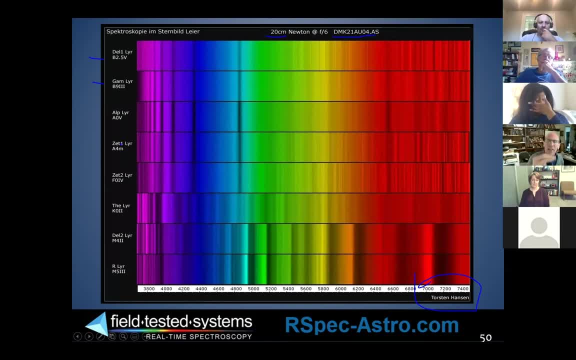 top are the hottest stars and the stars at the bottom are the coolest stars. Take a look at that Now. you see those differences. So different stars have different spectra. So we're already able to do a little science and tell something about the temperature of stars right So down. 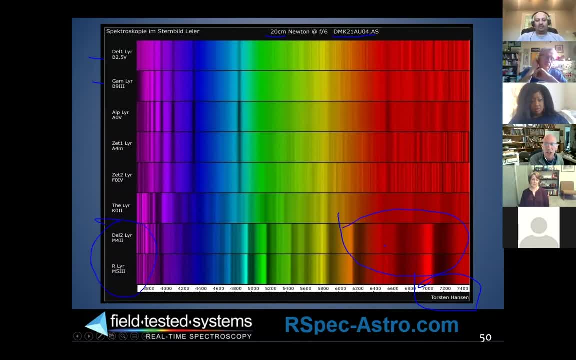 here, these stars, these cool type M stars, have these wide bands, right, But these stars up here they don't have bands, but they have this, which is hydrogen beta at about 4,000 angstroms. But notice this: hydrogen beta is darker and wider. 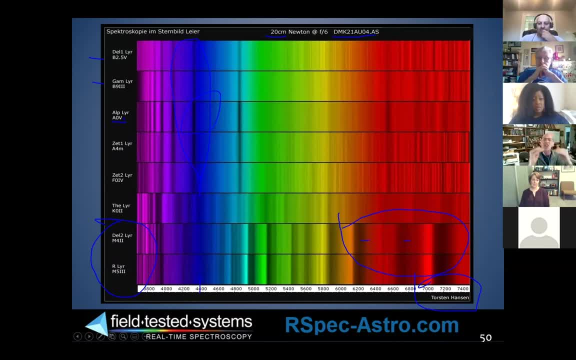 On this type A star. So A stars seem to be just the right temperature to get the most number of electrons jumping between shells, creating that absorption line. These hot stars at the top they are a little too hot and the electrons, a lot of them, just bounce right out of the star as 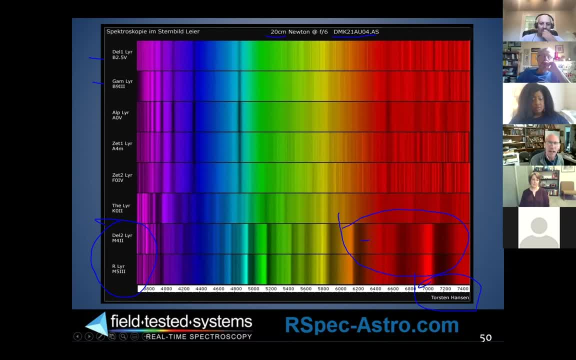 if? And these hot stars, oh no, oh yeah, that's right- And these stars down here don't pump up enough energy to get those electrons to jump between the shells that close that line. So this is again. now we're looking at the temperature of the stars and we're looking at the temperature. 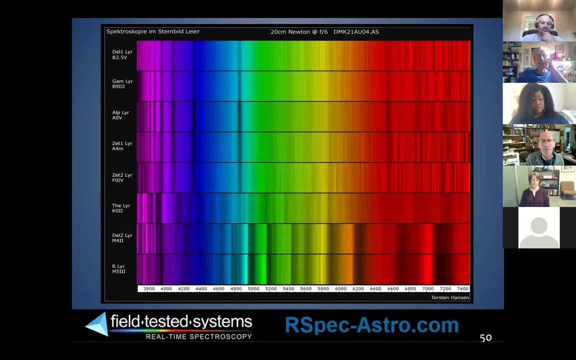 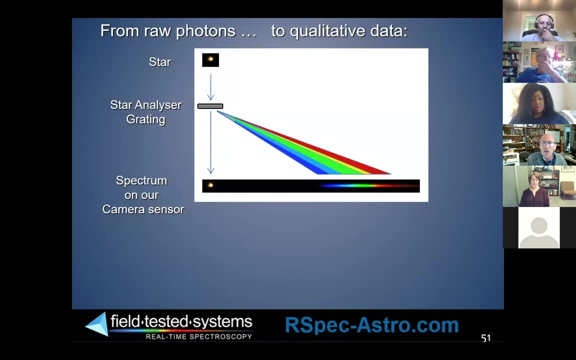 of the electrons that jump between the shells, that close that line. So this is again. now we're looking at star temperature as well as composition. right, If we're seeing hydrogen lines on a star, the star has hydrogen somehow. So now, if I was to show you this and look at that spectrum on the 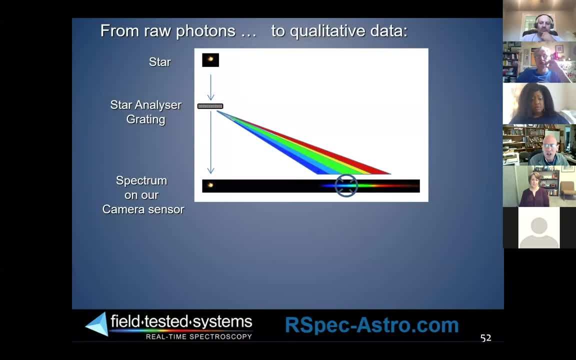 sensor there and see that crosshairs down there. if I was to show you that- I don't know how many of you can see that it's a little bit dimmer between those crosshairs where they cross. Can you see that people with video? Yeah, Joe's nodding his head, Thank you. So to do science, I can't. 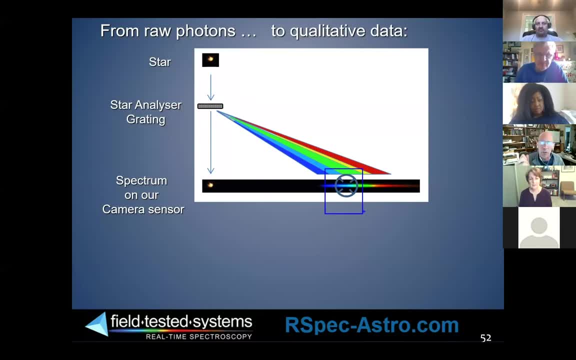 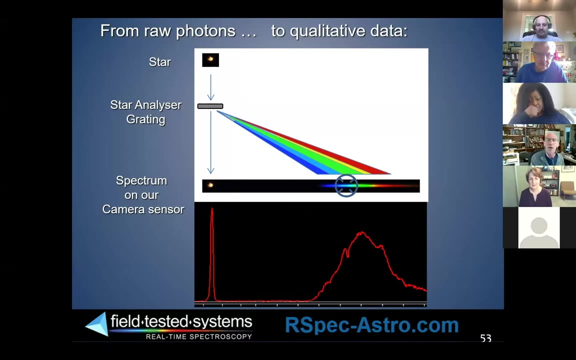 write a paper that says, yes, we used the Hubble Space Telegraph, yeah, telescope, and we saw a little dimming in the robin egg blue. That's not science. What science is is actually quantifying that data and representing it. This is an intensity graph. We'll spend just a moment looking at it. 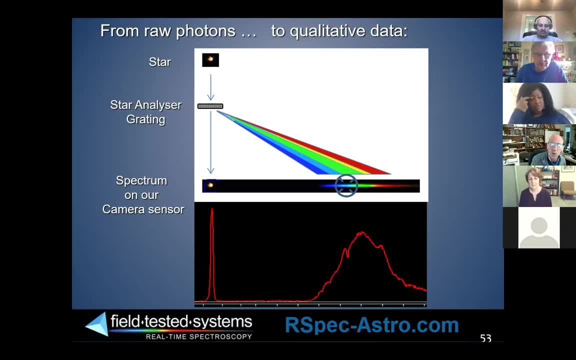 because this is the way we look at spectra. So this star is really bright, so we have a really bright peak of data here. And this star is really bright, so we have a really bright peak of data here. So this thing goes from dim, bright, bright, bright, dim. right, It's much brighter here in. 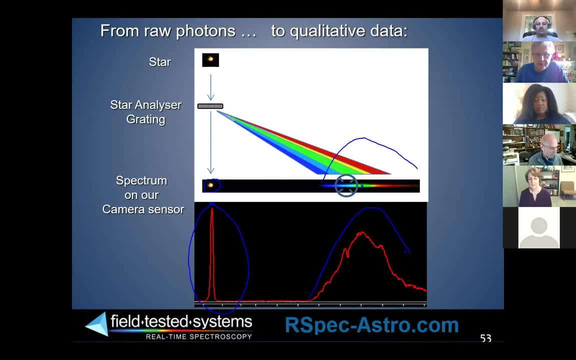 this green area. So this goes from dim, bright, bright, bright down to dim. So the cool thing is that that dip in the red curve is quantitative. Now we can study its width, full width, half maximum, its position, what color it is, how it compares in size and depth to other stars, to 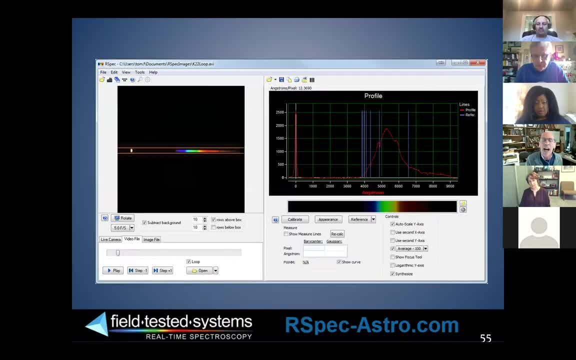 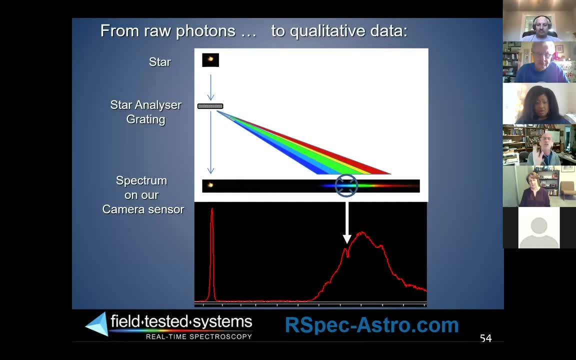 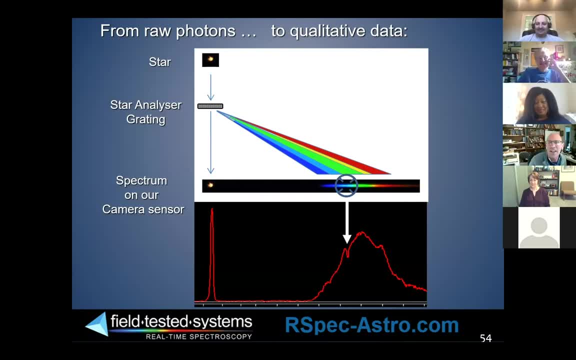 come back here so you you're not reading screens while I'm talking. So that night I went out here three miles from so late In my backyard. I came in at midnight, I'd been looking at Vegas and my blue jeans had grass stains on the knees. Next morning I was all excited to look at my Spectra. I looked at 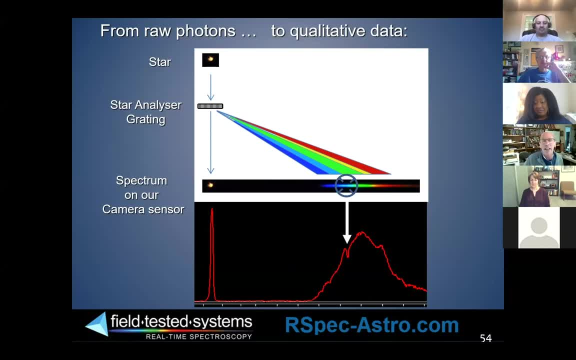 some of the freeware that was out there And literally two hours later I gave up, literally here, threw the star analyzer in a drawer and said: I don't want to do this, I'm not having fun, The software is hard to use, It crashes, It's in French, There's no manuals And I gave up. But I 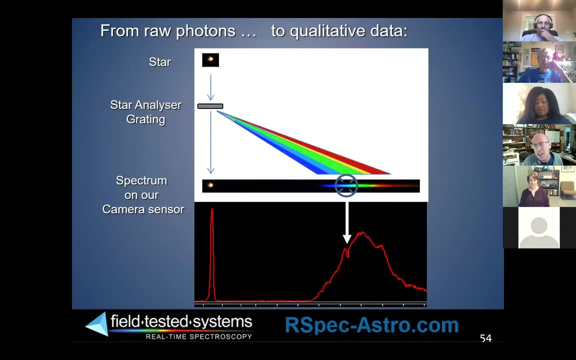 really wanted to do Spectra. So over the next week I kept thinking about it And I decided: okay, this weekend I'm going to write a program to convert the colorful rainbow spectrum into a graph. And now what? five to 10,000 hours later, the software is almost done, Almost. So I want to. 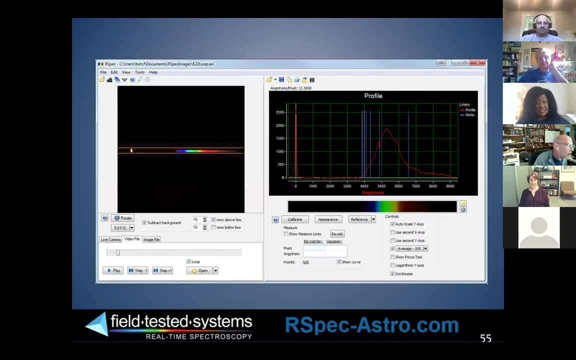 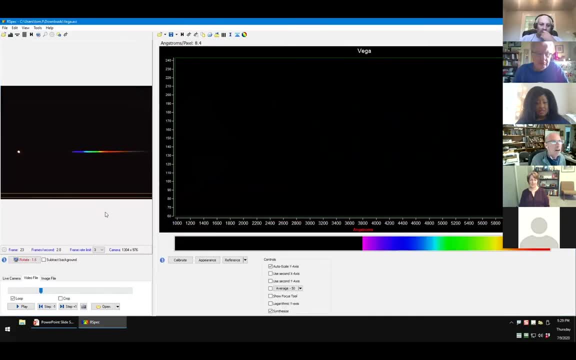 show you really briefly the software running. This is not a software demo. We're going to get back to real stuff in a moment. This is a software demo. We're going to get back to real stuff in a moment, But here's the software. I hope you can see that screen. I hope, Joe, you can see the software. 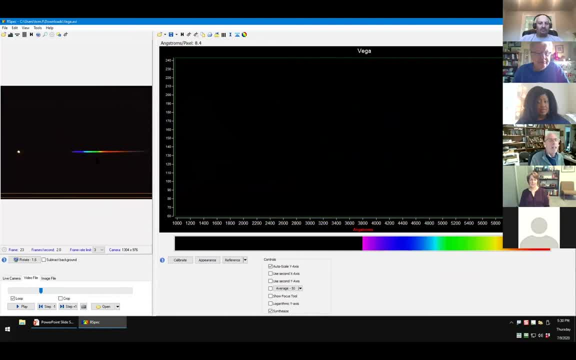 screen. Great thanks. So this is the image. It's in color, but it need not be. Color makes it easier to understand what we're seeing at first. Color cameras aren't as sensitive as you know. It could be a video. It could be a FITS image. Our software will automatically load whenever it. 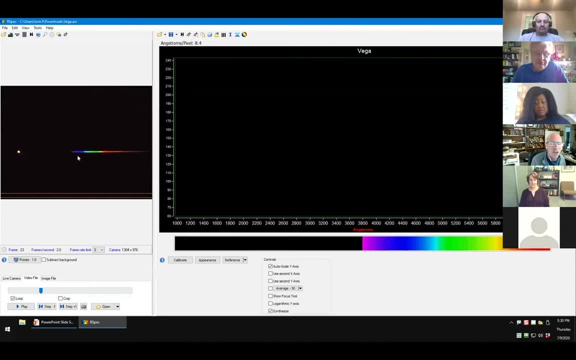 hits your hard disk or solid state drive. There's a star, There's a spectrum, There's some gaps. There's a big gap there. So now, if I drag these sampling lines around that spectrum, we get the graph I was showing you earlier. This peak is: 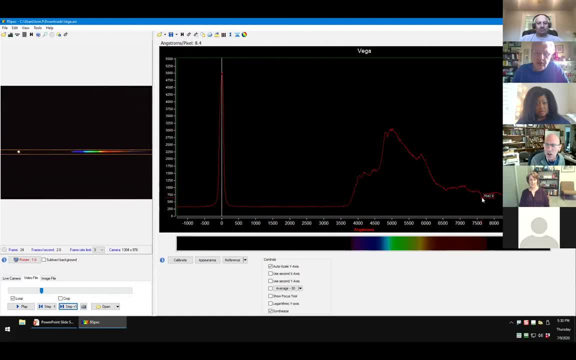 the star and this broad thing is that and that broad dip there is that. So now we're doing science. So- and this is in some steps I won't show you during my main talk- This axis is calibrated in angstroms. It's about a 20-second couple of clicks to do And now we see those dips. Now the real. 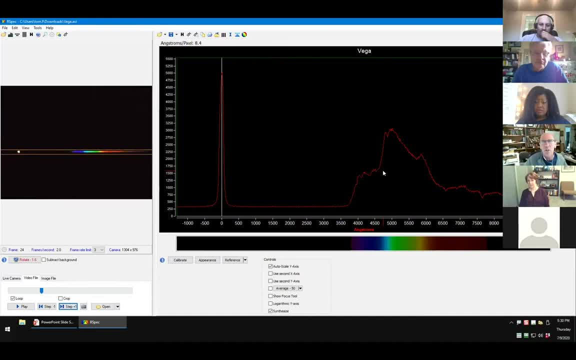 issue comes up, and I think this is a disincentive for all of us, including myself. when we get started, It's like: well, how do I know what those are? Well, one thing you can do is build into the. 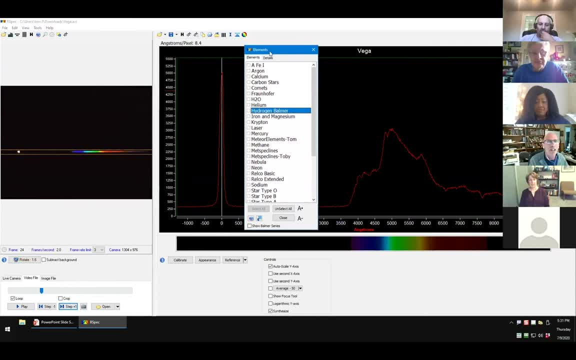 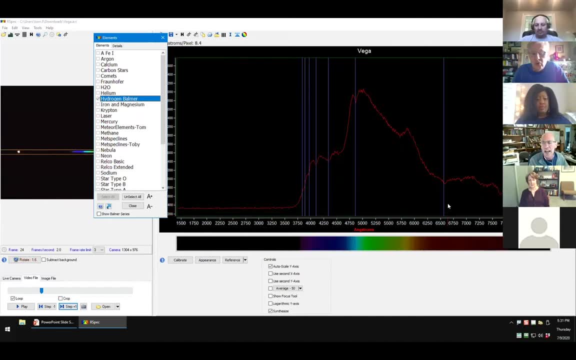 software is a library of measurements like Bunsen made So we can say: show me on the graph in an overlay where the hydrogen bomber features are, And look at that. We've got a line going through our dip there. We've got one going through there. That's our hydrogen beta, hydrogen gamma. 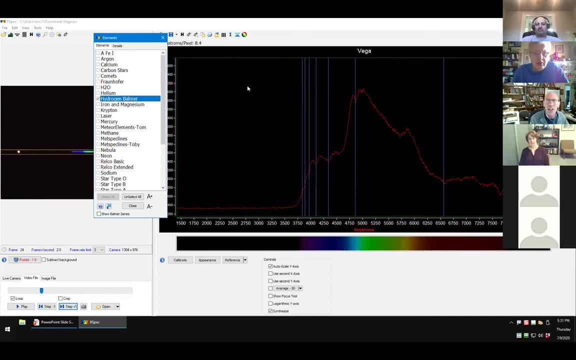 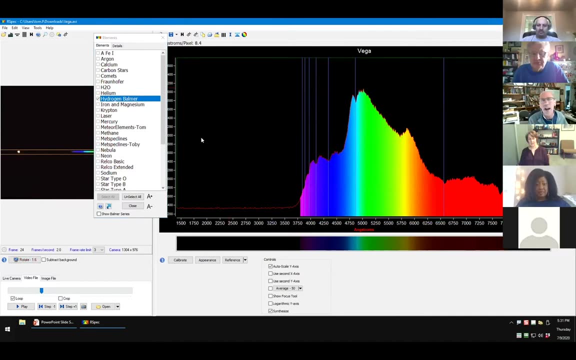 hydrogen delta. We've pretty well established that this star has a lot of very visible hydrogen absorption lines. That's the science that's fun to do Now. the other thing that we can do here is we can add some eye candy, and this is actually a frame from a video. This is the last thing I'm going to show you. 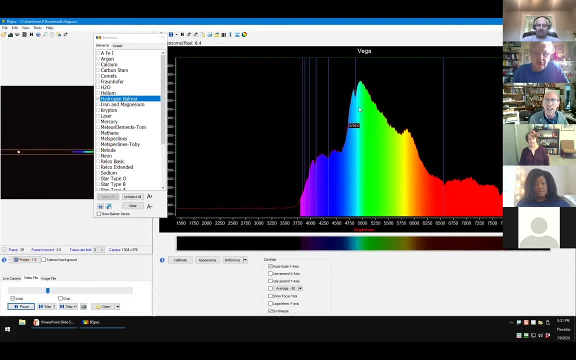 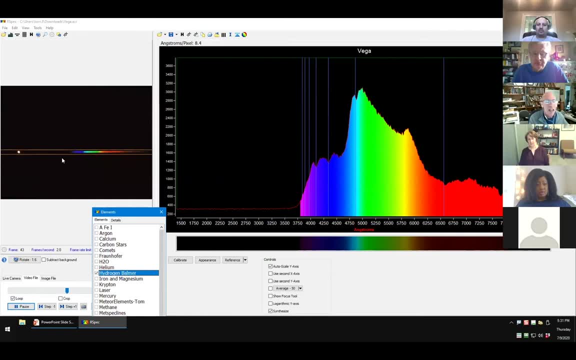 in the software. Let's play that video. You can see the image here. The graph is jumping up and down because our data is jumping them down from our scene. The video is playing at two frames a second. This is like a light to moths when you're doing a star party or some sort of public outreach. So 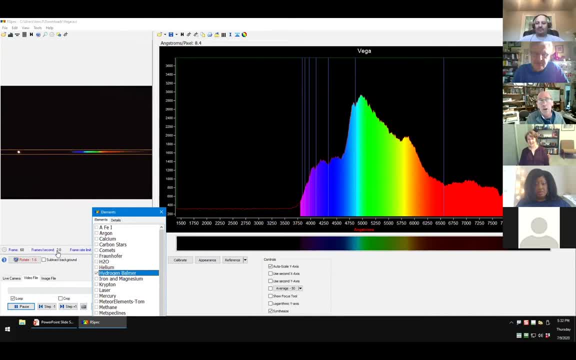 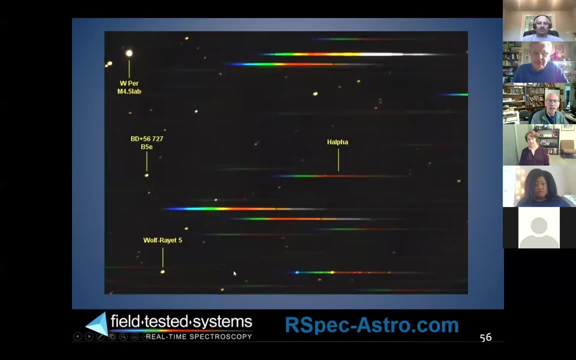 when we get back to that. this is the kind of thing that people really want: to know what they're seeing. It's a very interesting screen to show them. Okay, let me pause that and come back to the show and we'll dive into some examples. So this is a wide field example with a DSLR I want. 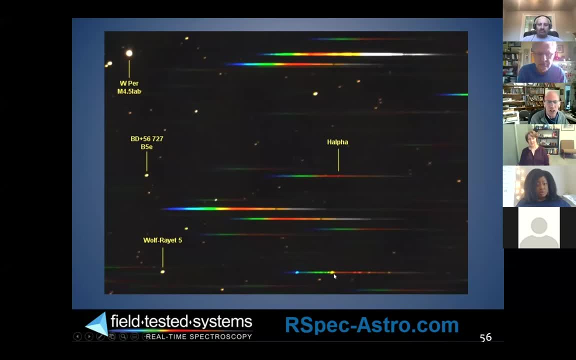 to show you this, first because it's beautiful. Secondly, to show you there's some emission lines right, Some bright lines, And there's some absorption lines. And then there's some emission lines And some absorption lines and of course, the parent stars are over here, to the side, to the left. 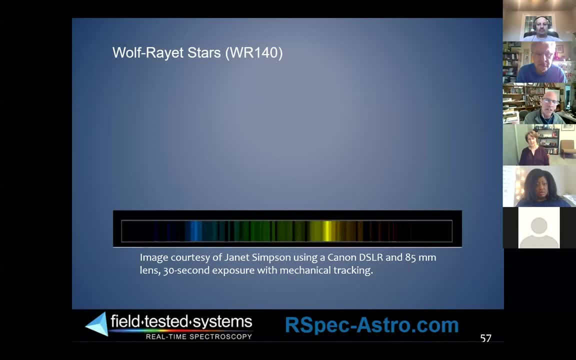 So when Janet Simpson sent me this spectrum she was in the UK and you can see down there. she did this with a cannon and just 30 seconds with a mechanical tracker. I have a confession to make to the group here. I couldn't remember what a Wolf-Rieh star was. Now I'd read about it countless. 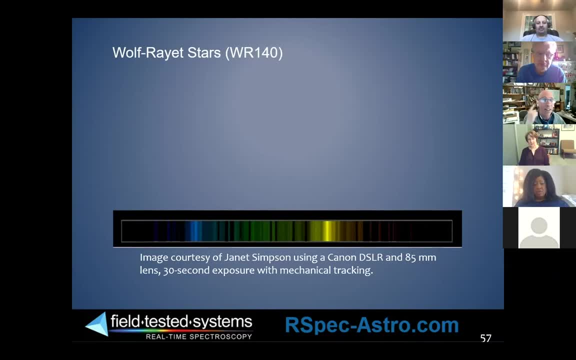 maybe five times in 20 years. but, like I said earlier, things go in one ear and out the other. Well, Wikipedia is your friend, Wolf-Rieh. stars are late stage stars. A lot of the outer shell of gas is gone, So we're able to see beyond that outer shell, where we'd see a lot of hydrogen. 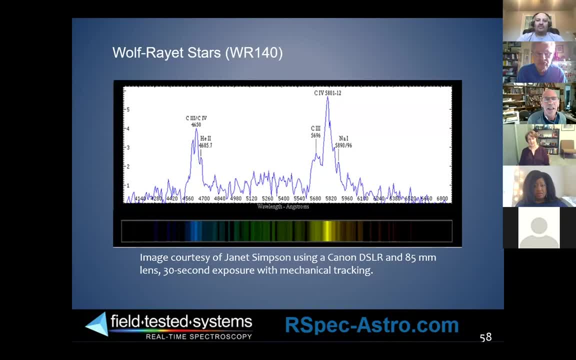 down into the core and we see a spectrum like this, And this spectrum is showing us a fair amount of carbon. right, There's carbon there, ionized carbon there. there's some helium, there's some more carbon. We are looking down towards the core of the star. This carbon is. 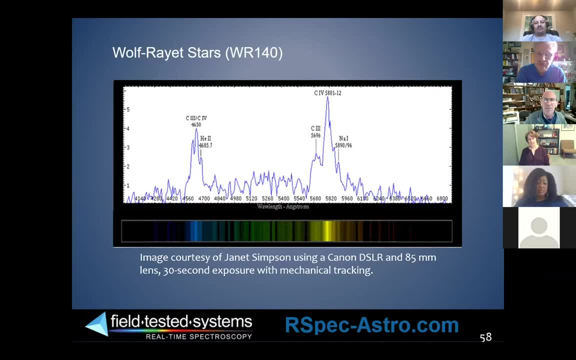 the bottom of the star. We're looking down towards the core of the star. This carbon is the bottom of the eye product of that star's life cycle, and we're seeing it with an amateur telescope, with an amateur telescope, With an amateur dslr: three inches of aperture and 30 seconds of. 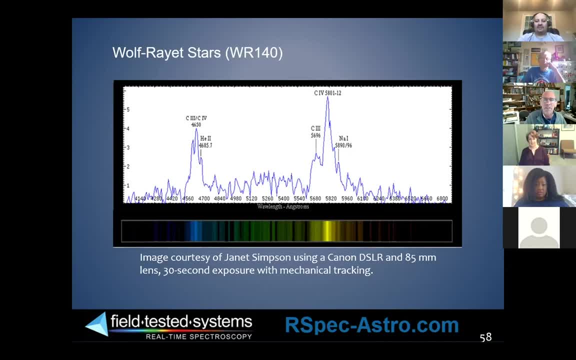 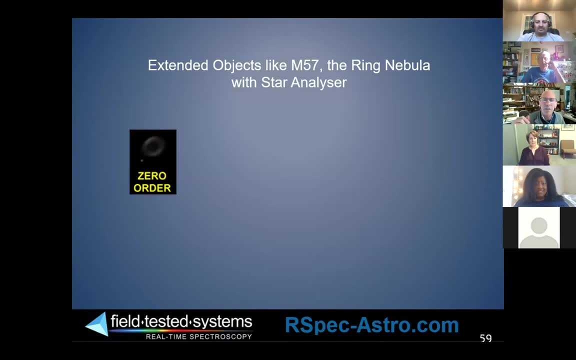 exposure time tracked pretty amazingly. So if we were to use a star analyzer in our beloved m57? for those of you who aren't familiar with this, Oh, now I got to get it right. It's a shell around a late stage star also, And that's what the spectra would look like, Because there are only 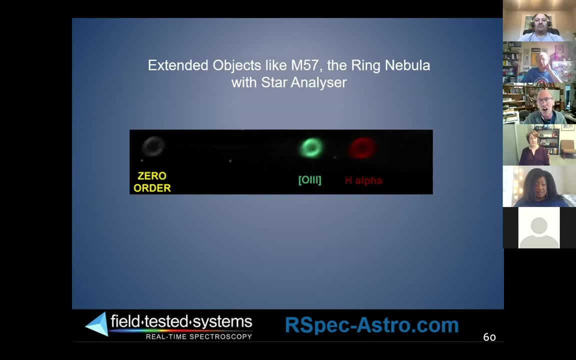 two things glowing on the star. there's really only two objects on the spectrum, But if this was a broad, much bigger object like a planet or a galaxy, there'd be lots of colors And because it was extended, they'd be all smeared all over each other there on the right. So one of the 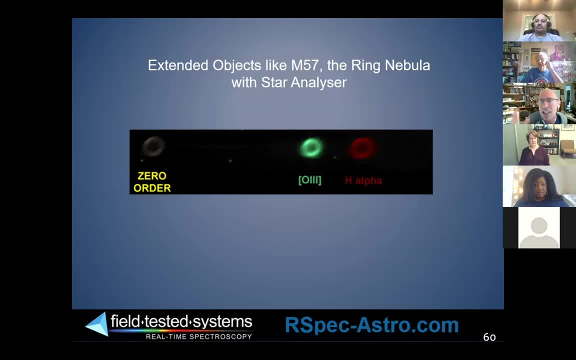 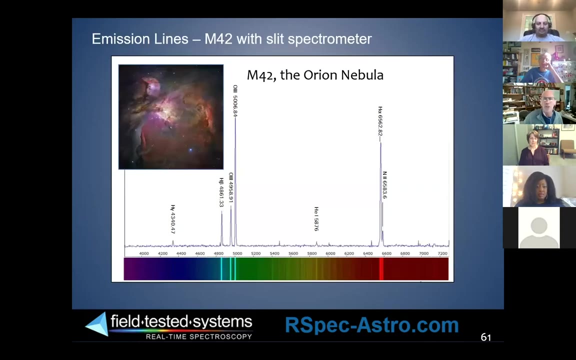 drawbacks of an inexpensive device like this is it doesn't have a slit. So you have to image objects that are like: what am I trying to say here? They look like they would appear in a slit, meaning very small. Let's look at an object like that: M42.. Again, they're all beloved to us, right? 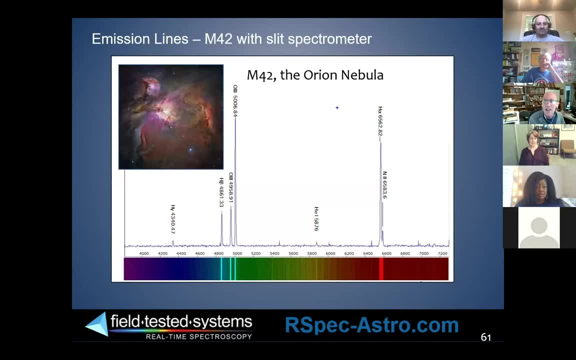 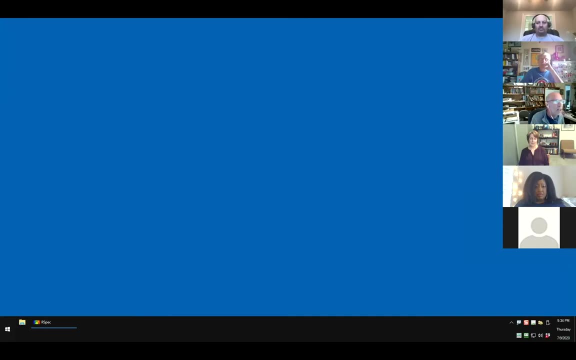 These are our showpieces, And here we can see same kinds of emission lines. They're very narrow here, even though it's a really broad object, right, So what I want to do here for a moment is turn off my screen. share Meeting controls are here. 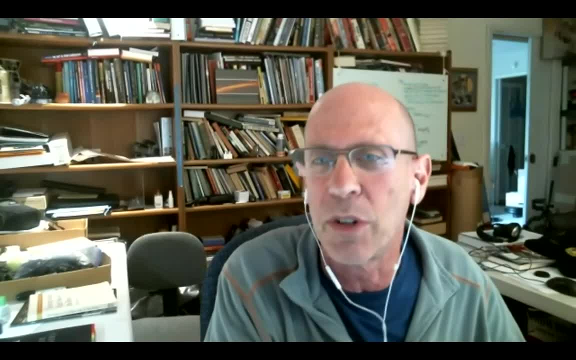 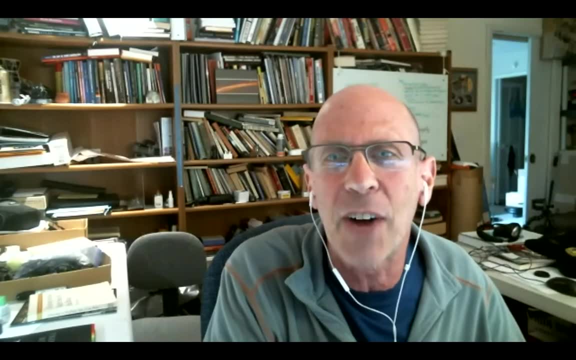 And now I want to have just a real brief discussion with you all. First of all, for those of you- and you probably all know this, but in case certain groups don't- if you're only seeing five or six named or video displays across the top of your screen, then go up to the upper right-hand. 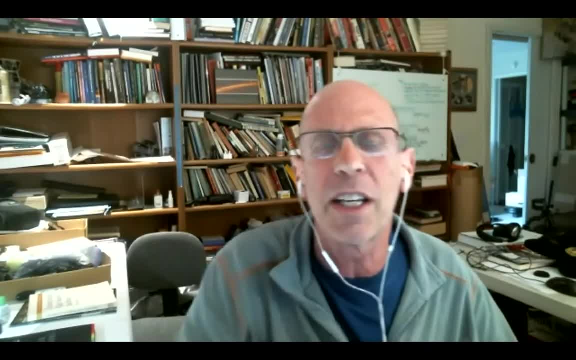 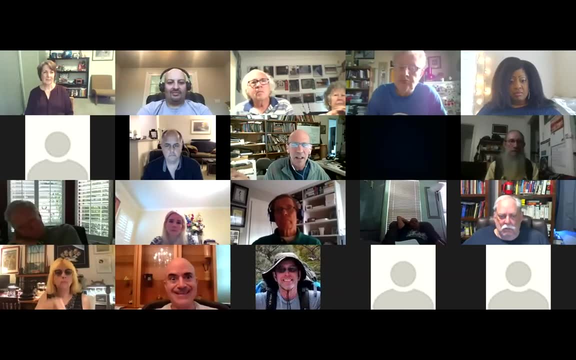 corner and click on that button labeled gallery view and you'll see 25 videos all simultaneously. So I wanted to ask a couple of you- hopefully with video or not- to unmute your mic and just tell us when you find it. How did you first saw M42 and what it looked like. It's sort of fun to hear. 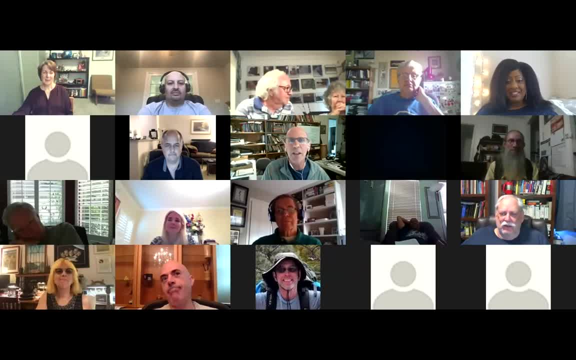 Any takers? Don't be shy, Bueller anyone. I'll go first. 1975 in a six-inch telescope. It was a gray cloud. Yeah, it was Anybody else? I was going to say a two and a half inch telescope, probably in the mid-80s and looked like a smudge. 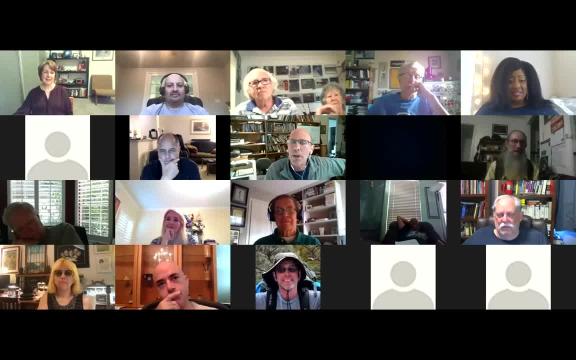 Yeah, it looked like a smudge. Thanks for those answers, Bill. was that your telescope You were looking through or somebody else's? Oh, I didn't have one yet. My brother's telescope, yeah, Six-inch reflector. 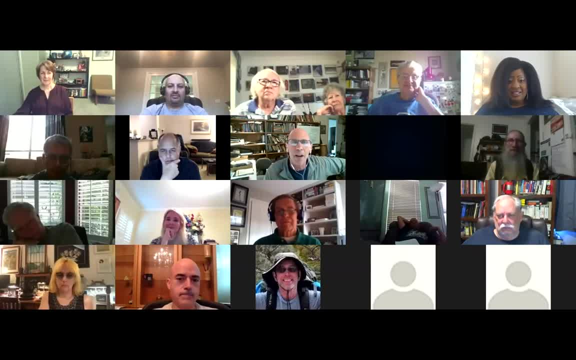 Good, And these guys aren't shills for me, but my story is the same And the reason I wanted to bring this up is because I was at a star party in Denver. It was just before Shoemaker-Levy 9.. That's how I got into all this And they had these things out there on the observing field. 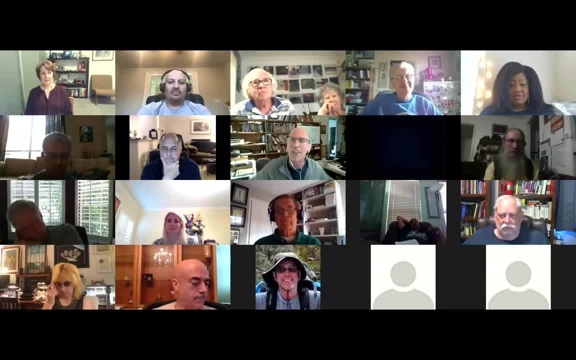 that looked like the cannons in the circus that they shoot people out of. Yeah, They were Dobbs, But what did I know? I didn't know what I was looking at, right? And the reason I like this live video and not to make anybody self-conscious. 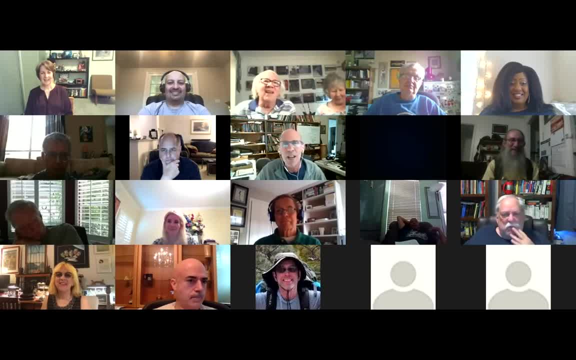 is. I got a laugh there from the Goldbergs, so I think I'm on track then. So when I got up to the telescope there were people like all of us showing different objects, And everybody, all the narrators were excited And I got up and I 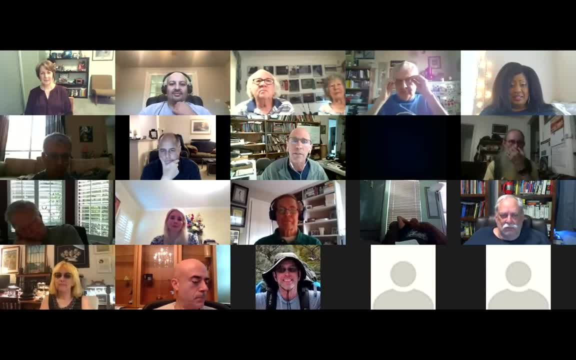 looked through and I would use that word myself: It was a smudge. I was really disappointed And I dare say that most of you have a similar experience. But here's the deal. I bet Bill and Joe and most of you still go back and look at M42, right. 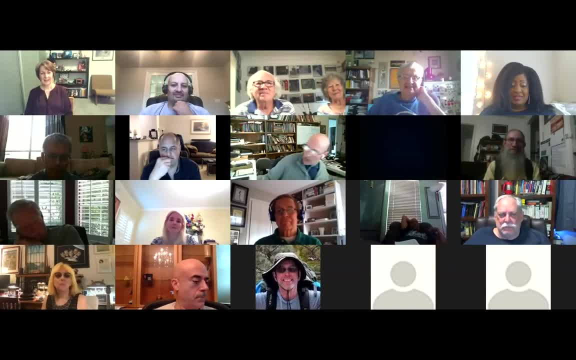 And one of the reasons you do that is because you're much better at averted vision And I had a visual aid here which seems to have disappeared, So it's a stupid one anyway, so we'll skip it for now. But you also go back because you know what you're looking at now And when we bring that. 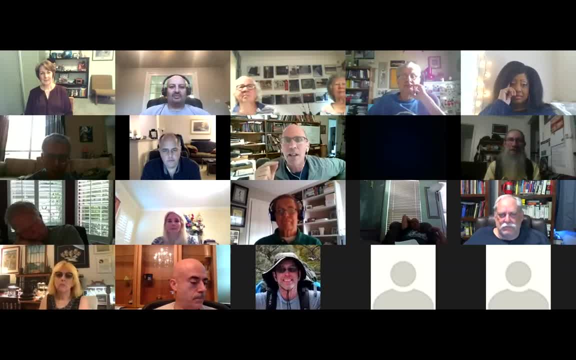 understanding that we've gained over the years to the eyepiece. our experience, as you've seen, you all know gets that much richer. So right now we know M42, for those of you who aren't familiar with it, it's a stellar nursery. There's gaseous clouds and they're glowing and stars are being. 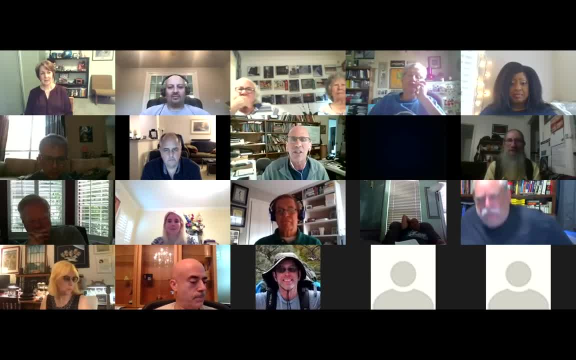 born And it really captures the imagination for us nerds. So the reason I bring that up is because spectroscopy has done the same thing for me is, as I've read about the different objects I've captured spectra of, I've learned more, And that learning I've learned more about the 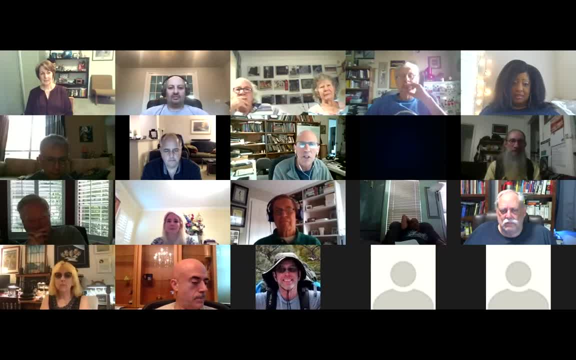 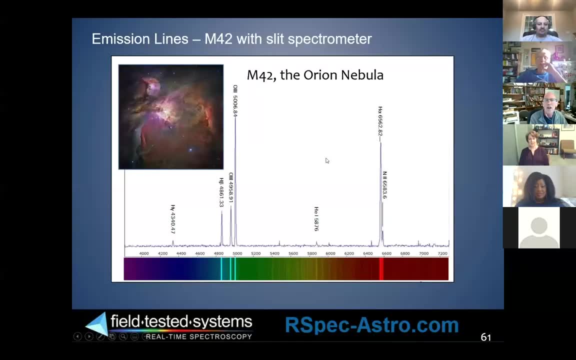 planet And I've learned about the universe, And so I think storytelling has deepened my visual experience as well as my imaging experience. So let me go back to the little show here. Give me a second Great, Okay. So let's move on. look at some other examples. This was also done by that guy. 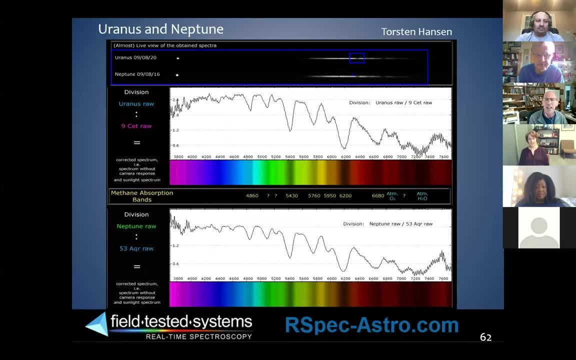 with the imaging source camera. it's Uranus and Neptune. Notice the bands there and notice the deep dips here and the bands visually. This is the methane gas on these planets. This is remarkable. It's a really remarkable example And it's interesting because you can see these planets. 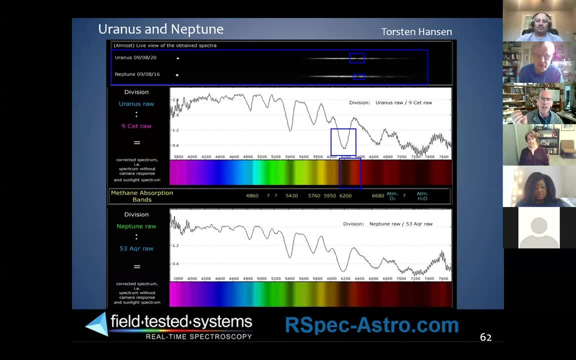 And it's interesting because you can see these planets, And it's interesting because you can see on a backyard video camera telescope. so think of astronomers 30 or 40 years ago if you told them, with an 8-inch telescope you could get this kind of. 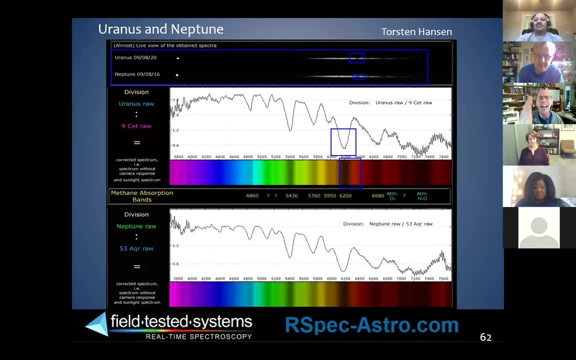 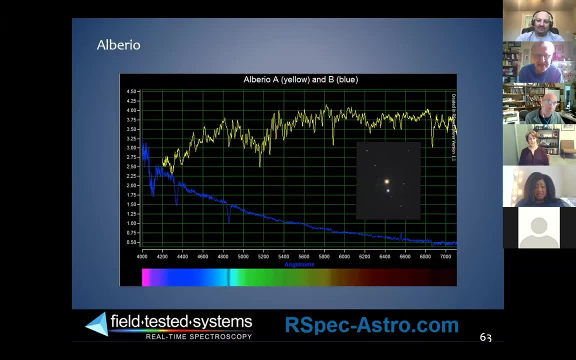 spectrum, they would have given their left a leg right to be able to do this thing. so another example, the kind of thing you can do. so here again, our beloved showpiece Brio, a beer, a beer, you know, our, that's what we're getting back to the space shuttle there, or a Brio I want. all I want to show in this slide is: 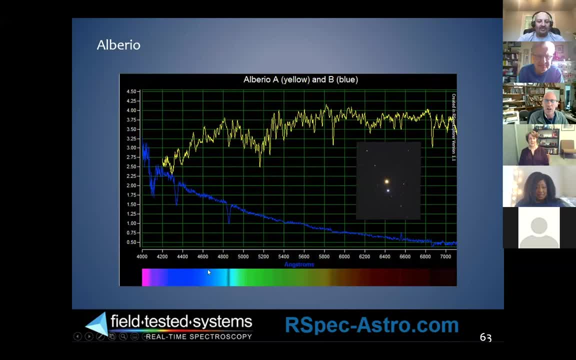 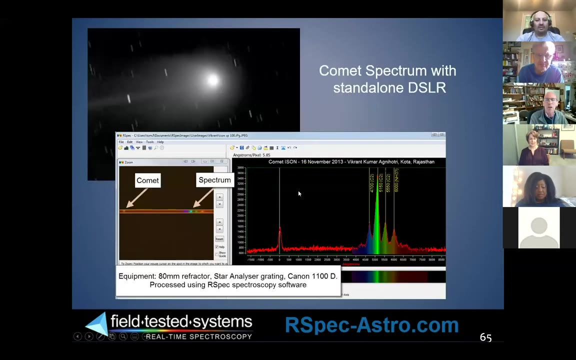 that you can see that the hotter star has more energy over in the blue end of the spectrum. so this is that intensity plot that we looked at my software creating, and in the late 1800s Henry Draper captured the spectrum of a comet. well, if Hank can do it, so can we. so here's a really nice string of jeweled. 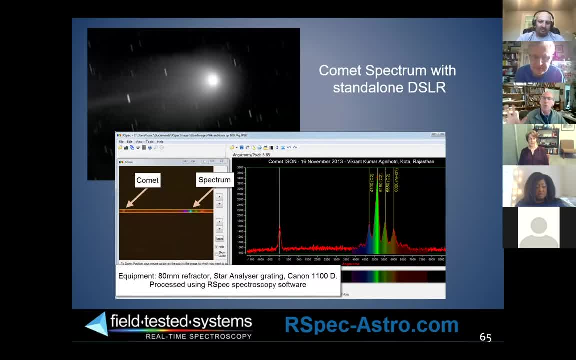 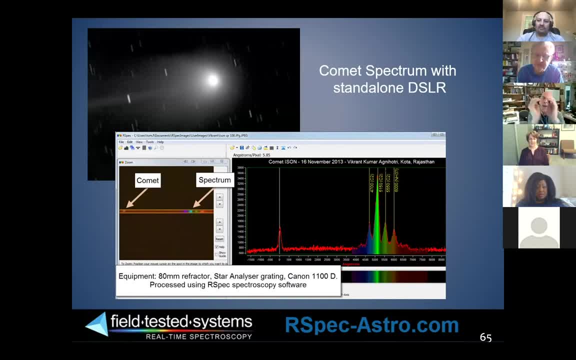 look at extended objects with a slitless grating. but this is a compact enough object that you can. so some comments you can, some you can't. over here we can see the carbon swan bands. this was captured by a guy, Vikrant Agnihotri. he's a nuclear. 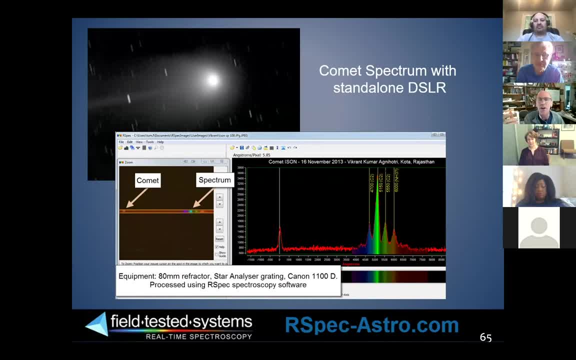 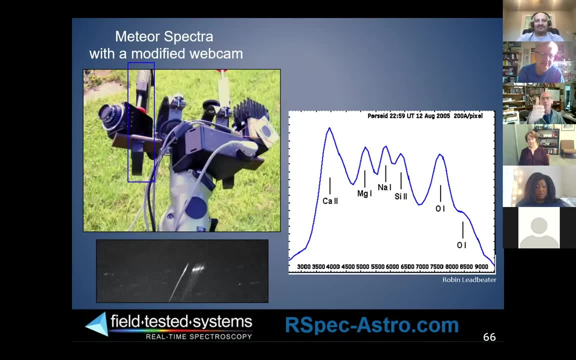 power plant engineer in Rajasthan, in the northeast part of India. it's a great imager today. so now anybody who uses a c-clamp as part of their step is my kind of do-it-yourself. or, of course, I would tighten mine too hard and the enclosure would pop open. 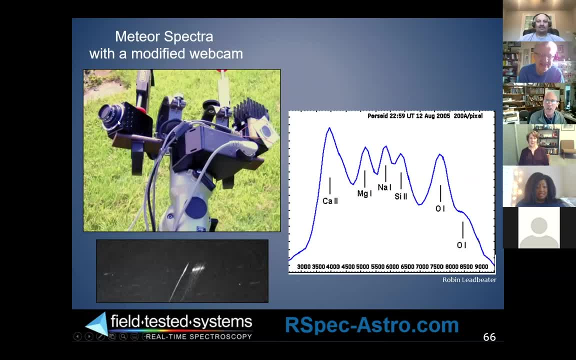 probably, and you can see the star analyzer on this video camera and down here we have our spectrum. it's one frame from a video. the meteor was traveling that far in one frame and at this moment there was a bolide. it got bright and he captured this spectrum and identified some of the minerals in in that spectrum. 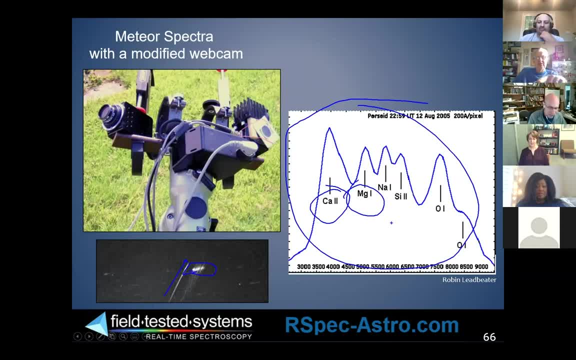 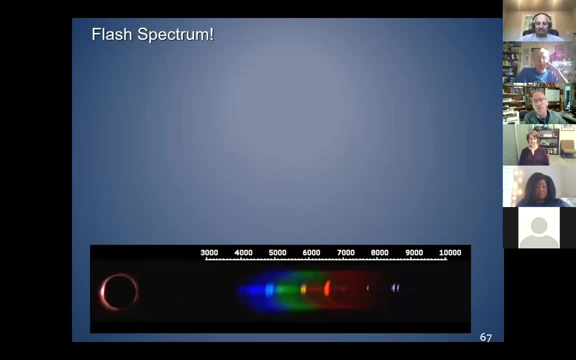 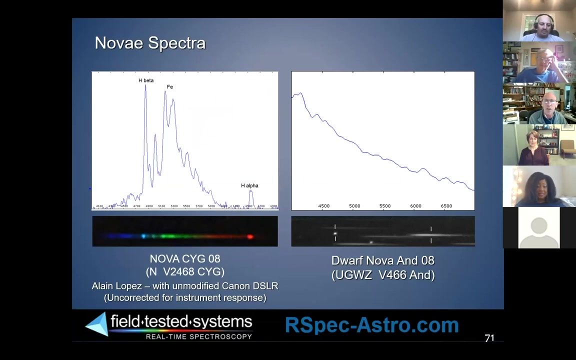 pretty cool. this is a subset. this is even more challenging than some of the other hard things people do, but for some people in the 21st century it's a fairly� eh discovered. so you can capture the specter of uh of nova and notice this nova has some iron in it. 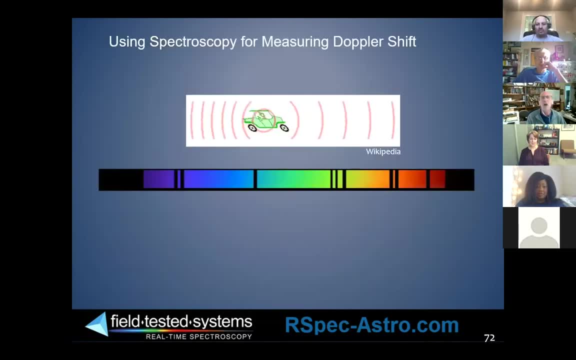 and this one doesn't. so there's science going on there. so doppler shift: you know i'm really sort of bummed out by that, that missing um prop. so during the q a i'll get up and find it. but um just to review, for those of you aren't familiar with doppler shift, which um 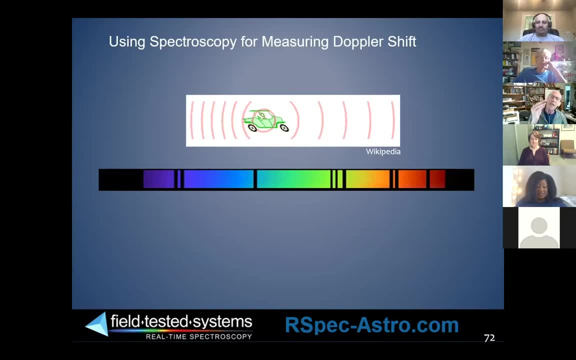 is similar or is it is a name for the change in pitch that a car horn or a train horn coming towards you goes through as it goes past you, so it's high pitch this is coming towards you and as it's low pitches is going away, it actually changes in pitch by that movement. 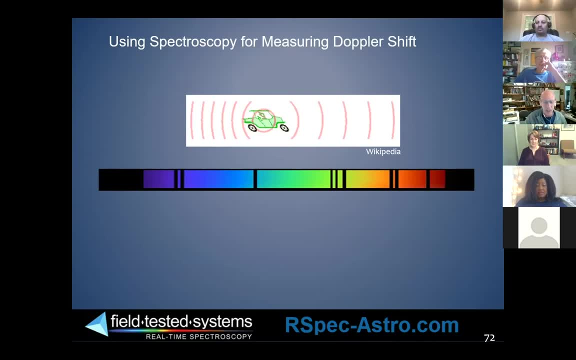 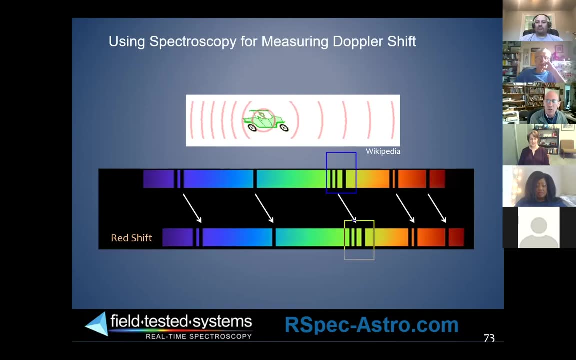 and so, whether it's sound or light, we get the same thing. so if something is moving away from us, we'd expect the spectra to be here, but it's shifted over to the right. we have redshift in the spectra, and so that's what's happening. 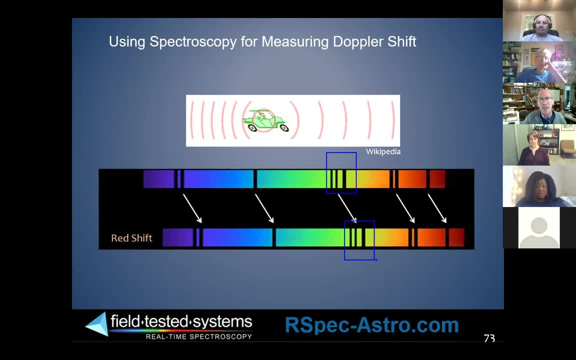 and that's how the first exoplanet was discovered in france. they looked at this, the spectra over time of a particular star, and they saw the spectrum going back and forth over a period of time. and how does that happen? the way that happens? i i could use a good um, a good prop here too. 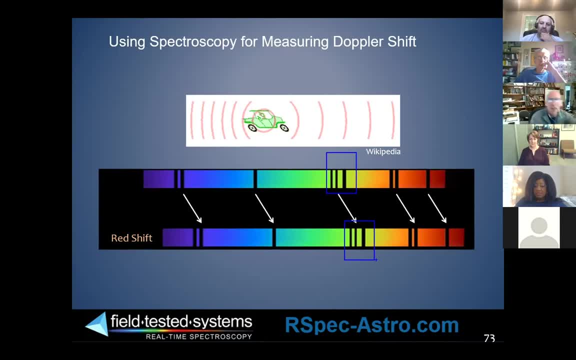 if this is a star, and this is the planet, the exoplanet, and the exoplanet is going around, like the exoplanet, even though it's tiny, is dragging the star towards you, away from you, towards you, away from you. and guess what that gives you? doppler shift, red shift, blue shift. so these 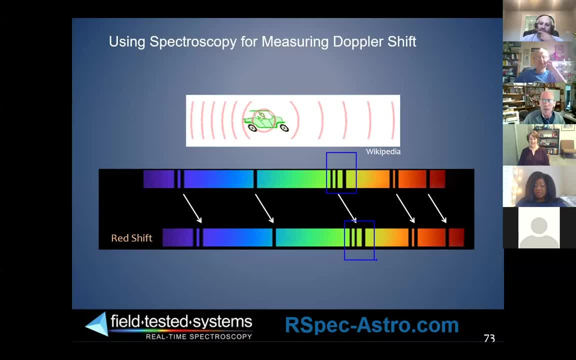 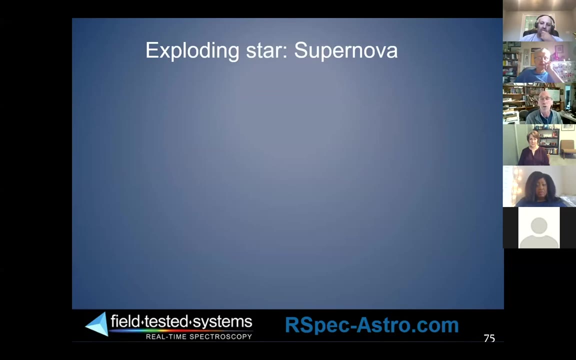 days, amateurs can detect planets using uh photometric measurements. uh, the amount of shift that occurs is very small on objects in our solar system or even in our galaxy. however, there are some objects- that's not the case for um- that are moving fast enough. we haven't had any supernovae. 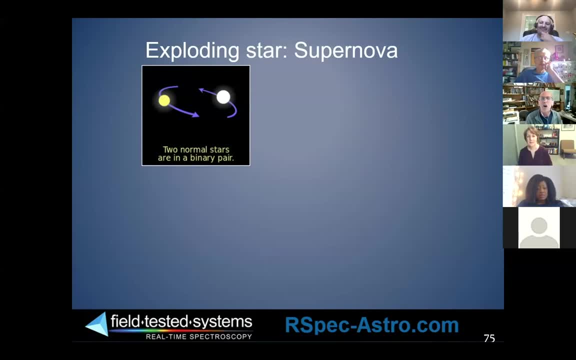 uh, catching our imagination. we were hoping so. uh, supernova, just very briefly, and again i apologize to those of you who know far more about this and could explain it better, or know far more and don't want to hear yet another explanation. two stars orbiting each other. we won't get into the details. 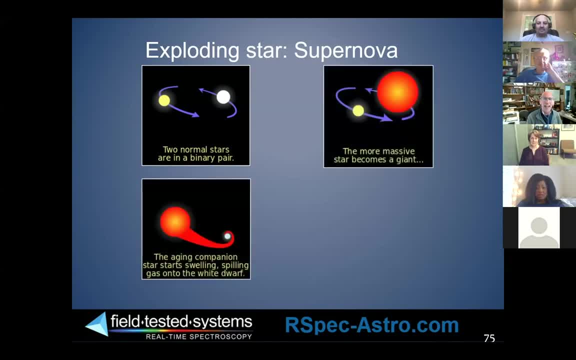 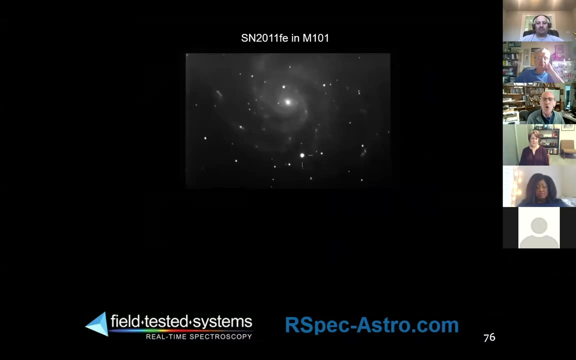 except one of the stars becomes a giant and has a lot of spare gas, as if, and some of its gas spills or is gravitationally attracted to the small star, and when you think that you're going to throw gas on something hot, it explodes and you get a supernova, supernova. 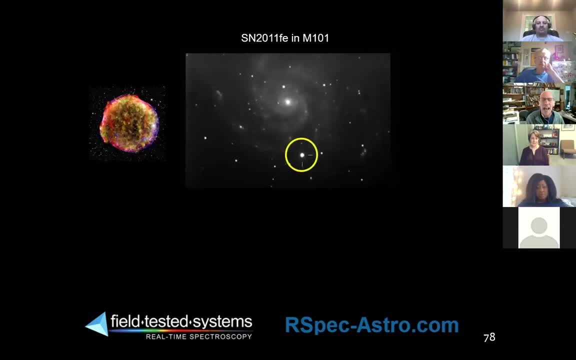 enormously bright. there's one in m101 and there's what a supernova of this type looks like. it's not this supernova and that's the expanding cloud. i love that image because you really we recognize that as likely to be a sphere that's um spherical as most spheres are, so there's a spectrum and 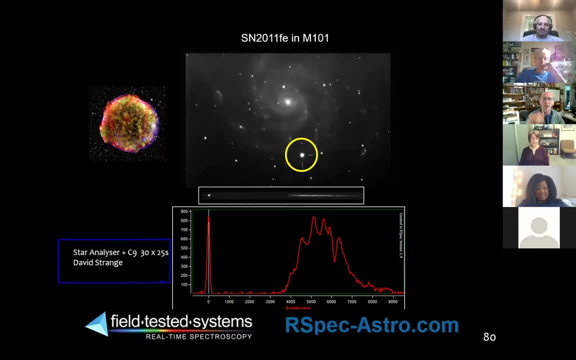 there's um david strange's equipment which i want to point out: nine inch celestron telescope star analyzer grading and less than 15 minutes of integration time. when he uh looks at this spectrum, he found a little absorption feature right there and when you look at it in the software, it's there now the shoulders upon which we're standing and the heads. 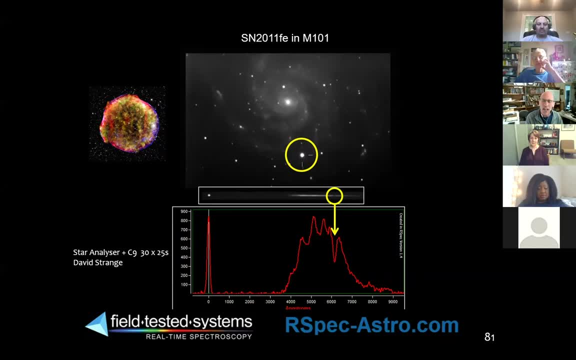 that are on those shoulders have figured out that type 1a supernovae, where you have these two stars, one dumping gas onto the other, occur. you get a very deep dip from silicon and that dip, david, measured on the x-axis at 61.50. now bear with me four lines of. 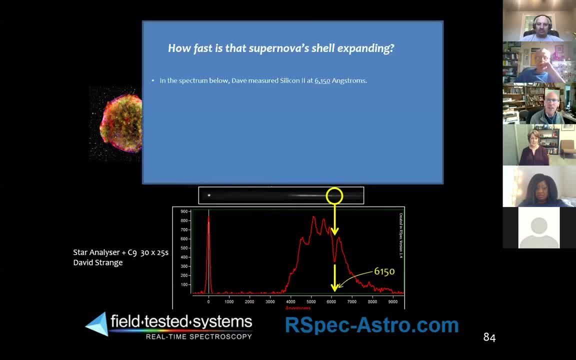 math, nothing fancy. there's the number that david strange measured down in the x-axis right: 61.50. so there's this. there's where the dip would be if bunsen burnt silicon like beach sand. those numbers are different, so we have some doppler shift. when david sent me this spectrum, i went to wikipedia. 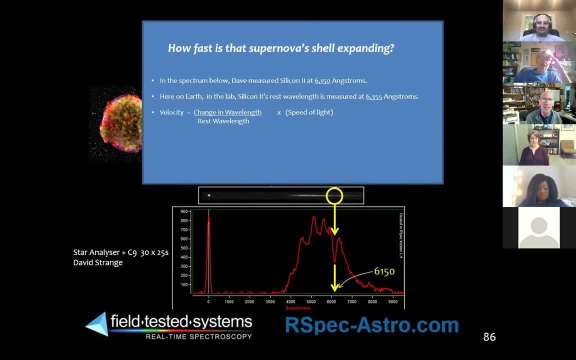 didn't know the doppler shift formula by heart. maybe i did 40 years ago. i doubt it. and there the numbers plugged in and there's the result, that's blue shift from the shell coming towards us at 22 million miles per hour, measured on a nine inch telescope in the backyard. in less. 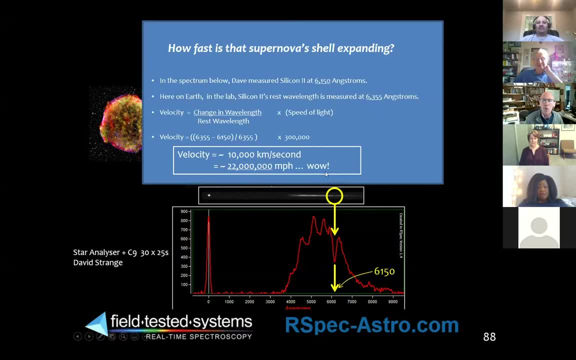 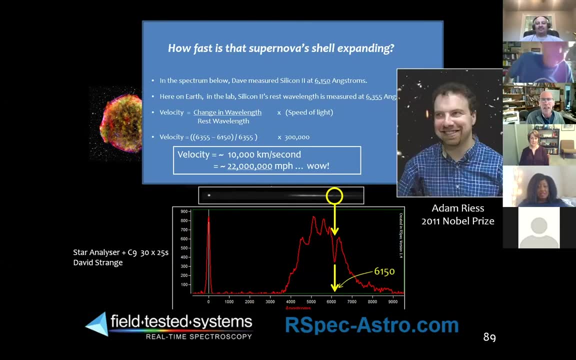 than 15 minutes. there should be two wows here. one is wow, that's fast. the second is wow, i can't believe i measured a spectrum, uh, with such simple equipment. now, some of you are familiar with adam reese, who won the nobel prize in 2011 for work he and his team did just before the turn of the 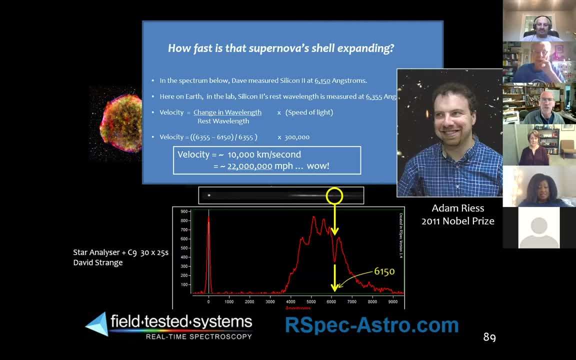 century. i wonder whether this feels like you're drinking from a fire hose here, and whether that's good or bad. this is being recorded, you can go back to it, and i'm going to also give my email address at the end. so, uh, so i love the topic, as you can tell, so don't worry if you're missing things. we. 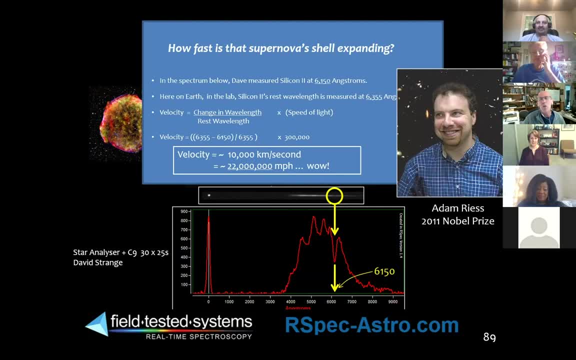 can have a chat about it afterwards or at some other time. so he won the nobel prize, as many of you know, for a measuring cosmological expansion of a solution to the expansion of space. the reason: expansion speeding up, And he used these type 1a supernovae as his standard candles. 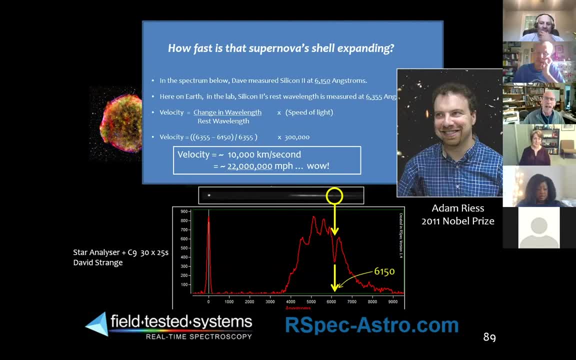 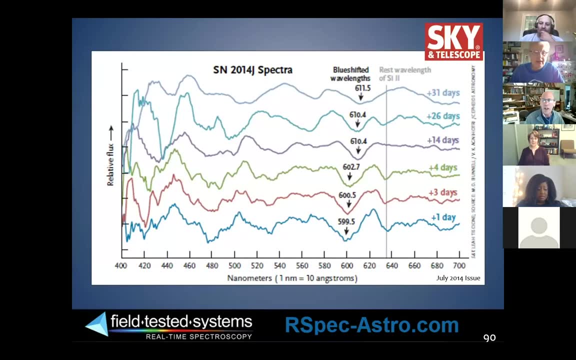 And we've just measured a supernova and its radial velocity of its shell anyway, on backyard equipment. So here's another quick example. These are plots, day by day, of a supernova. There's the same dip we were looking at of ionized silicon. You can see as the days go by. 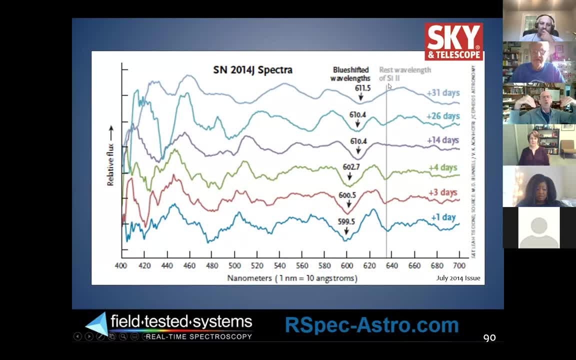 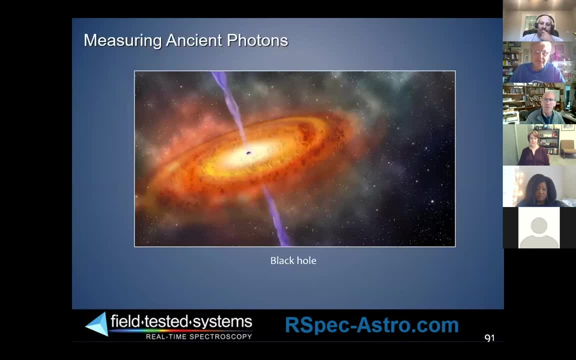 it shifts back to its resting wavelength and it gets more flat because the shell is thinning out, And so we are able to see through it to the start. So this is a black hole. We're not going to get into a lot of theoretical discussion about black holes, except they can be enormously bright. 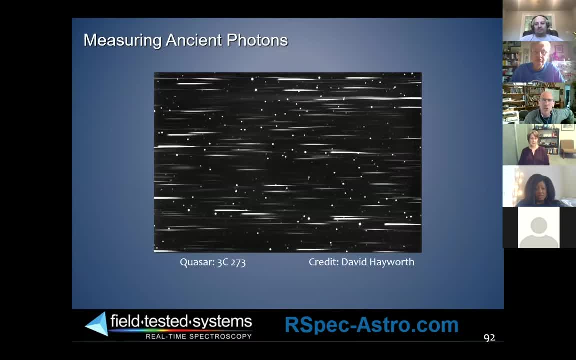 An example of that is a black hole 3C273.. These were named as quasars in their original naming Because they were quasi-stellar objects. We didn't know exactly what they were. David Hayworth captured this image with a similar exposure time, about 15 minutes integration. 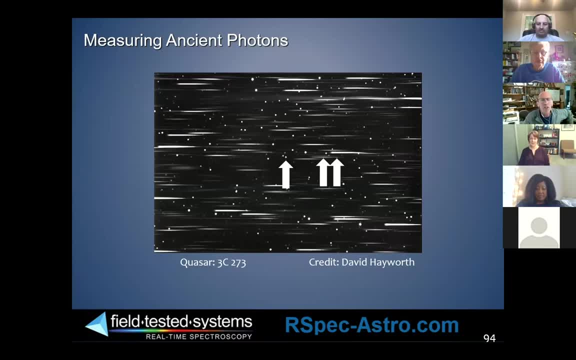 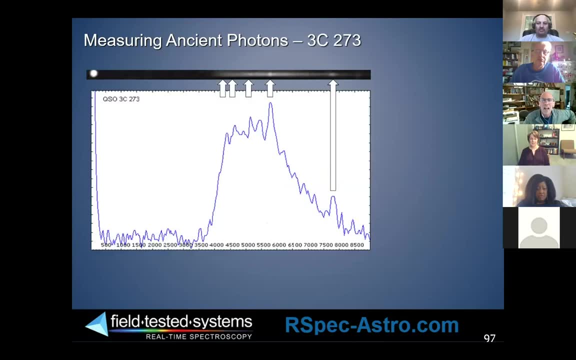 There it is. I've never seen 3C273 myself or its spectrum. You can see the two dots where those arrows are pointing and there they are blown up. When we plot it, we get that plot, And this guy who was 25 years old or in his mid-20s, and the 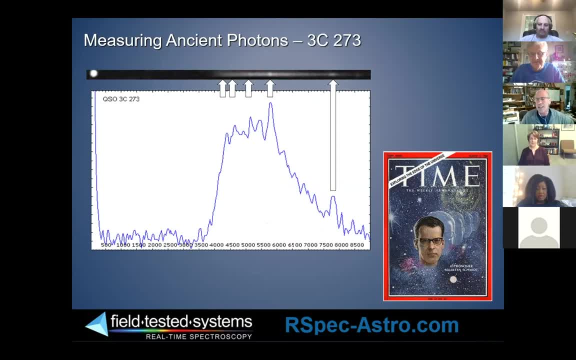 same age as me, stared at this And there's a fantastically interesting transcript of an interview of his, the link to which is on our site, but I can also send you. I think you'd enjoy reading it. I don't know any easier way to deliver it to you. I guess I could have a tiny. 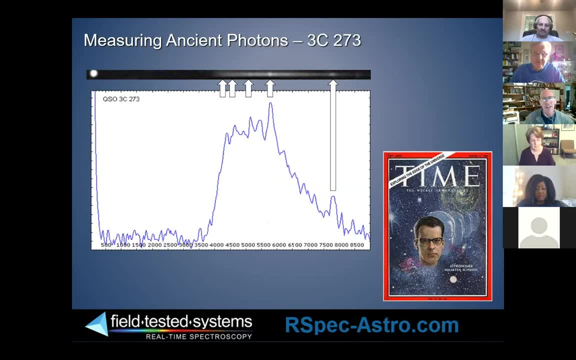 URL here with it on it. But he describes staring at this and the science and how science works. First of all, lots of frustration. Can't figure out what it is. Can't figure out what it is, Decides after pulling his hair out. that well, at least you know. let's just. 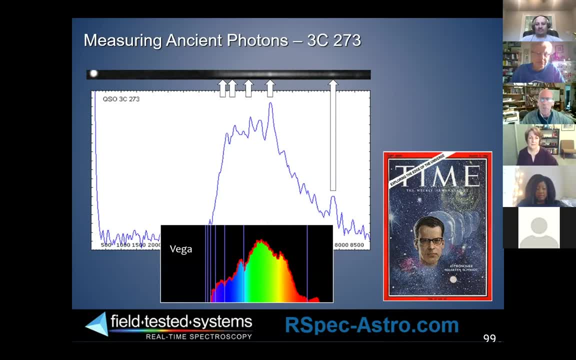 eliminate, it being hydrogen lines. So he pulls up a spectrum much like the one I just showed you. In fact, this is the one I just showed you in my software. I forgot. I wanted you to look at it and remember it. And he went. well, no, those don't match. except they do match, but they're shifted. 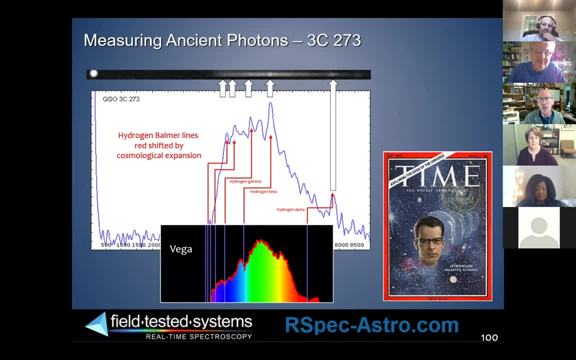 way to the right. There's a lot of Doppler shift going on here, And this shift is from cosmological expansion. In fact, when I wrote my first article for Sky and Telescope 2011,, I called this redshift, And the editor-in-chief of Sky and Telescope, Bob Noye, 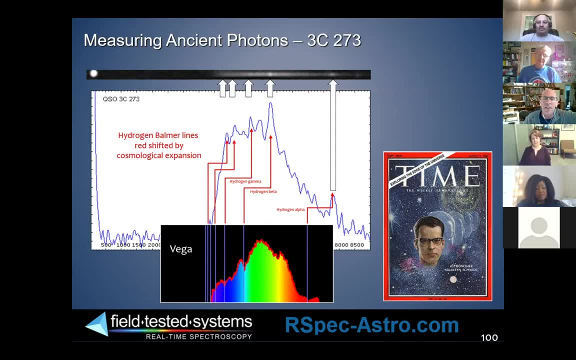 sent an email to Reese, the Nobel Prize winner I mentioned in the previous set. He hadn't won his Nobel Prize yet And I asked him. he said now Tom wants to call this redshift or Doppler shift. Is this Doppler shift, from speed, from velocity? He said no. 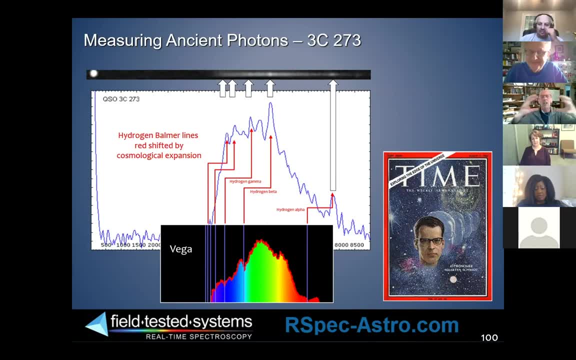 there's nothing moving here. There's cosmological expansion going on. It's an interesting distinction, a subtle distinction- the way words work and the way scientists use words to be clear about what they're talking about, So we can measure the cosmological shift. 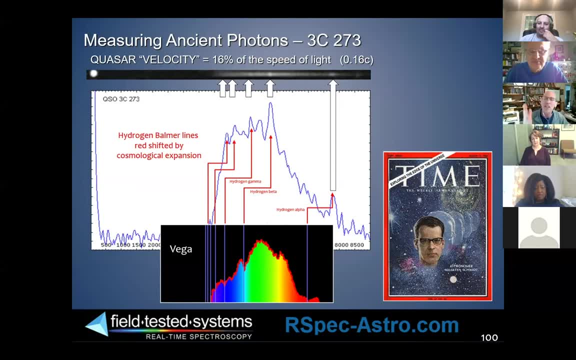 of this quasar with a backyard telescope. The amazing thing to me is- and what this discovery was, by the way- was that this object was so far away- 2 billion light years away- but still bright enough that we could see it, which meant it was enormously bright. That was the discovery. 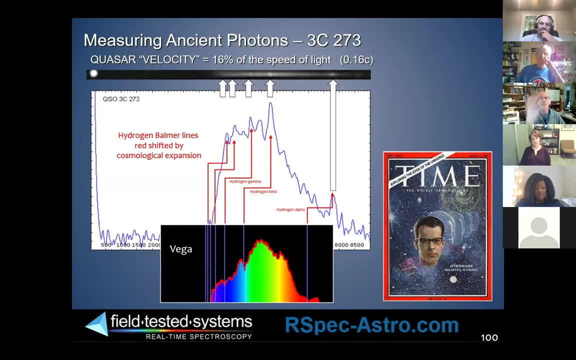 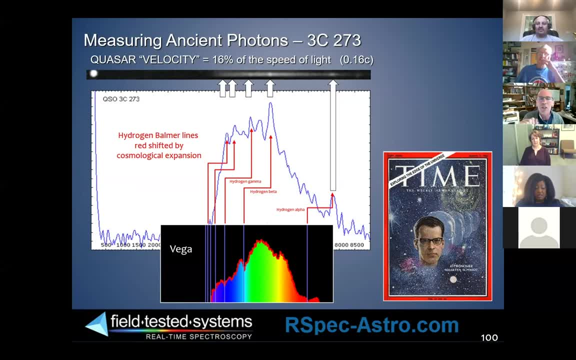 are when we go out on a limb with something that's new and novel. He was scared And he talks about in this interview. he was worried he was going to be laughed out of the academy because he made a stupid mistake And there was an easier way to explain this, But he published it anyway. 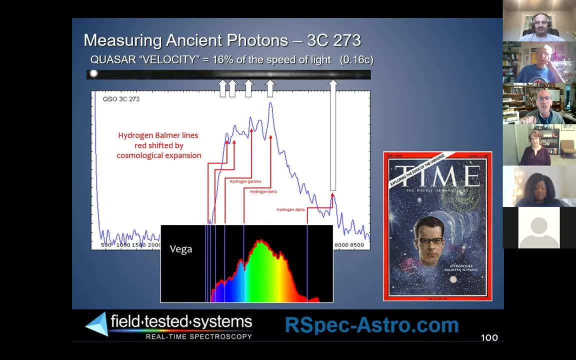 after conferring with him, some colleagues who agreed with him that this was the right interpretation. 2 billion year old light that still has enough information in it that you can understand something. And I can't understand anything about the original object and how it got here. That's amazing to me. 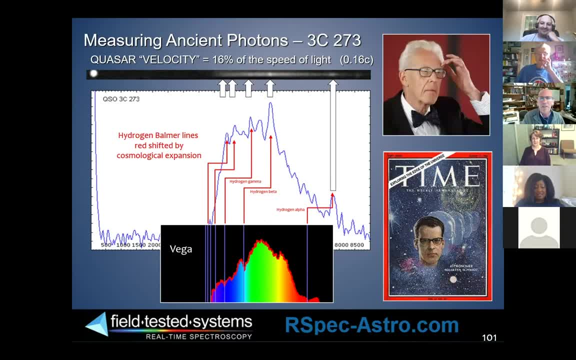 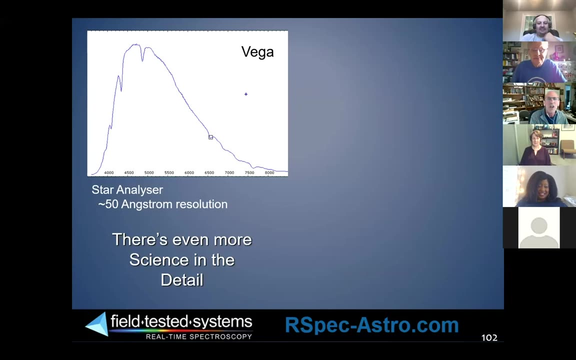 There are other things in the universe that do not age as well. Here's Martin Schmidt, a few years ago. Now I live in a glass house, so I shouldn't be throwing stones, I know, But it is remarkable what can be discovered with such ancient light. Now, so far. we're just about to wrap up here my presentation. 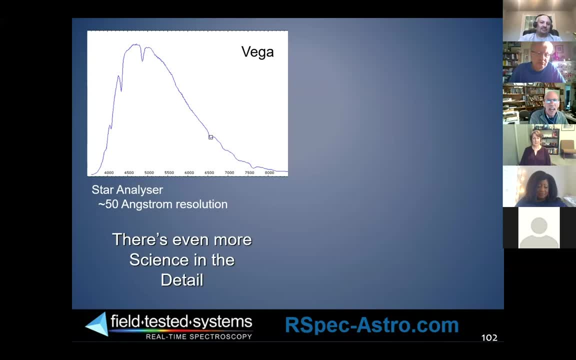 So far we've been looking at features like these, the hydrogen bomber lines. If we wide are those lines. Let's just take a look here. Let me bring up my pointer here. So if we drag down to there and to there, what's the width of that? It's about 50 angstroms. But if we want to, 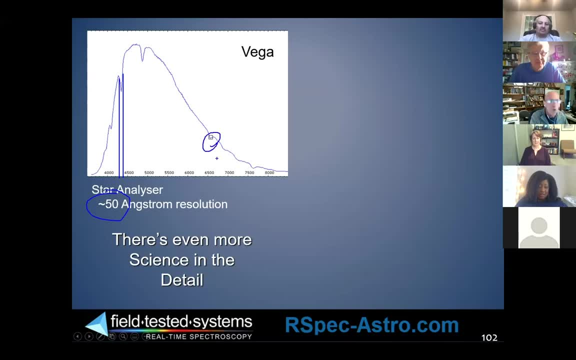 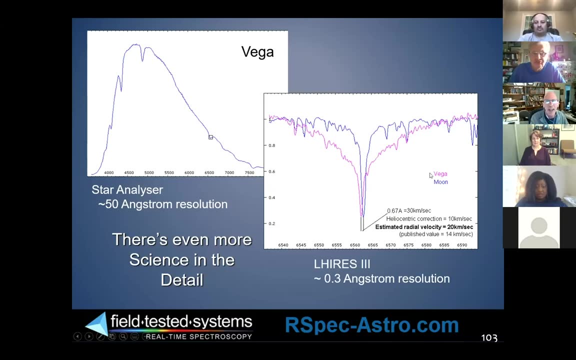 drill down into the details of one of these, zoom in. we need a lot higher resolution, And that's where you end up using a slit spectrometer. And here we have two spectra, one of Vega and the moon, And you can see this major dip, this hydrogen alpha dip, is in different positions. 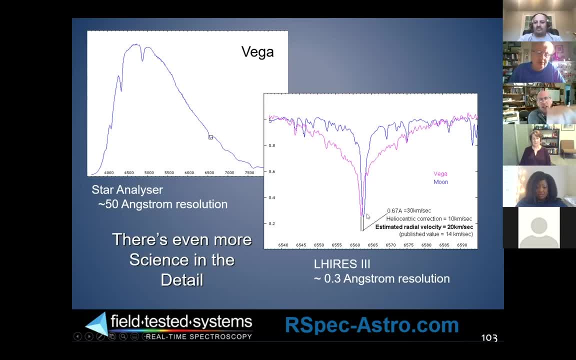 Because Vega is moving towards us, blue shift and the moon really isn't. So we compare a known stationary object to an unknown moving object And now we can measure again the radial velocity. And that's another way that we can. well, as I mentioned earlier, we can detect the exoplanet. 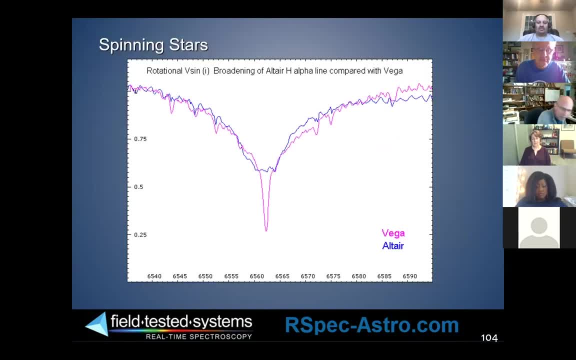 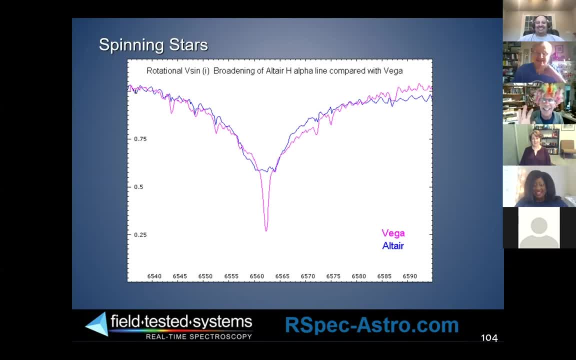 spectroscopy talk. They tell you to dress for success, And that's their hydrogen beta line, right there, I think, And then the gamma. So anyway, now I have a little problem here. I know it's here somewhere. I had, like you know, I haven't been able to get to my stylus in like 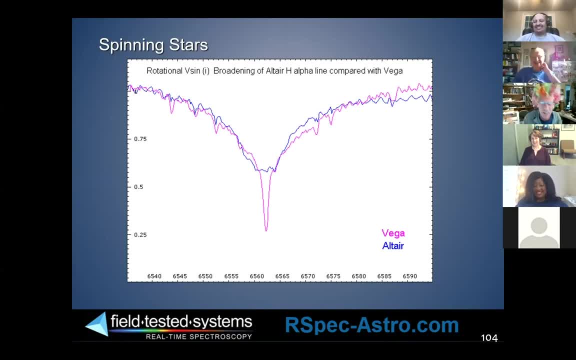 months. You know they're, just they're not. none of them are answering their phones. I don't understand, So forgive me for the look. So over here I have a star And that star is rotating. So the light coming off the star here is coming towards you as it comes off the star a little. 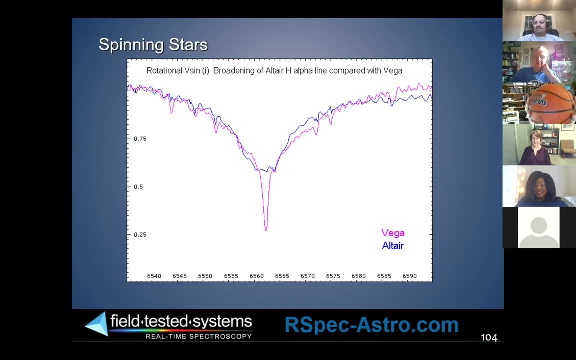 faster, a little sped up, as if, And the light over here as the star rotates is a little slowed down right, Because the star is rotating away from you. So you have a smearing. What would normally be a very deep dip here is spread out and smeared on. let's see which is that: Altair. 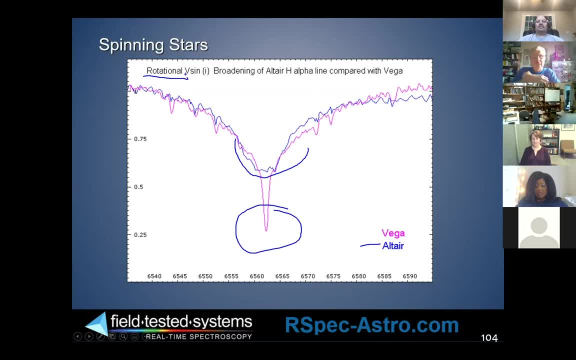 So now we're measuring the rotational speed of a star. This also requires a slip to get that kind of resolution, but it's pretty cool that you can do it Okay. So how do you get started? Very simple. I've talked about the star analyzer grading here. 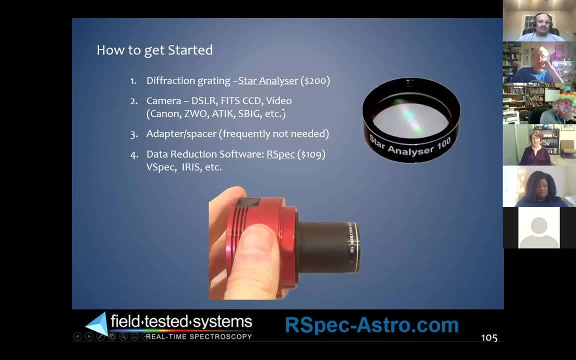 You need almost any camera. It's not as important as focus, but this distance from the grading to the sensor in the enclosure of your camera needs to be in a certain range, And so you may need a spacer number three there, And there's a little bit of space there, So you need a little bit of. 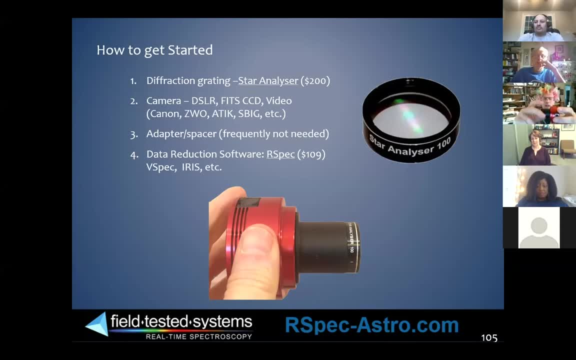 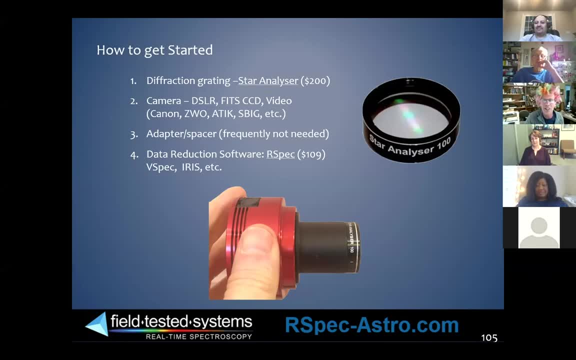 would work with their equipment. You know, in the UK somebody was recently telling me they don't call them speed bumps, They call them sleeping policemen. So it's funny how different cultures have different expressions like that. And finally, you need software, My software, which I showed you. 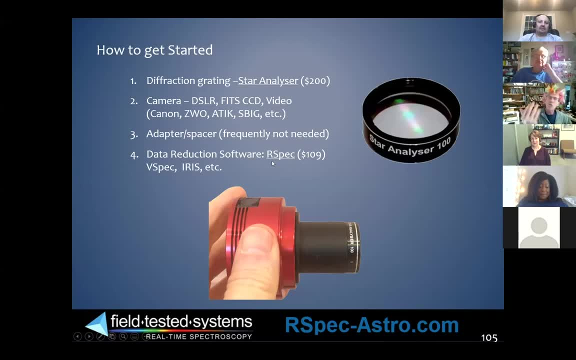 RSpec stands for real-time spectroscopy. because you can do real-time video. You can also have, as I mentioned, FITS images or raw DSLR images automatically loaded into the software as they hit your hard disk. So there's lots of. 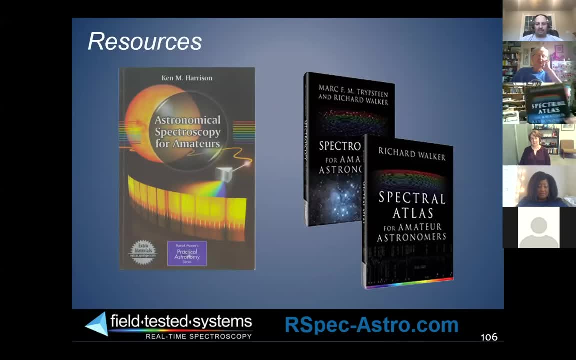 resources. The one I just wanted to flash in front of you- and they're all listed on the site- is this, And the cool thing about this is because I mean it. as I said earlier, I was worried. well, I understand what I'm looking at. How do I interpret it? So this book is great. 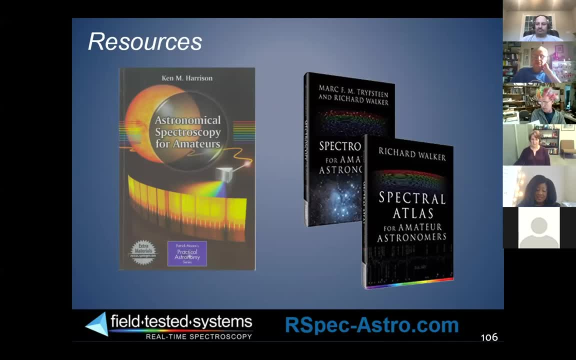 because it's got. let's find a great example. Let's find one here. It's got sample spectra with various things called out in them and which are worthless to most of us, including me, because I don't know what I'm looking at. It's got the pros to explain what we're looking at. 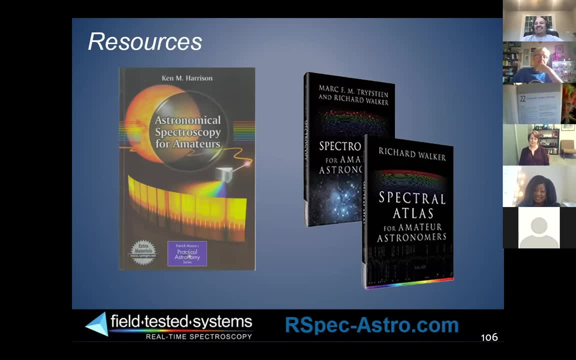 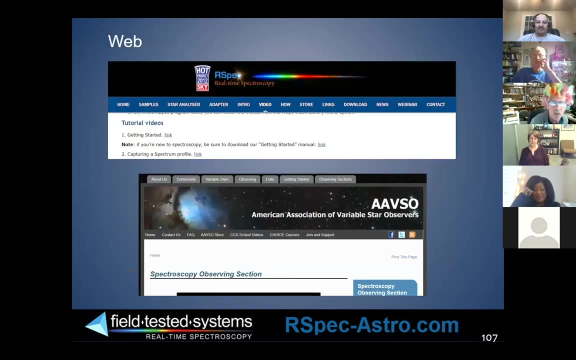 And so even for an armchair philosopher- yes, like that Frenchman who was wrong- even for an armchair astronomer, this is an incredibly valuable book. There are video tutorials for my software on the site. In fact, the software is free for 30 days. 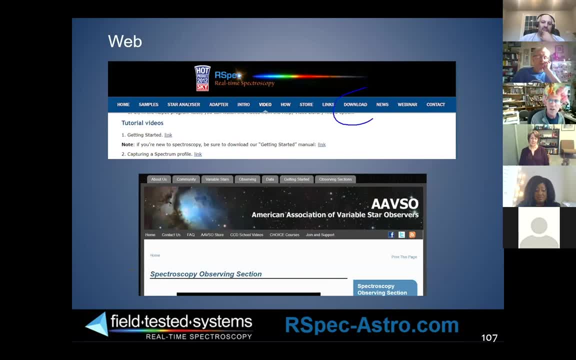 on the same link. It's this one here. on this download link You can download the software As well as a link to a one-hour YouTube video of me giving a workshop in person to the AAVSO a few years ago at the SAS in California. Sample data is there. You can go through all that on your own. 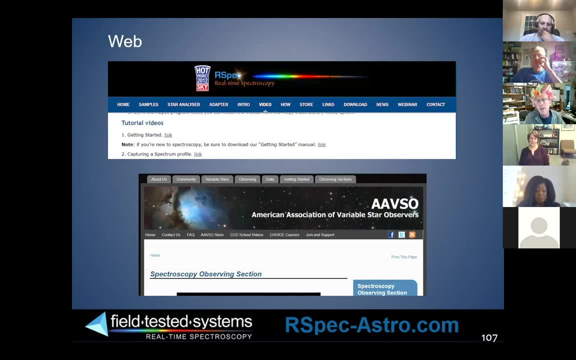 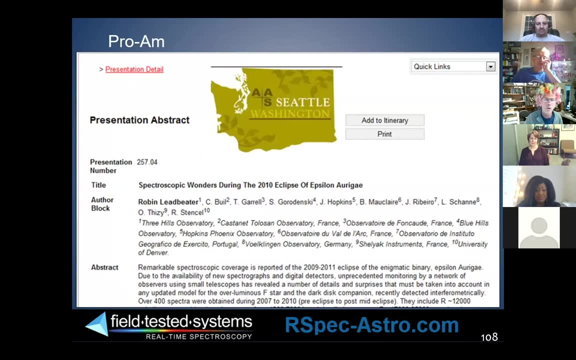 for fun, And there's, as you can see at the bottom, there, the AAVSO has jumped with both feet into spectroscopy. They have their own database for it. now, too, There are opportunities to do pro-am collaboration. Not as many as all of us would like, but there's more and more, and the AAVSO 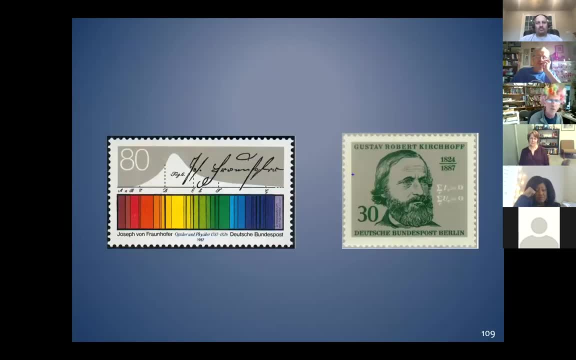 is going to help us get there. So we've come a long way in the last 45 minutes, as well as in the last three centuries. Fraunhofer, you may recall from an earlier slide, discovered a spectra of stars, invented the spectrograph. 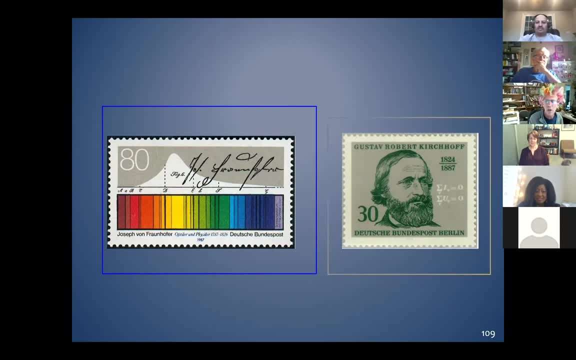 Kirchhoff to the right, was a contemporary of Bunsen's and helped us understand what we were seeing. We do stand on the shoulders of giants And it's amazing the discoveries. I think I might have used that word amazing too many times tonight. The other thing I wanted to mention was I wanted 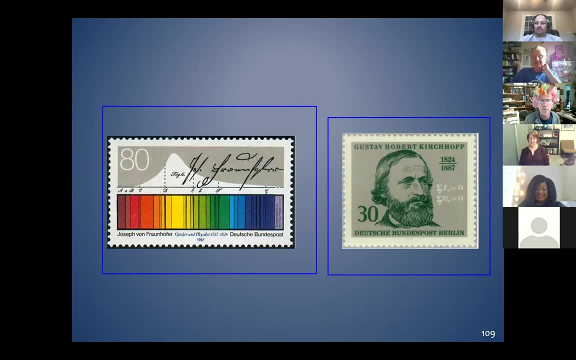 to thank the club Because looking at your site and talking to people about it beforehand over the last several weeks, I know the club and a lot of you do outreach and educational work And in my mind that's one of the most important things we can do, especially because we have the science and we've all had the opportunity in our lives and the privilege to be able to learn what we've learned. 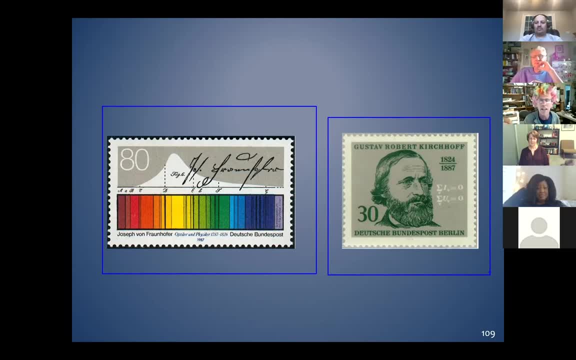 And it's nice to give back. It feels great, as you all know. So I'm mostly singing to the choir, but I wanted to thank you for all that. Thanks for your attention tonight. Thanks for smiling at my jokes. I'll see you next time. Bye-bye. 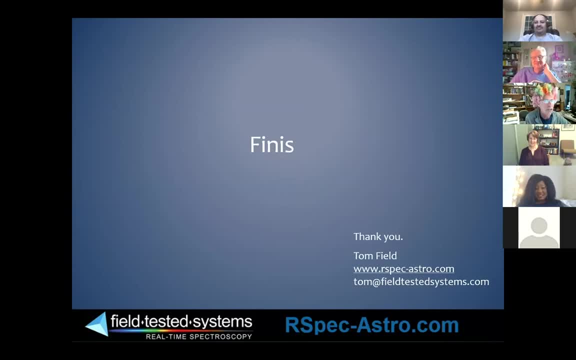 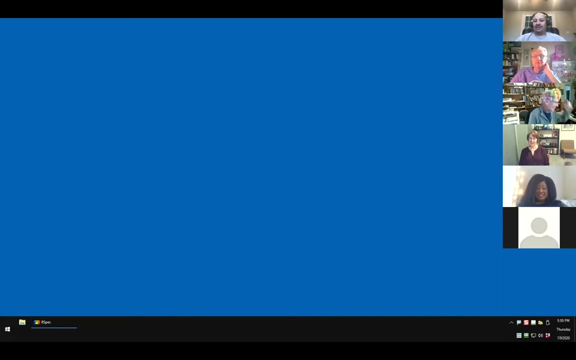 I'm here and I'm happy to answer any questions, Joe, that they chatted or that they may have that they want to say out loud. There's my contact information also. Thank you again. Wonderful Tom. Thank you so much for that presentation. You said you can't use the word amazing enough. I think that was an amazing presentation. I'm ready to go out and start doing this myself. So, if you want folks, go ahead and unmute yourself so we can ask some questions. But we did get some through the chat room that we have. 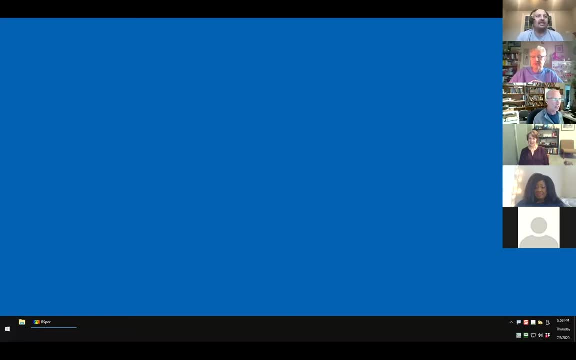 Bill asked first: how can we get some quote inexpensive gas tube type of targets? Yeah, good question. Well, this, here is there. This is, oh, my camera's on a different monitor. This is a gas tube that costs about 30 bucks. The power supply costs a couple hundred. I can give you the names of some suppliers if that's something you want to do. 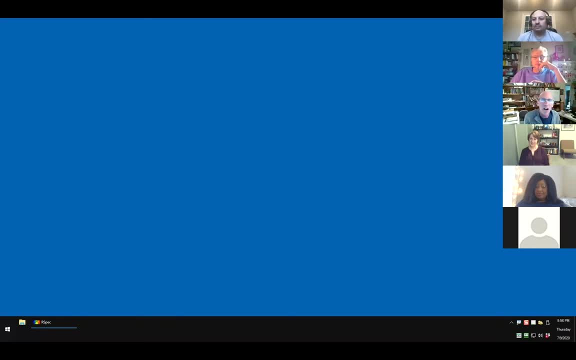 It's not real exciting as an amateur to do a lot of that. After a while They're always the same. You pull them out, But they're and they're not really necessary for us, because we don't need them to help us calibrate our specter- a topic we didn't get much into, Does that? I wonder if that answers your question or whether there was more to it. 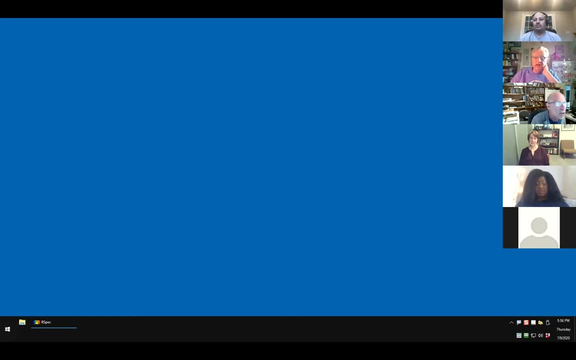 What kind of place would I get gas tubes like that? Oh okay, So the place I recommend is called Arbor Scientific. They're out of Michigan And they're very responsible good people. I've worked their booth at a variety of educational shows. 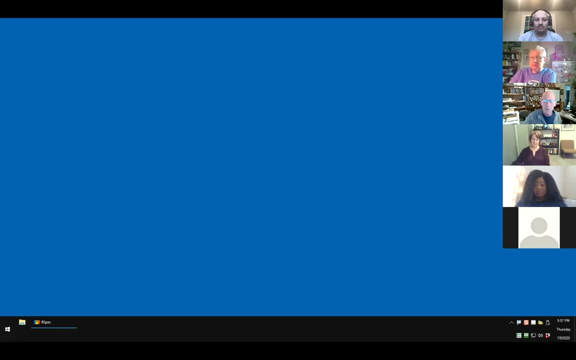 And I can send you a link. if you want to send me an email, I can send you a link to the actual products If you're going to do that. just a just a brief advertisement for this thing that I showed. This allows you to capture spectra on a lab bench. You may want to just do it with a telescope or DSLR, but this just plugs in and has a video camera in it, Same software as the astronomers use. 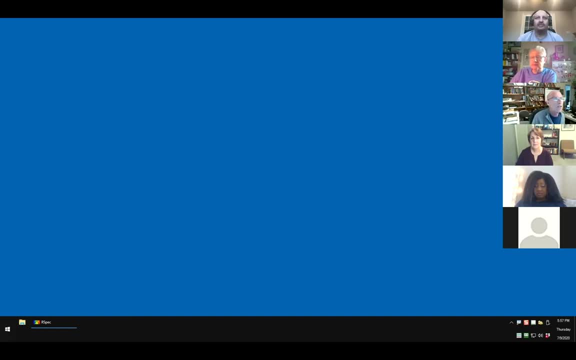 Are you sharing a screen? right now, People are saying they just see a screen. No, a good question. All I'm sharing is the little stamp that they can see. I think All I can see now is a blue screen. Oh, my apologies, Let me stop sharing my screen. I really appreciate your pointing that out. 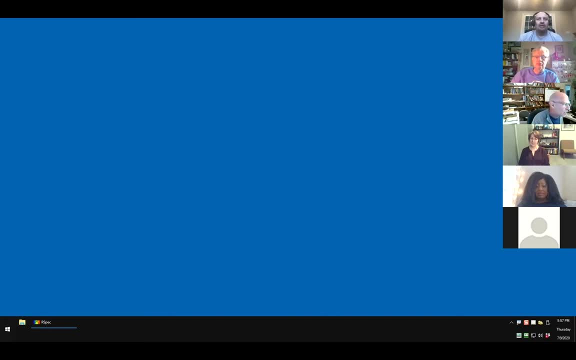 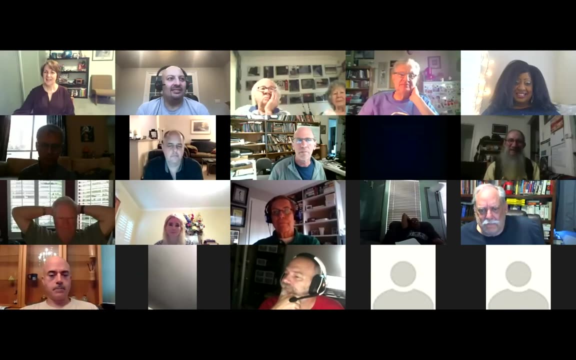 Oh, no problem, If I can find Zoom is so easy Meeting controls. So Justin McCollum asked: is that large red curve correlated, Related to the source's blackbody radiation curve? And I think that was when we were watching the spectra where you showed the first slide of a spectra. 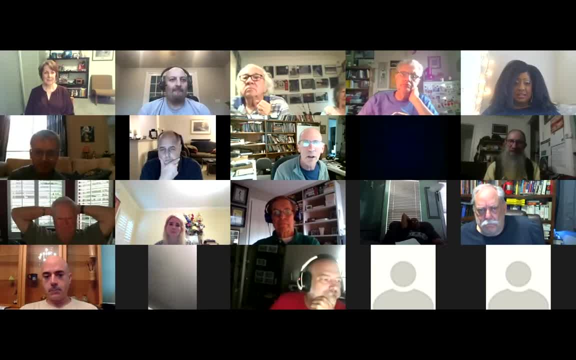 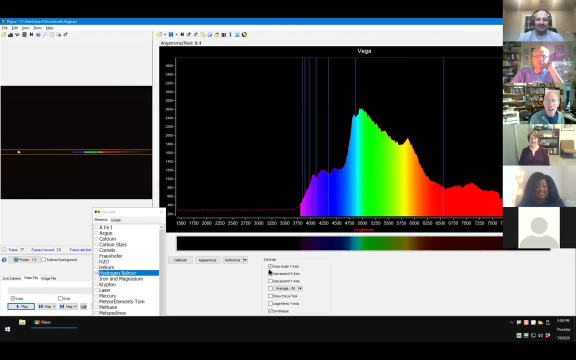 Yeah, a great question, And for that I'm going to share my screen again. Sorry, Just in time, right? Yeah, this happens. So here's what the question is. The question is: stars have a particular shape of their curve depending on their temperature. 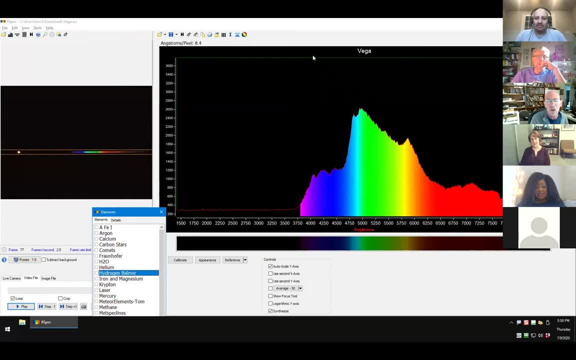 Not only the dips but their shape, And that shape is often called a Planck curve, Even though, in truth, stars are not blackbody radiators And this curve doesn't look like a star's Planck curve would look like. 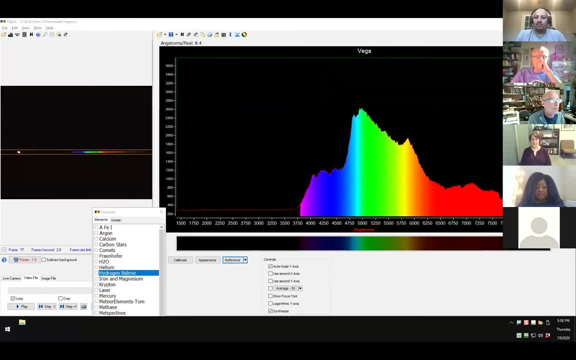 And let's see why it doesn't. Let's see why. So the software has built into it a reference library of all the different stars: O, B, O, phi and G, K, M. There they all are. So let's bring up a type A05 star, because this is Vega. 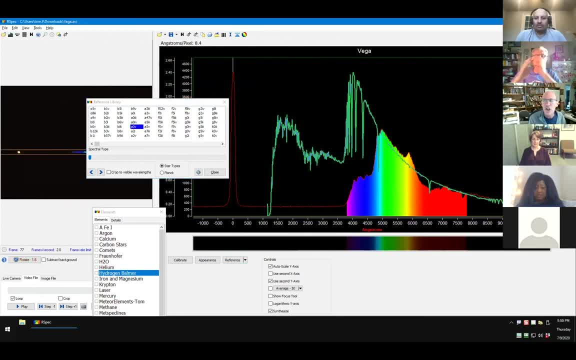 So now in blue, there's what the star should look like, curve wise, and in red or green, now that's what it looks like. So the question is, the question is saying, first of all, does the red curve reflect the blue? 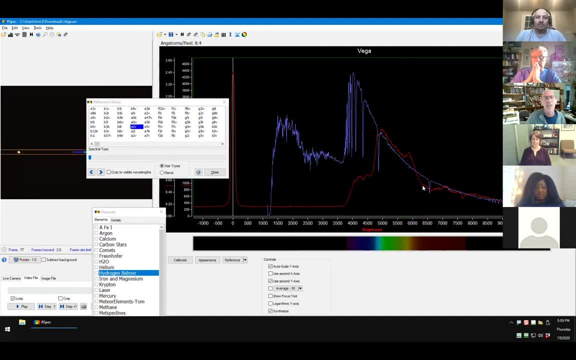 And my answer is no, it doesn't. And the reason it doesn't is an interesting one, And that's because our cameras are more sensitive in the green and lose sensitivity as we move into the blue as well as red, So that's why. 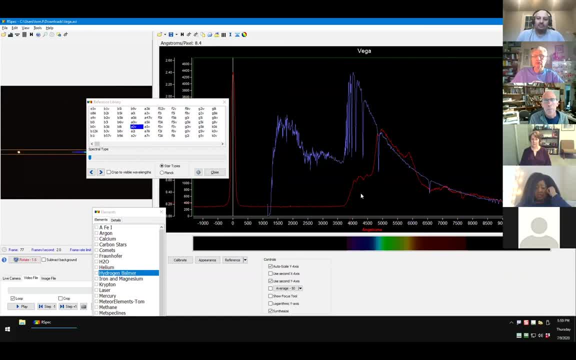 That's why this curve drops down, But the good news is we can correct this curve. This is a curve from a professional who's already corrected it. This is the Planckish curve. By the way, the reason this isn't a Planck curve is because there's all this energy over here you have to accommodate. 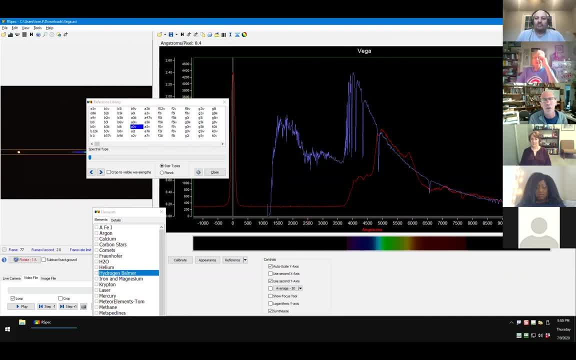 You have to account for if you're going to use wine's law, for those of you who are familiar with that. So the other reason it's not a Planck curve is because the starlight could be coming through some red, reddening dust on its on its travel, coming towards us. 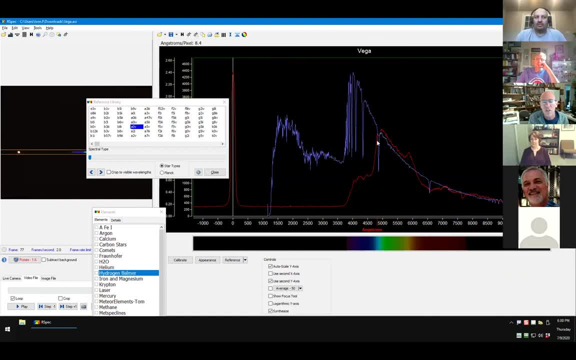 All those are fixable. But so there is a way to correct our curve so that this curve looks like a type A star. And I have just for a second- Let me see if I can find it- A B E R I O. 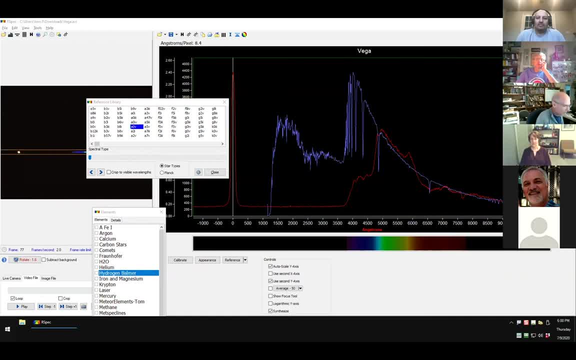 Let me try one more time. A N P something. Here we go. So I'm going to show you a video of Albireo A and B that demonstrates that, And I'll narrate it as we go. It's pretty cool. 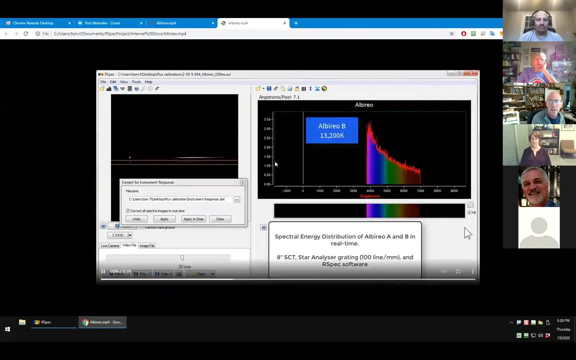 So, if I can get it onto the screen. So here is the corrected spectrum of Albireo, the dimmer of the two, which would be B, And notice it's got more energy because it's been corrected over here in the blue. 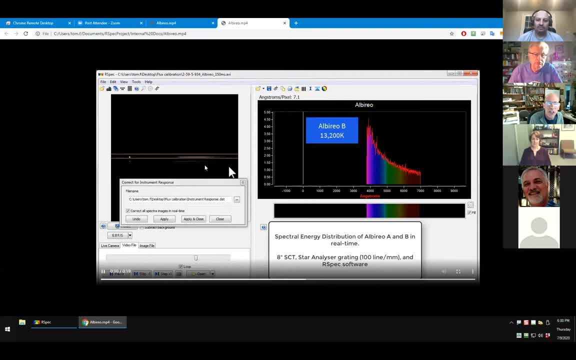 But if we run the video a little longer, I'll move the sampling lines to the other of the two Albireo stars And it's got all of its energy over here, Or not Not all of it, but more of its energy over here, in the red instead of the blue. 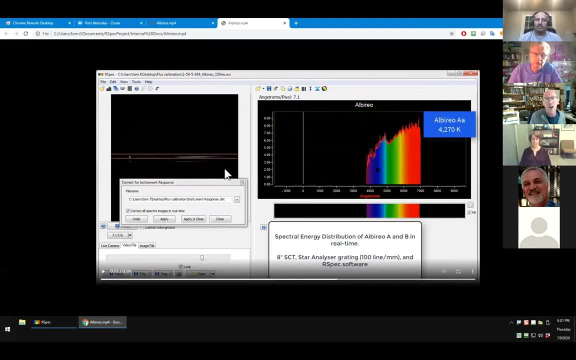 So now we're again. it's a secondary way of detecting star temperature. I hope that answers your question. If it doesn't, I'm happy to get into more detail. Absolutely, I think Justin had asked that question. There was another question from Jeff Kempner. 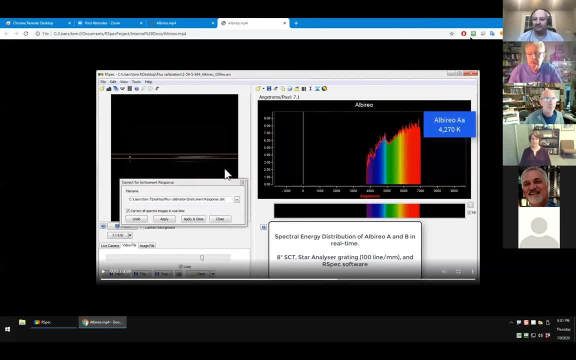 Does the atmosphere affect the spectral results? And I think you just alluded to that a bit. Yeah, that's right. If you capture this like any object especially, we see the sun. the sky gets red. The sun gets red as it gets closer to the horizon. That extinction happens in spectroscopy too. So if Albireo was just rising or just setting, this would have even more red here, And so the atmosphere does affect it, Not dramatically. It's not really a big hassle for most of what we do with the spectra. 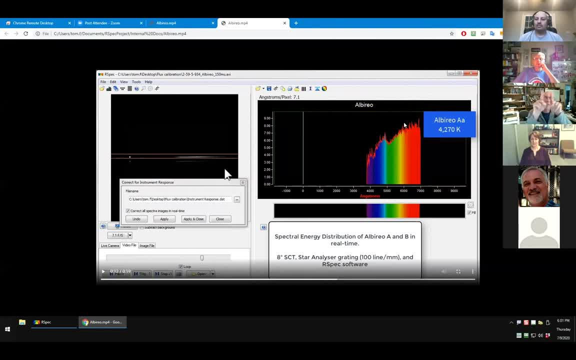 But it's important to, if we're doing comparisons, have them in the same part of the sky and, in general, be above, say, 40 degrees above the horizon, just to eliminate most of the reddening that occurs. That's a good and insightful question. 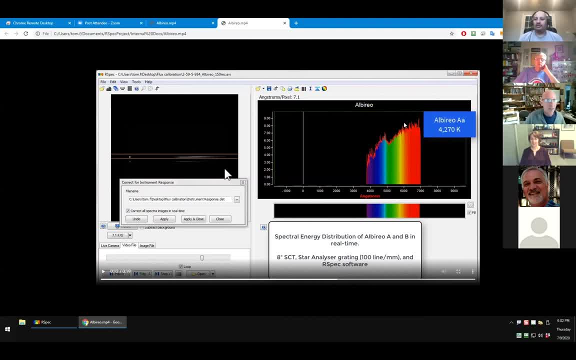 And not dealing with a plume of Saharan dust like we are here in the southeast United States, right? Oh yeah, there's that too. There's that too, You know? just a quick thing: The reason I've enjoyed doing spectroscopy is because your questions are good ones, but you can have great fun even discounting all of that. 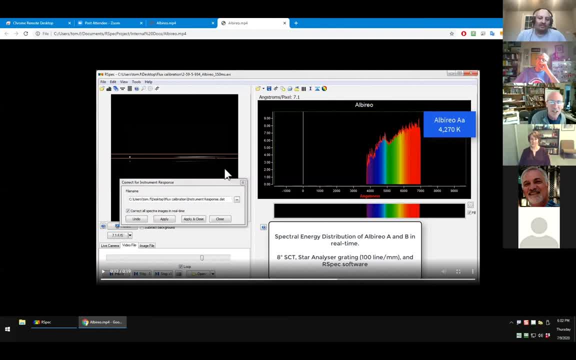 Because all you're really looking for- and you can see it here in this slide- is that little dip right there, Right, Which, if we spread this out, we'd see is right there. So go ahead. What else, Joe Perfect? 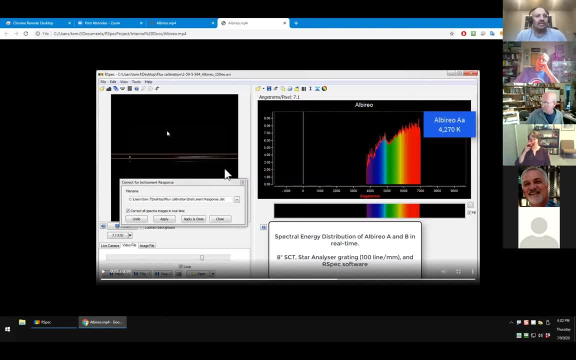 Justin also asked any spectral changes to Quasar, integrated over time detectable and plotted data using the RSpec software. Good question, I don't know. I meant to say before we started the Q&A that you'll stump me easily. I don't know the answer to that. 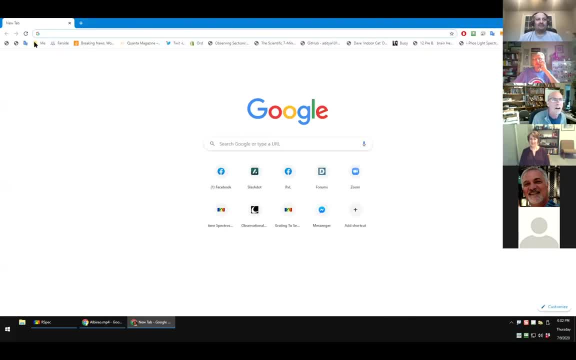 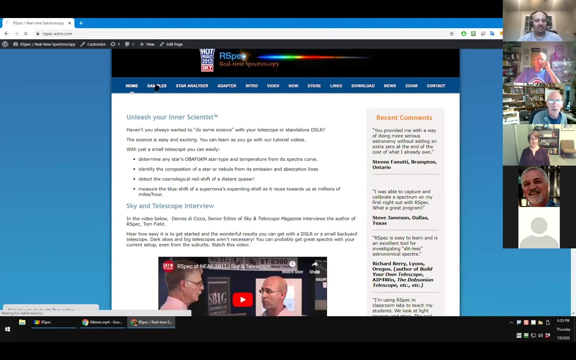 But over time there are things that you can. I hope I don't have anything revealing up here. I don't I've got the Far Side. By the way, he's publishing a Far Side character or fan. But what I wanted to show you was on the RSpec site under samples are a lot of the samples I just showed you here. 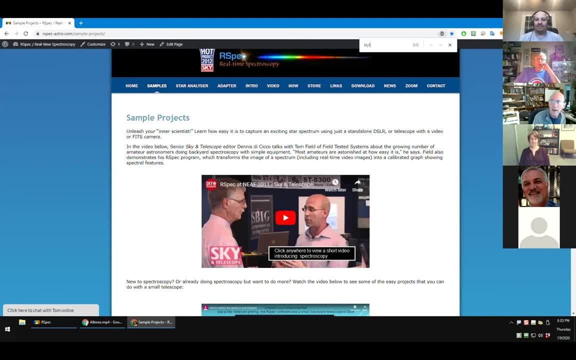 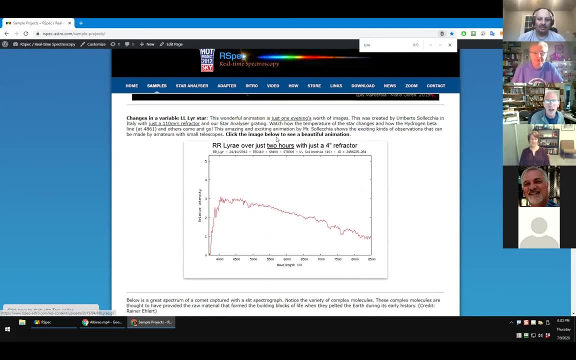 But what I wanted to show you, L-Y-R-E, L-Y-R-E. there it is. So here is our Lyra, over two hours. I'm going to play a little video. if I can find it, I'll click on the image and I guess I made it clear there. 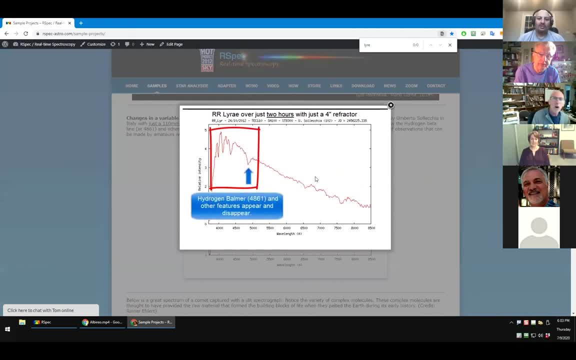 Watch this video over two hours, done with a four-inch refractor. Watch the change in the shape of that line. And not only did the hydrogen bomber features come into clear view here, but it gets much hotter right down here in the blue range. 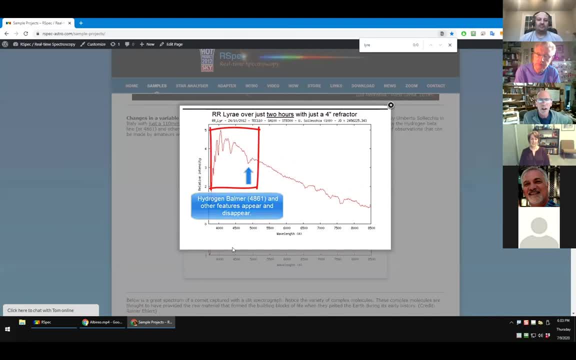 Two hours Now. this animation wasn't done in my software, But you can capture this kind of data. That's pretty cool. I mean I love this. What else, Absolutely? Justin did also ask what's the software language required to write this program. 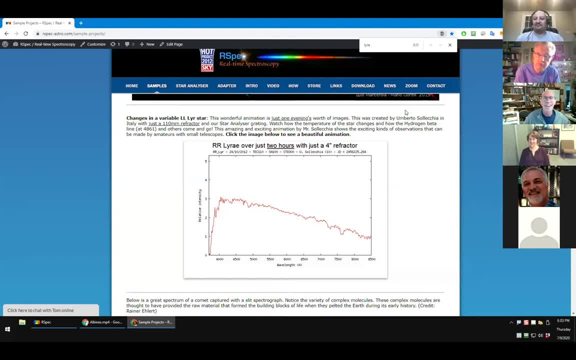 So more of the techie stuff with the software development. Well, you can write it in anything, I don't. well, I'll tell you, I was a little embarrassed, because it's not C-sharp or C++, It's Delphi. 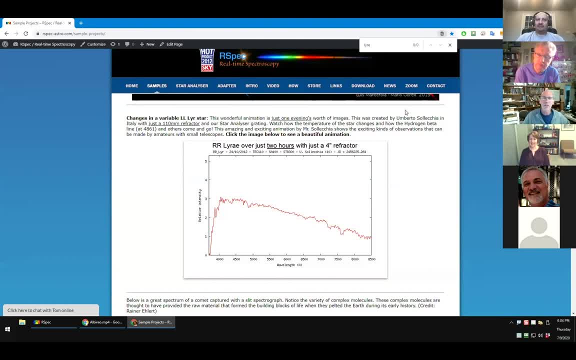 And if you're not familiar with Delphi that's because it's a little bit of a second-tier language. But it allowed me to port the software to the Mac. in a week or two We have a Mac version of the software for the classroom, for this thing, for the little classroom: gas tube spectrometer. 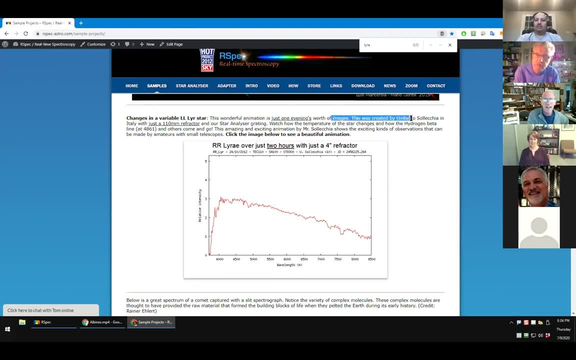 But there isn't a Mac version for astronomy. I'm not taking the time to do that, Sorry Mac users. There aren't enough of you to make it worth my time. We hear that often as Mac users. Yeah, But I'm thinking about it. 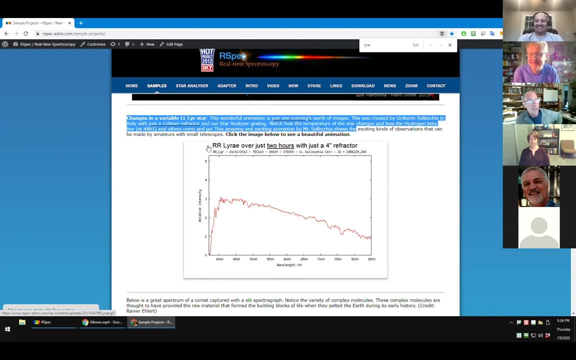 I really am. In fact, for those of you who can see the postage stamp view of me, that whiteboard in the background is a list of the things I'd have to add to the Mac version. The problem is I can't erase that stuff because it's been up there for about three years. 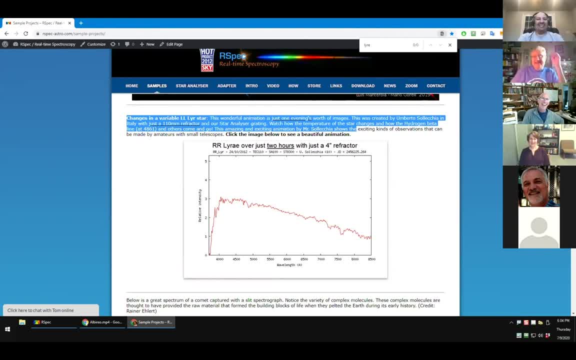 You know it's permanent. on that. It's permanent now, right? What else? Oh, while you're looking for something, let me interrupt you. This was the other prop I wanted. It's so stupid. I'm embarrassed, But I was talking about averted vision. 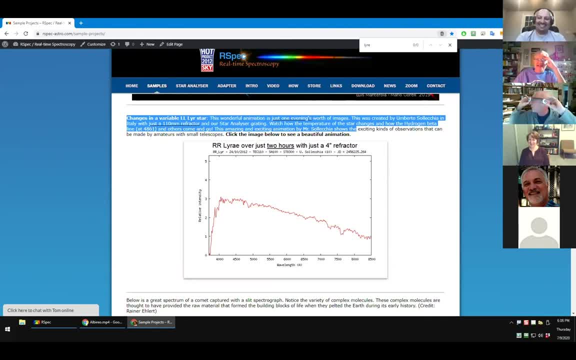 How's that for averted vision? You can't get better than that, can you? You know both sides. So there you go, Wonderful. Well, I'll go ahead and open up the microphone now to anybody who wants to ask any additional questions. 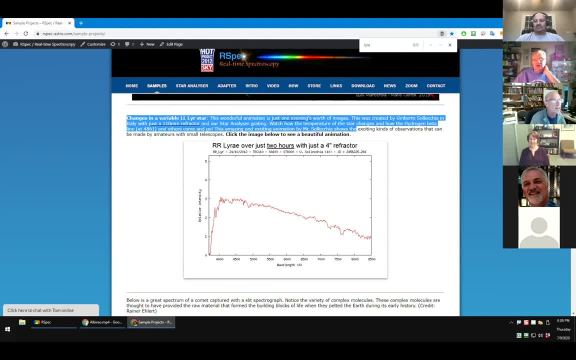 Great. Yes, Tom, I have a question. You mentioned- I don't know how to pronounce it- August Comte, who said we'll never know what stars are made out of. Yes, What kind of scientist was he? He was a French philosopher. 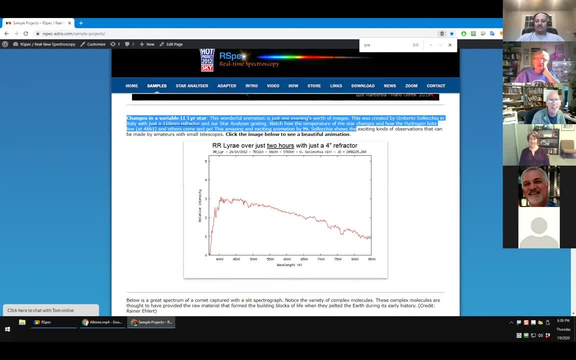 I don't know if they really had categories of scientists, because that was like in 1835.. It's a good question. Yeah, I don't. I don't know much more about him except that quote which is used to ridicule French on some occasions. 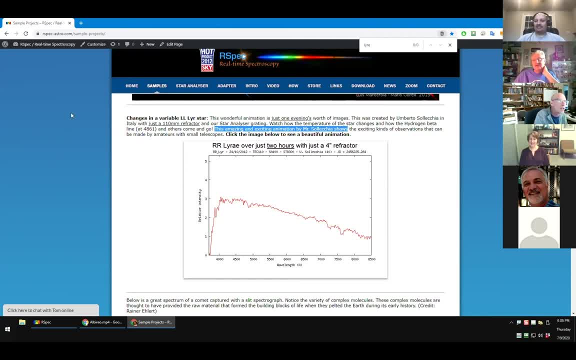 But, Bill, you know I was planning to really give you a hard time because I heard that you got thick skin and that you deserve it both, But unfortunately I didn't get there. But that's what they're saying behind your back before the meeting starts. 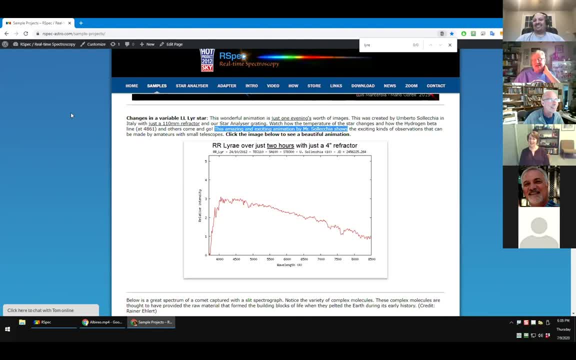 Is it true You're going to have to ask them, I guess? OK, Go ahead, Bring it out, I can handle it. I'm from Chicago. That's, that's the attitude I like. What other questions do we have? 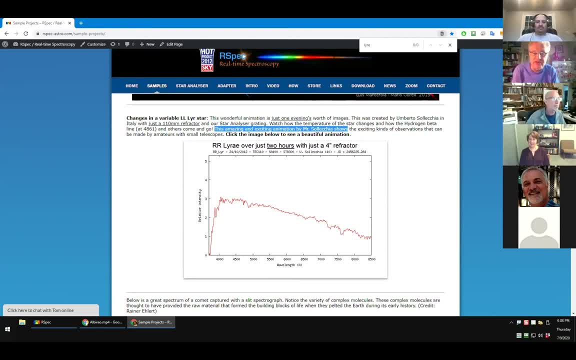 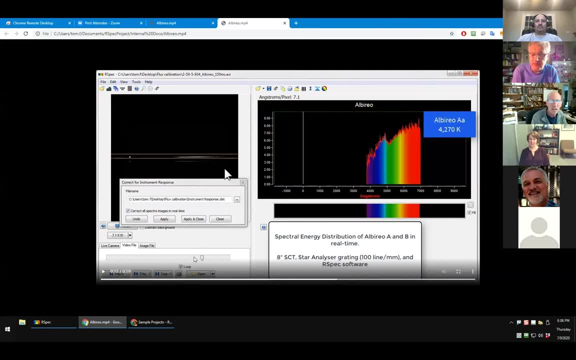 I do have another question. You showed us a spectrum of a star superimposed over the spectrum from the moon and there was a lot of hydrogen being shown on the moon- And I know there's been a lot of talk of that lately. but is that the hydrogen that that spectrum was showing? 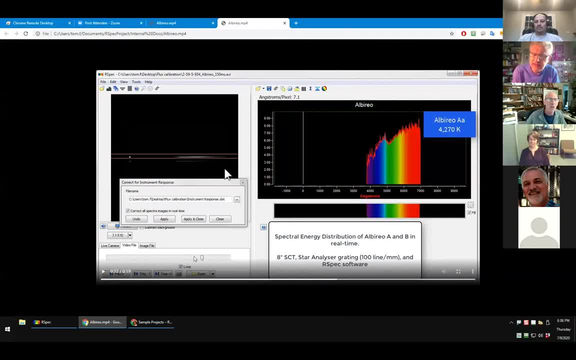 No, it wasn't. That's a really good question. The first time I've asked it or I've heard it, I don't know the answer. No, that's not hydrogen on the moon. I think that's probably the reflection of sunlight on the moon. 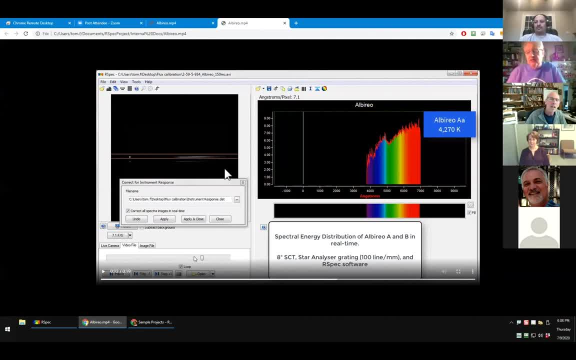 Most of the moon is basically inert. In fact, even it's a good question because it brings up that issue of reflected light. So the sun has a lot of hydrogen on it, And so that was the absorption line from the sun, I'm pretty sure. 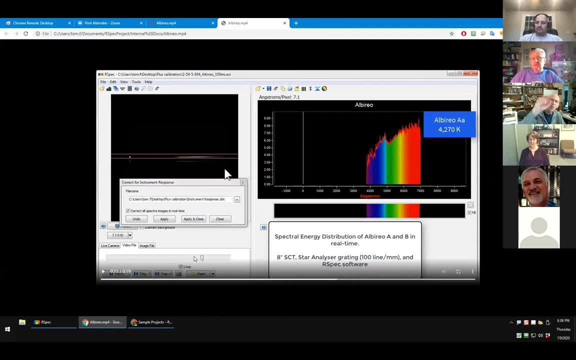 But that spectrum I showed of Neptune in order to really see those methane lines. what that guy did was he subtracted or divided out the spectrum of the sun, And so that was the absorption line from the sun to the sunlight star, so that the only light we were seeing was the light that was different than the sunlight that was hitting the planet, the contribution of the planet to the sun spectrum after it bounced off. 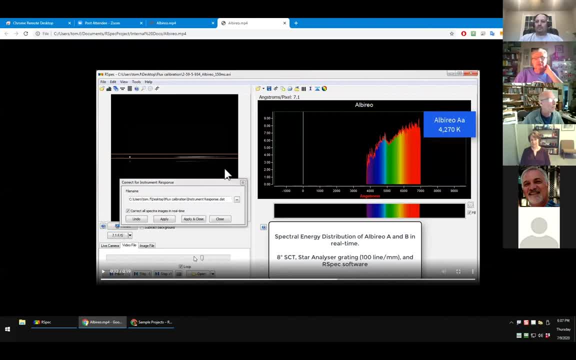 But that's relatively easy to do too. OK, thank you. Sure, Thank you, Great question. Bill Pellerin had asked what kind of new science can be done with the AAVSO spectral data. So that was kind of getting to where I was going to, to a question I was going to ask myself. 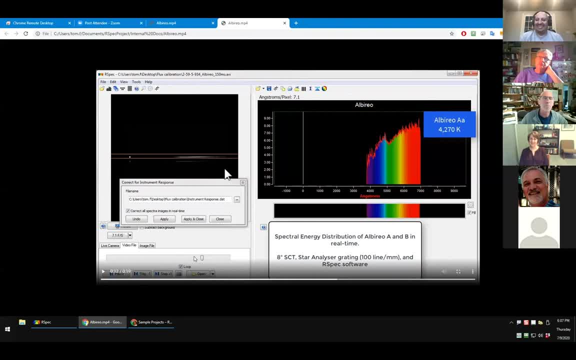 Yes, Stella and Arne. There you go. You know, I don't know, Because I'm not a photometrist. I haven't even been that familiar with the work they do, except that it's applauded in all areas of our field. 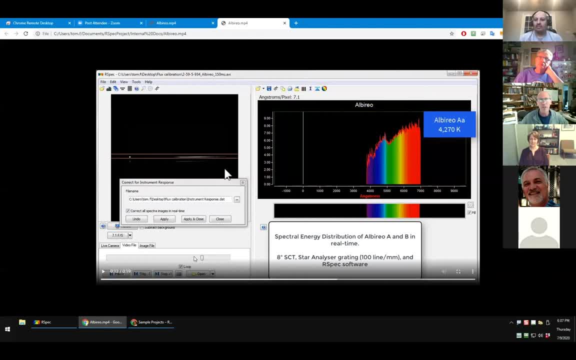 I think the sense is that this data becomes archival data for people to go back and look at when they're interested in historical changes that have occurred. As I mentioned, the pro-am world: Yeah, Yeah, Yeah, Yeah, Yeah, Yeah. 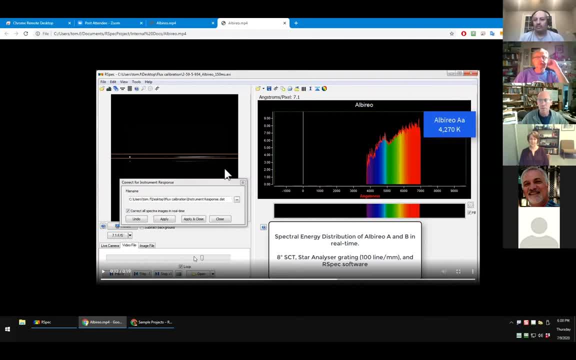 The pro-am world is unfortunately not as developed in spectroscopy. There is an American astronomer in Italy named Steve Shore who a few years ago solicited the help of some more advanced amateur spectroscopy participants, And he did the right thing. 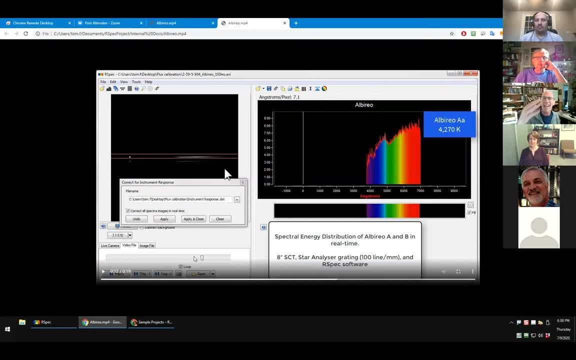 And that was he fed them. every week he would write a mini essay And he'd say: now, the spectra you gave me this week it was on a fast-changing star, It was on a BE star, Which is a type B star that has an emission line. 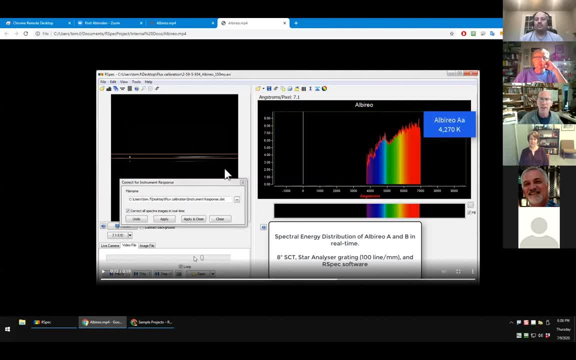 That's what the E stands for, because it's thought that it has a dust ring around it that varies in angle to us. But so he wrote these essays and he explained to them what they were seeing. So they got all excited. But there has not been as much of that kind of thing going on. 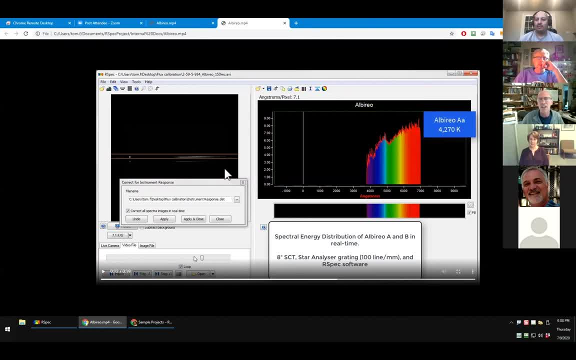 And I know Arnie originally, and now Stella in charge of the AVSO, want to reach out to the scientific community and see more of that kind of thing going on. There's also, And I think as you all know, there is in Europe a BE star database that the French maintain. 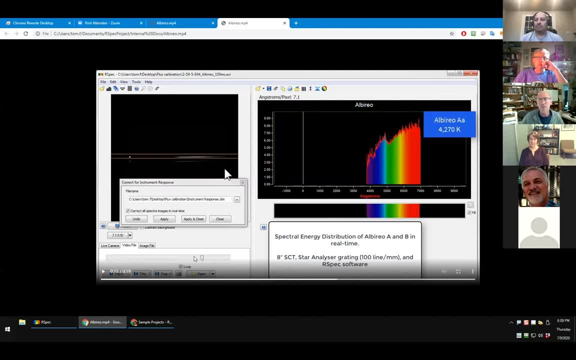 that a variety of members and contributors to that database have been named on a variety of papers that have been published, including the one that I popped up on the screen for a moment from the AAS a few years ago. So there are opportunities, but it's important for me because I actually sell something. 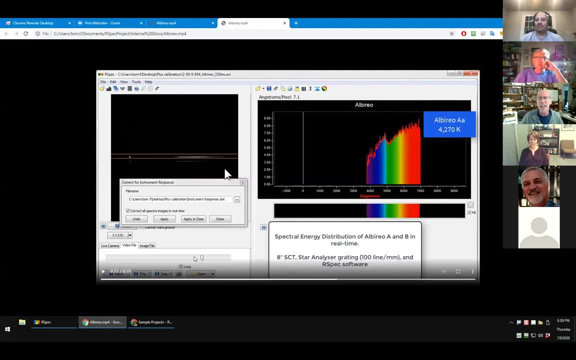 not to overpromise that. you'll be solicited and you'll get emails from scientists every day asking you for new data. Well, there are a number of opportunities, but I actually think not everyone is a scientist. There are other groups of people who are not scientists. 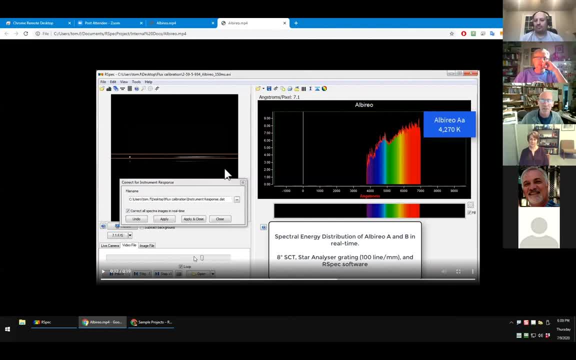 One of the things that can be done also, I believe, is- and I'm trying to think of the name of the guy- he went from a camera company, went up to SBIG for a while and now he's on a sailboat. 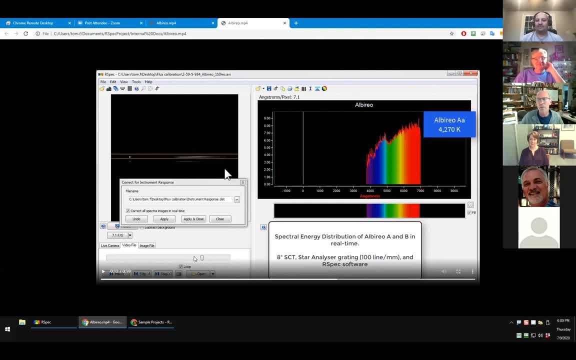 But he is a supernova hunter and you'd know his name if I could remember it. But apparently there's a ton of supernovas out there that never supernovae, that are never identified as to their type. They're sort of a backlog. 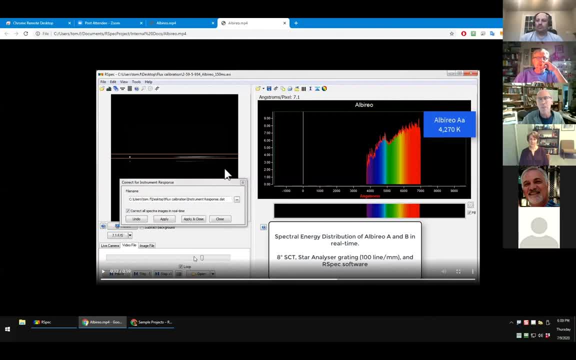 Well, the good news is that we've got the time to do it and we can pick some of those off, and if they have that deep dip, we know that they're a type 1a, for example. The bad news is- and this is a question that hasn't been asked, will be, and I'll provide it for you- and that is that you know how deep can I go with a star analyzer? 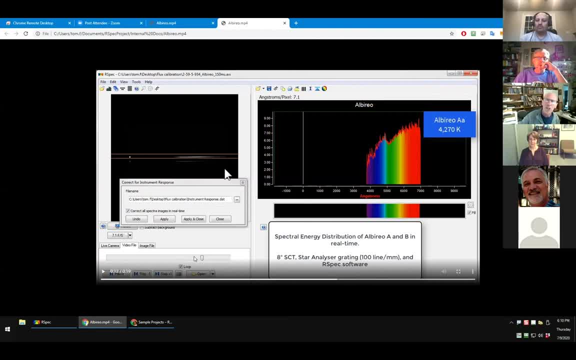 This is an important question because normally, when we're imaging normal stars without a grating, the star's photons, all of those photons that come through our telescope and through the atmosphere and hit our sensor, are on a handful of pixels right. 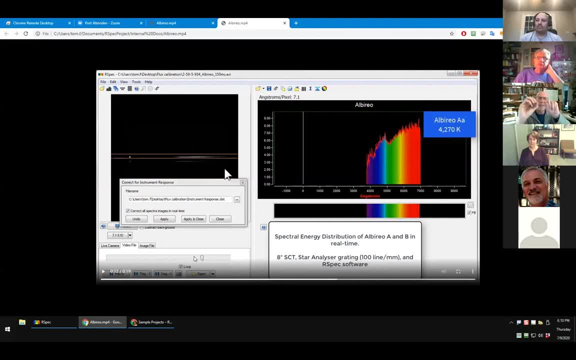 Well, now take that same total number of photons and spread them out way across the sensor. Now they're spread out across hundreds of pixels. You lose about five or six magnitudes when you put a grating in the light path. So if you can normally image down to magnitude 15, you'll be able to capture stars down to, say, 10 or 9.. 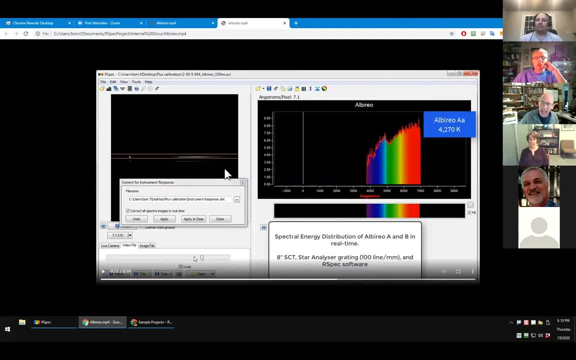 There's tons of interesting stars to look at. You can stack these images, You can do darks. Eventually, though, if you go for a few years and that becomes something you want to do, you want to get to dimmer and dimmer objects. 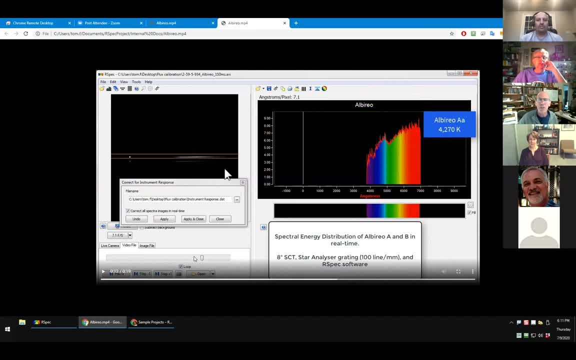 then you step up to a slit device which can go much deeper for a variety of technical reasons. So what else? Go ahead, and if you have a question, go ahead and unmute yourself and ask away. Joe, I have a question. 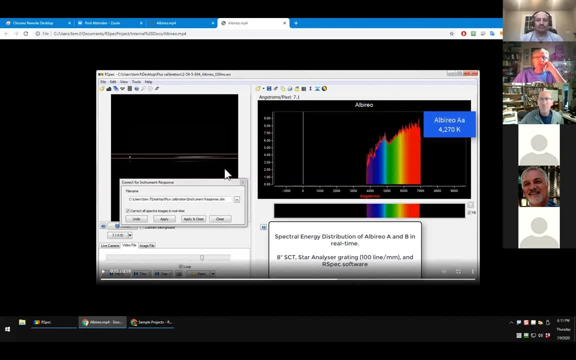 Sure, Hi Chris, How are you? Yeah, I'm great. Hey, Really good talk, Tom, Appreciate it. I'm a real novice, so this is going to dial us back a long way. Not a problem If I have a nebula that I'm trying to see and I understand the emission bands from that nebula. 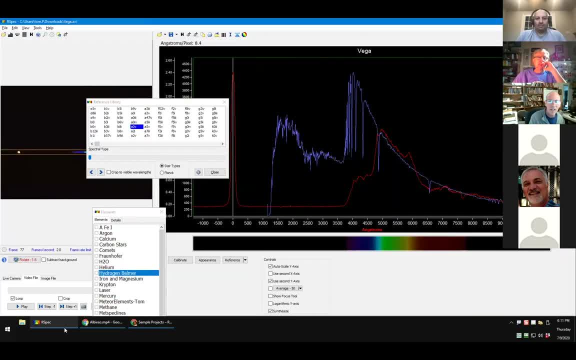 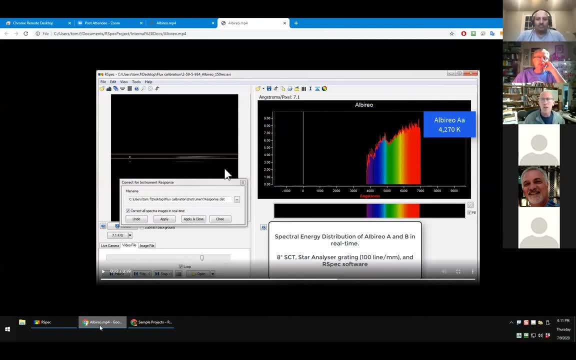 would that guide me to a filter that would help me see that nebula? Yeah, it would I mean, but there's people who know far more than what knuckle draggers like me might be able to discern. But you could confirm what other people say. 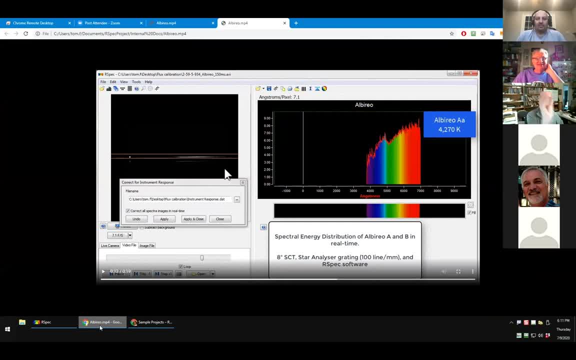 Absolutely. If you have helium or hydrogen line, then you know that's where your data is, And so that's a great question. So you're no longer a novice. In fact, I have the luxury that I can say things like this. 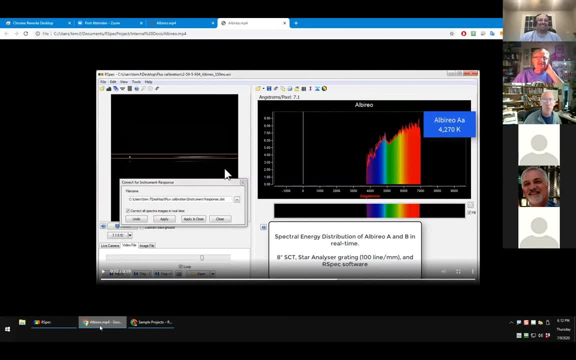 What's with the name novice? That name, novice for this group, is sort of not a popular name. You need to come up with a synonym for that. that's better. You're enthusiasts right. There we go. Well, I'm an enthusiast sort of you know. 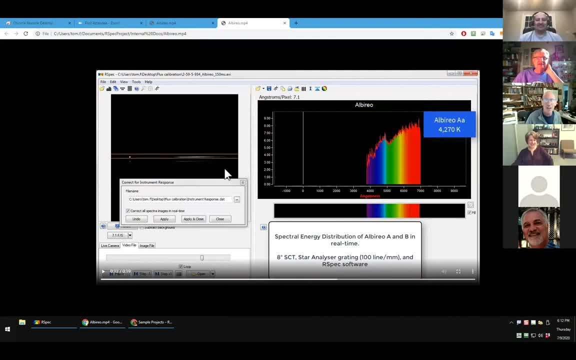 Yeah, Anyway, that's my contribution, But just to again, just that would. I'm just trying to see a nebula, Right. I've got basic, pretty basic goals, Yes, And I'm looking for some technique or piece of equipment that will help me do it in and around my home. 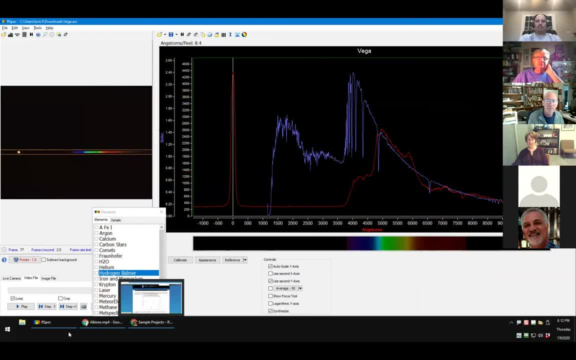 Now I've got a lot of light pollution, so that's probably part of my problem, But that I just want to understand the concepts and it sounds like I've got somewhat of a grasp on it. Absolutely, It's an ingenious way of looking at it. 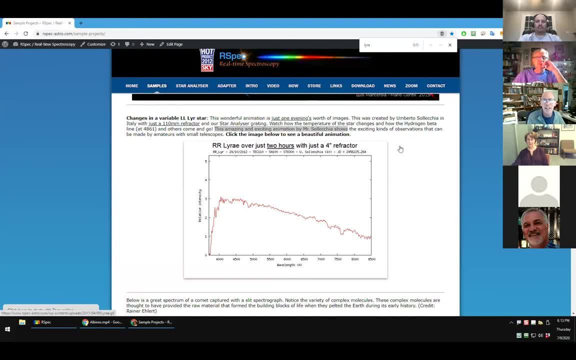 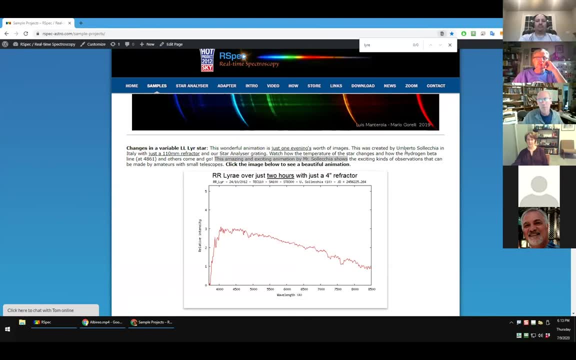 And it's why newcomers often come up with ideas that people who are more familiar with the field don't, Because not a lot of people have thought about doing it that way. doing it that way, I would say that the cost and the learning curve- and, you know, not only learning about spectroscopy- 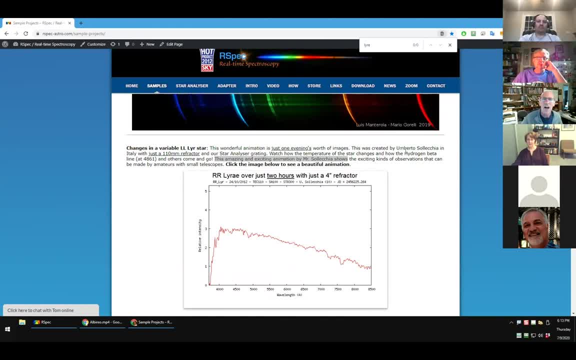 but you know, perfecting your imaging of dim objects, It's probably not the best time to spend your best way to spend your time right now. I'd talk to some people and ask them: you know what do I need to observe this object. 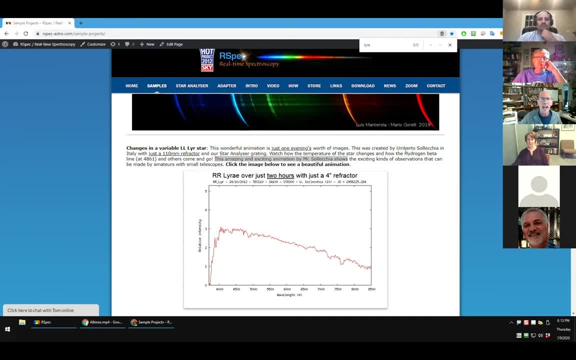 And, as you said, light pollution filters are very popular And, you know, different type of nebulae require different types of filters, And that's something a lot of the members here in the club may be able to help you out with. 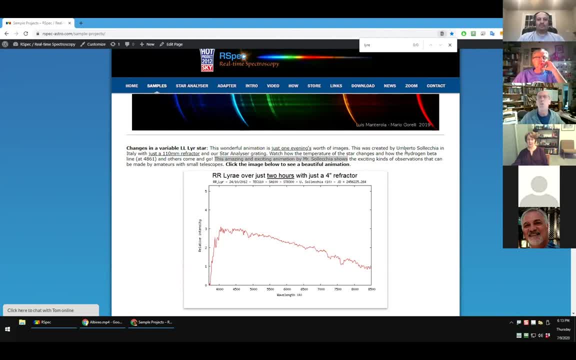 But theoretically and practically that is doable. It's a great question. You understand what it is that we see when we see an emission spectra And for those of you who don't know, it's a great question For those of you who are wondering about that question. just very briefly here, I was going to show it. 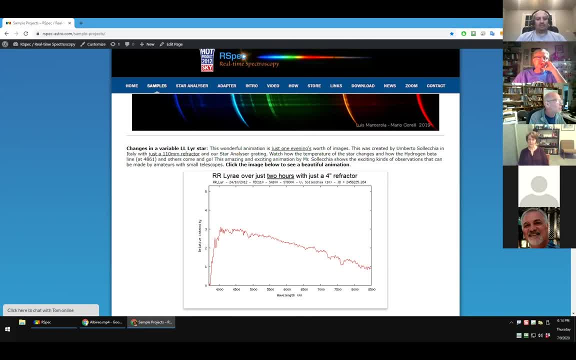 But instead I for some reason started clicking on another screen, which isn't exactly what I wanted to share with the group. I can't bring it up. I was going to show the nebula image from my slideshow, But let's skip that for now. 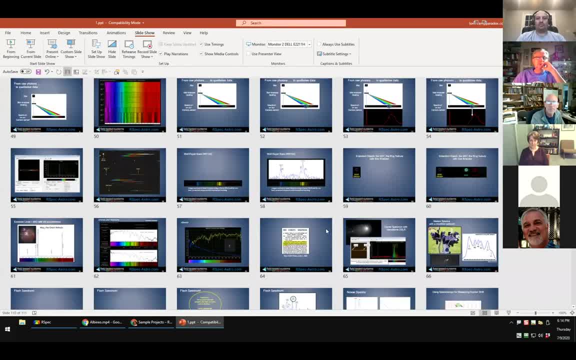 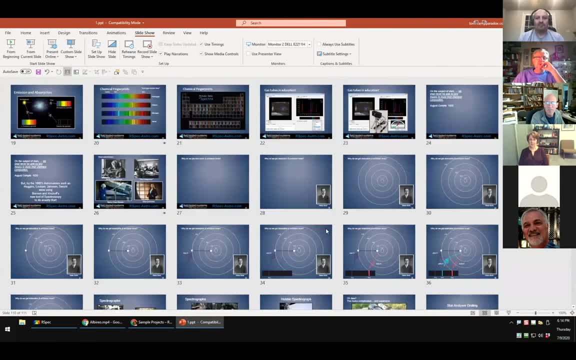 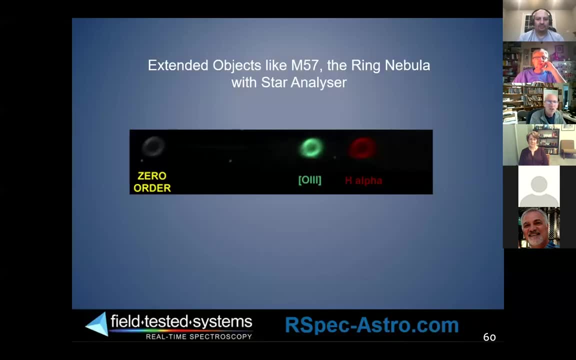 What else? Again, if you have questions, go ahead and unmute yourself and ask away. Good Tom, I apologize, I had a little bit of a problem. I think I interrupted you. No, no problem, I just wanted to show this slide. 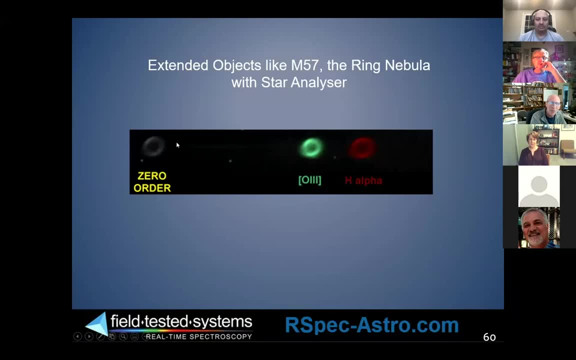 So what he was just asking. he said: when I try and image this object, let's pretend these aren't visible. They aren't visible. I don't get it because it's too dim, But if I could just select and look at only the colors that were here, that were in it. 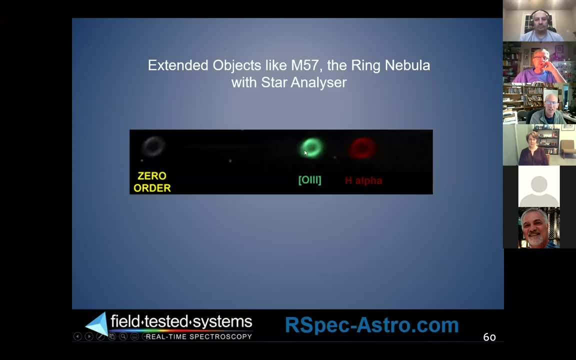 I'd get brighter images, There'd be less noise from the streetlights And in this case if you had a filter that just you know it's not going to be visible, but if you just allowed ionized oxygen, then you wouldn't get any of the sky background. 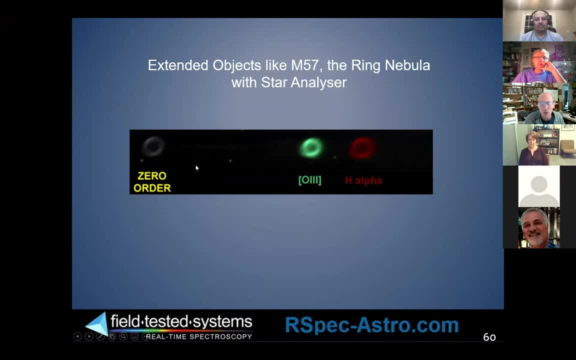 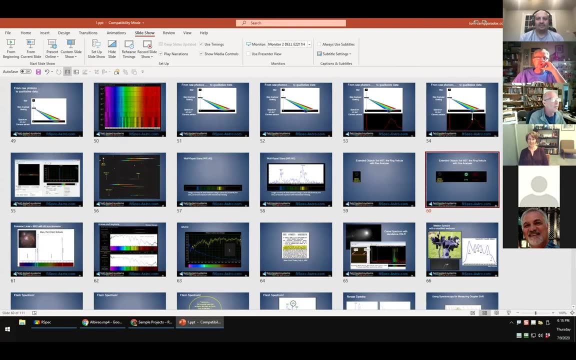 that is causing this image to be dim. It's not a great explanation. It's the first time I've tried it. Anyway, what else? So, Deborah, how'd I do? Come on Great. Thank you so much, Tom. 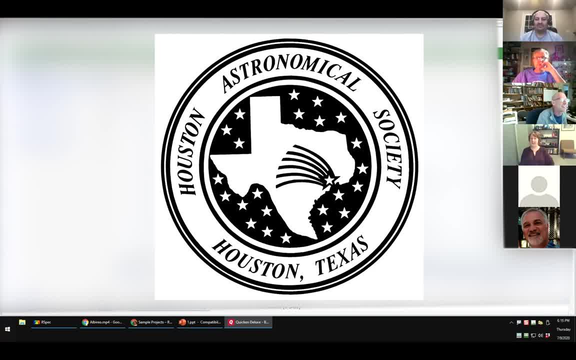 It was actually a topic. I was thinking of new topics as one that had not. it wasn't on my radar, So I really appreciate your bringing it up. It's like the fairy godmother of topics came across just as I was planning the second half of the year. 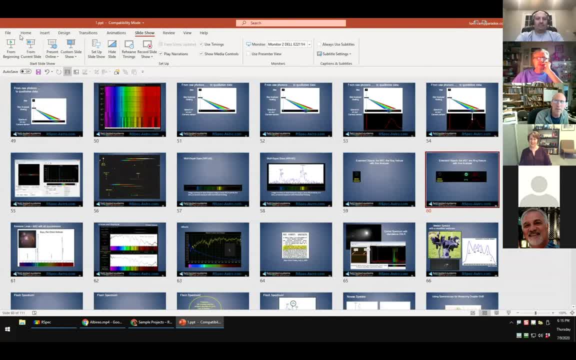 Yeah, So thank you so much. My pleasure. I'm happy to meet you guys And if there's anything I can ever do to help any of you, you know how to reach me And carry on and have a great evening. I'm going to check out and you all can hang out if you want. 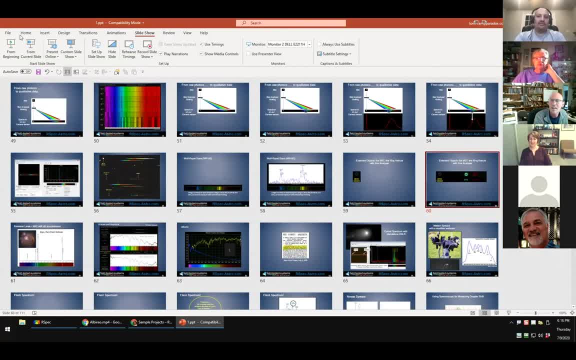 Appreciate it, Tom. Thank you very much. Before you go, I was going to ask you: do you have anything coming up in Sky & Telescope we should keep an eye out for. No, I don't. Okay, I'm actually working with a professor in Montreal who's going to describe some of his students doing spectroscopy as well as doing some photometry, and we're going to see if we can get that published. 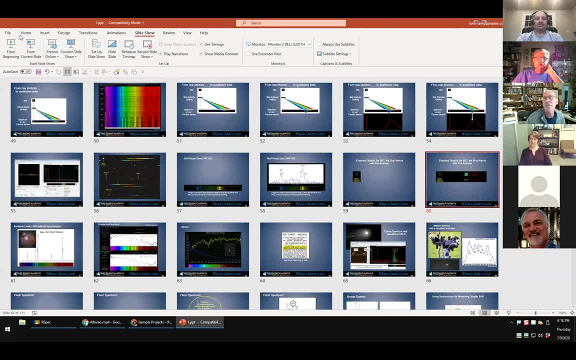 My goal is to popularize spectroscopy and I have a side benefit that I sell more product. But really the main thing is that amateurs, like all of us here in this meeting, mostly five, 10 years ago didn't know this kind of thing was possible and even today many don't. 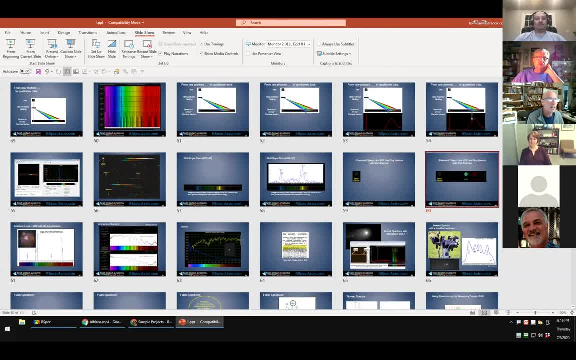 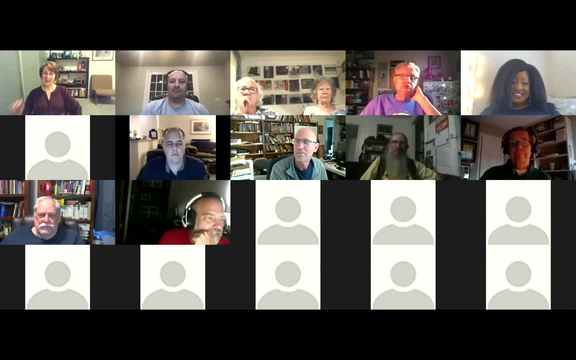 So that's what we've got coming. Thanks for the question And again, let me know. if there's anything I can do, Appreciate it. Thank you, Tom. Sure Bye, Have a wonderful evening You too. And for everybody else, remember our general meeting is tomorrow night, so please register for that when you get a chance, and we'll see you online tomorrow at 7..